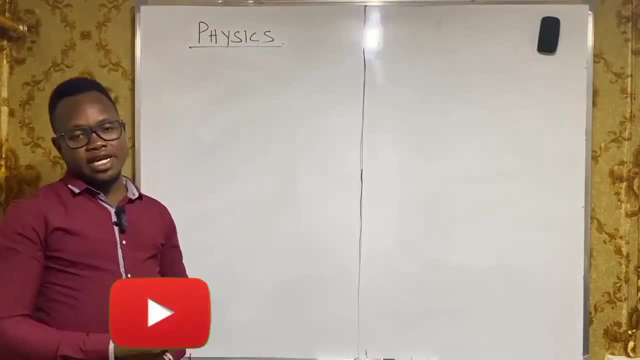 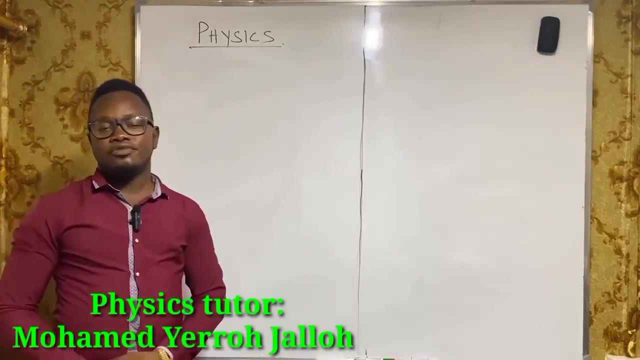 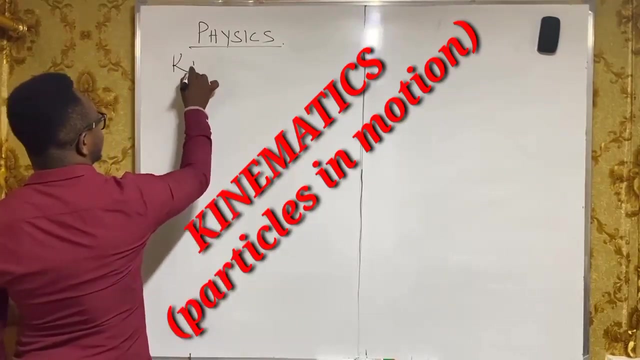 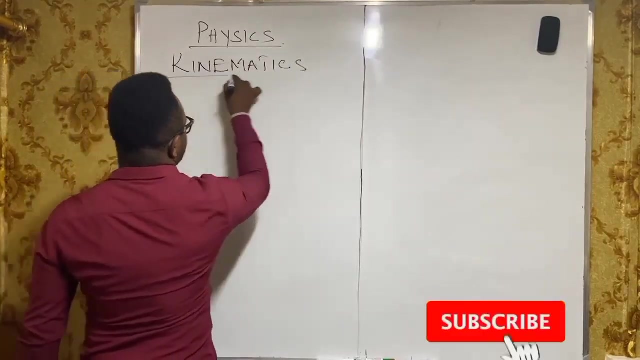 Good day, viewers, and welcome to your best learning hub for the sciences, JALO Science Academy. I am Mohamed Yerojalo and in this tutorial, I'll be taking you through your physics and we are going to look at kinematics, That is, particles in motion. 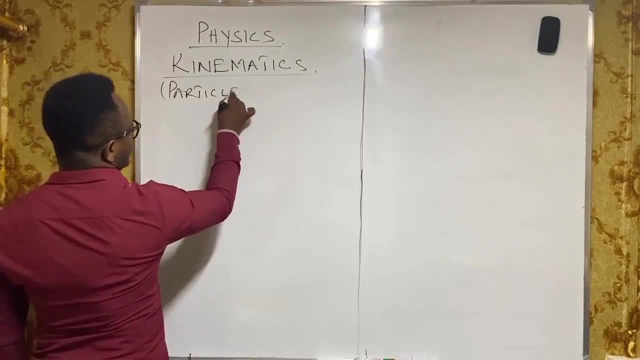 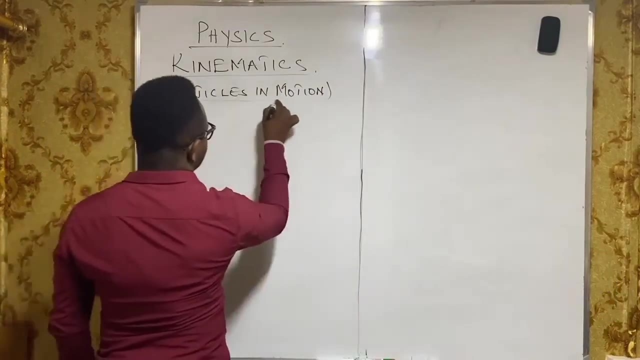 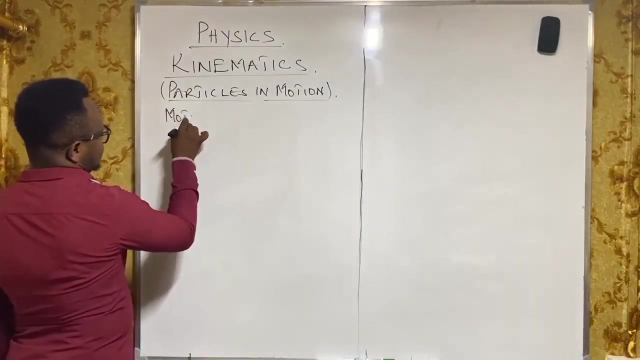 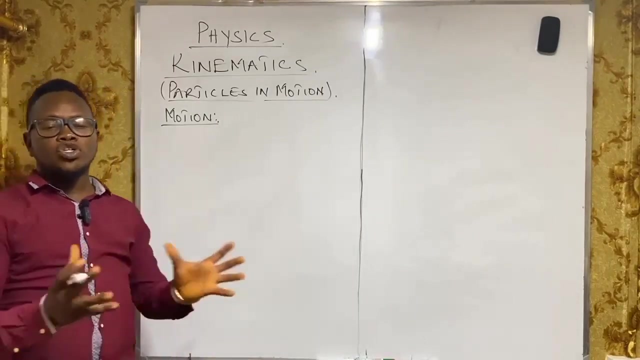 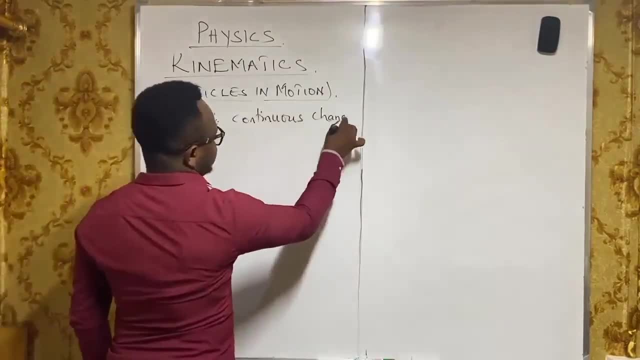 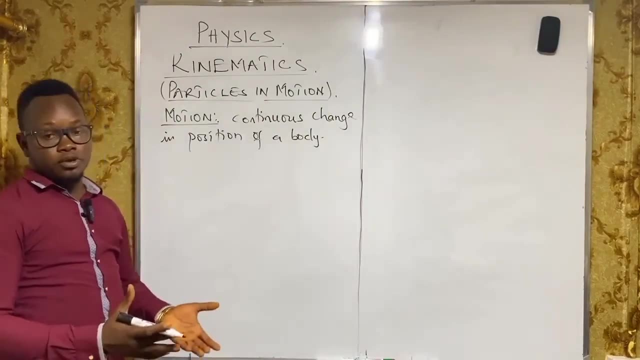 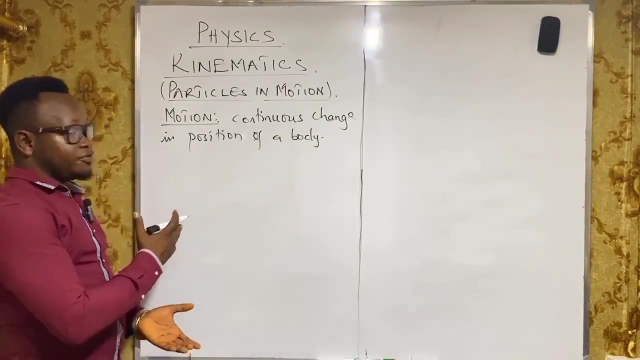 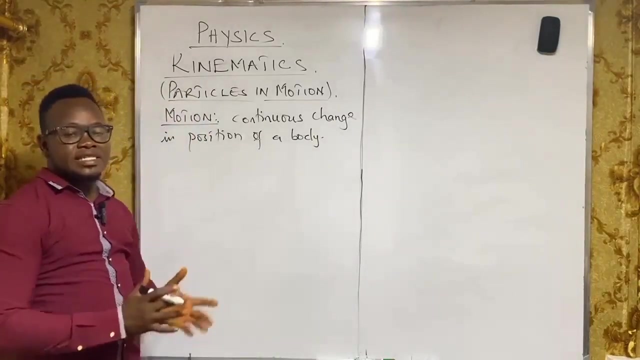 to a reference point. This continues. change which takes place in the position of a body relative to a reference point is most times measured by an observer. okay, Reference to a frame of reference. Now motion can also be looked at as any physical change in position of an object. Meaning if: 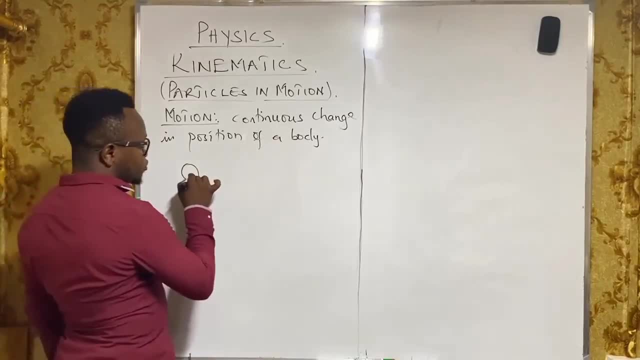 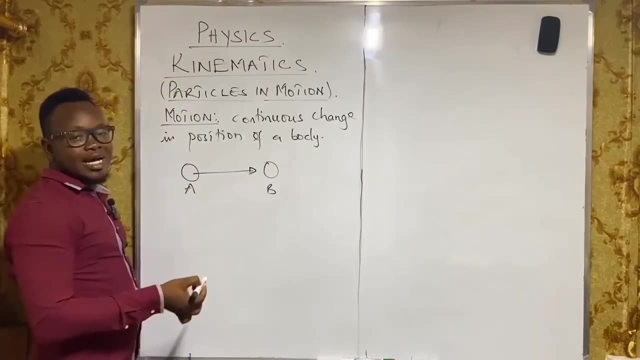 if an object is here and then it moves from this point to another point- let's say, this is point A and it moves to this point, point B- then we say motion has taken place because there has been a change in physical position. 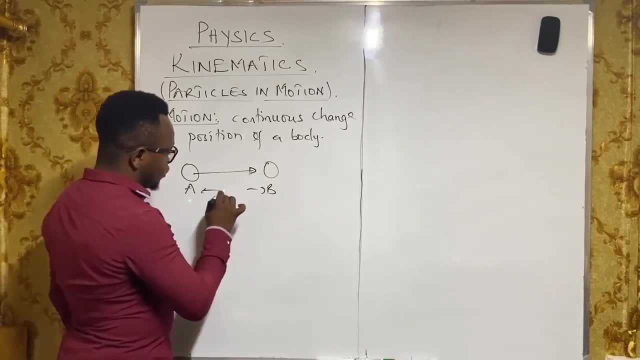 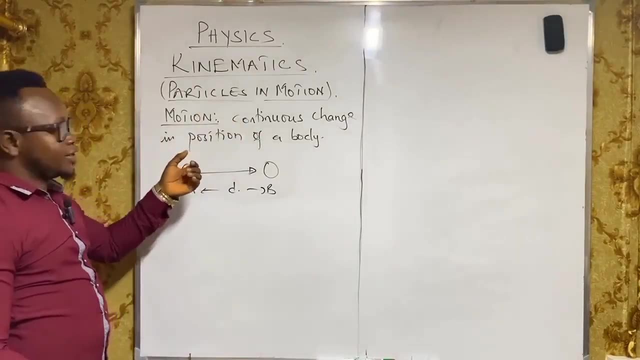 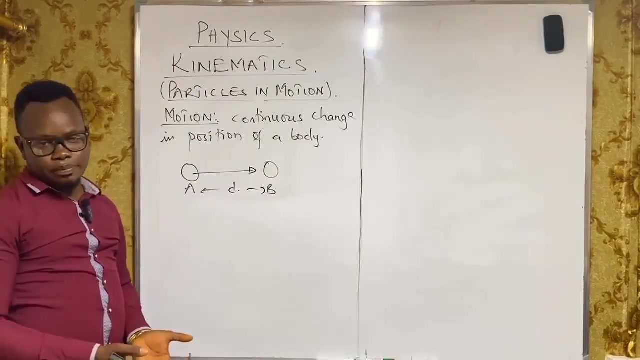 It has moved from point A to point B, which are separated by a distance. So we say this is motion, Having looked at a motion here. so what then, can we say is kinematics? Kinematics simply means the study of the motion of a particle. okay, 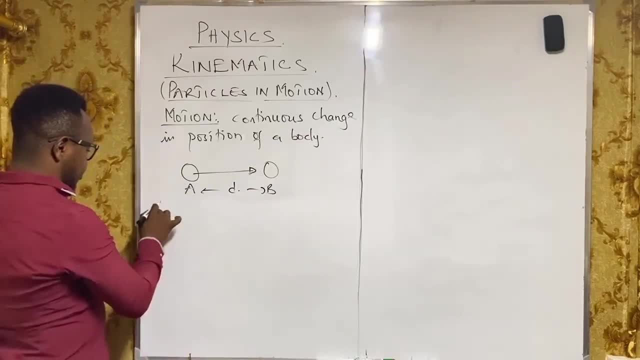 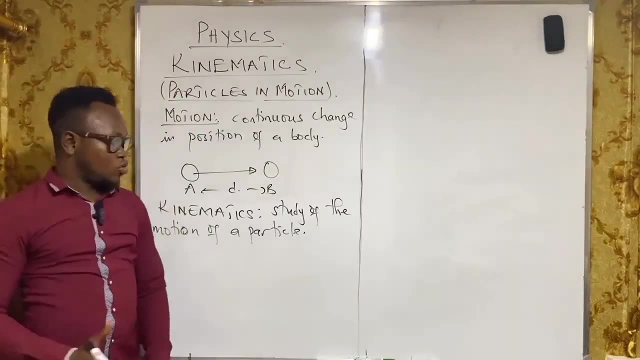 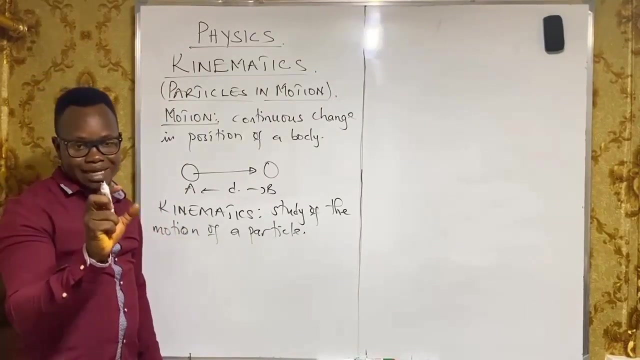 The study of the motion of a particle is what we refer to as kinematics, So the study of the motion of a particle. And a particle is a body whose dimensions are negligible with the exception of the mass. All the other dimensions are negligible except the mass. 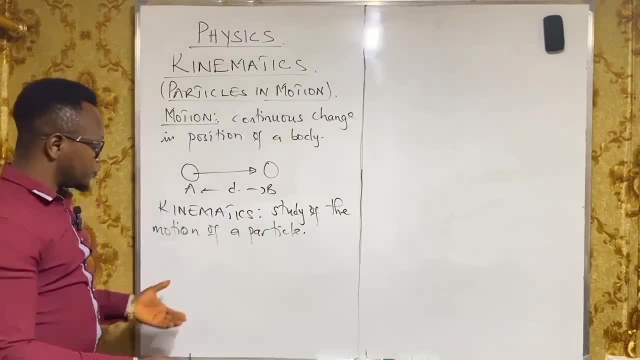 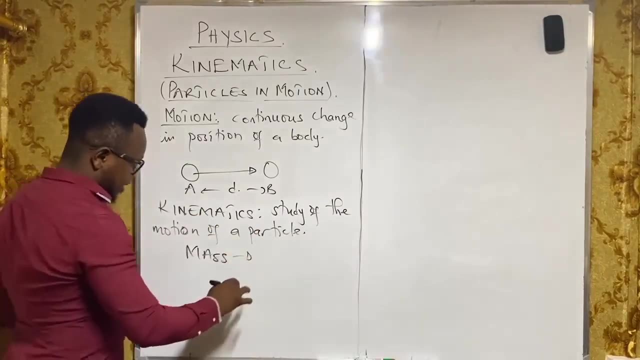 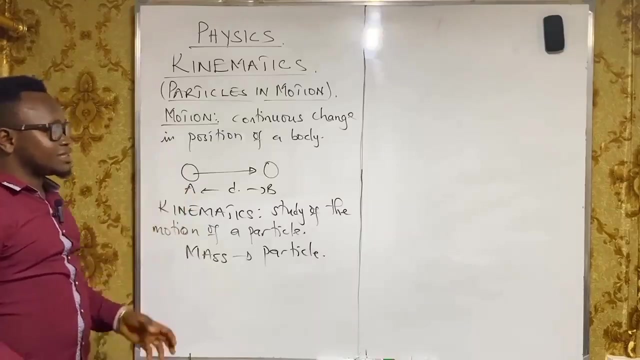 That is what we refer to as a particle. So if you have A particular body whose dimensions are negligible, with the exception of the mass, then that is referred to as a particle. okay, So we can now look at the types of motions. 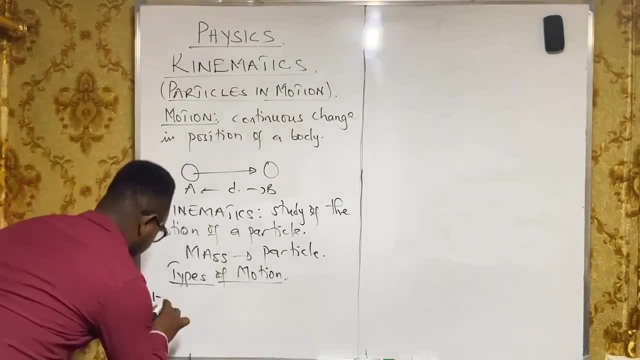 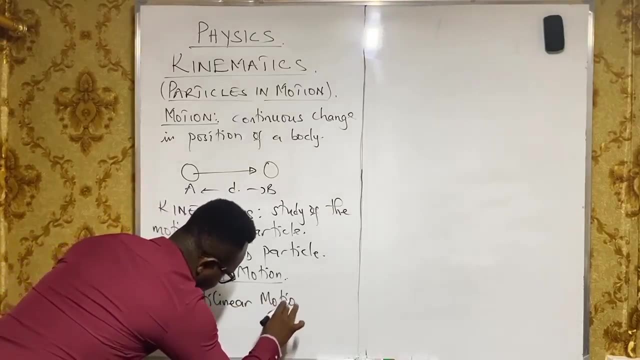 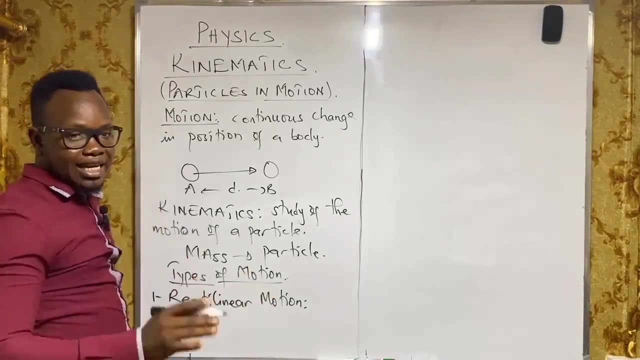 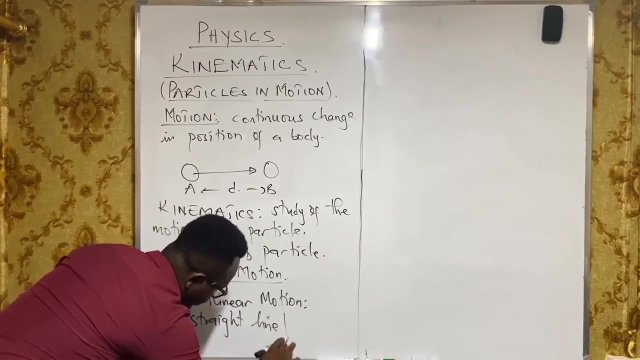 So one we can look at is: So one we can look at is Rectilinear motion. So a rectilinear motion is a motion that takes place in a straight line or a straight path. So if a motion takes place in a straight line or a straight path, 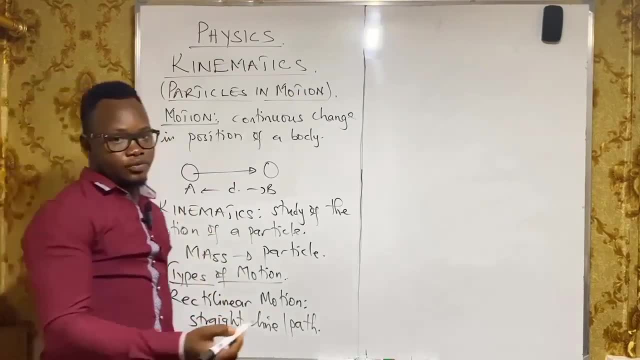 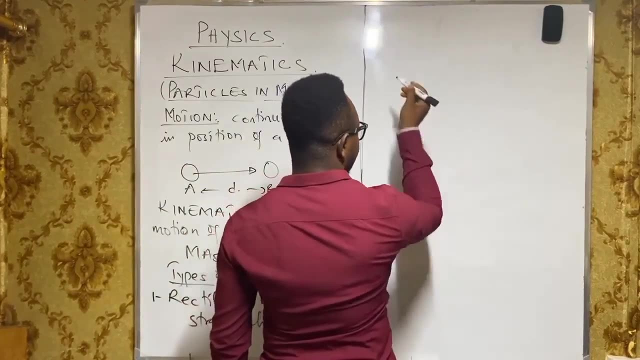 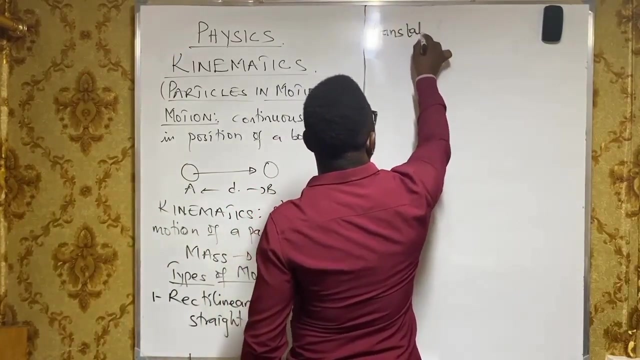 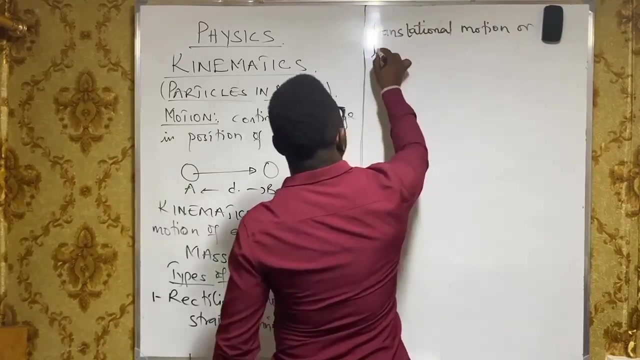 then that motion is referred to as a particle, Okay, Rectilinear motion. We can refer to them as motion in a straight line or in a straight path, Or we can also refer to it as a translational motion, Or we call it a linear motion. 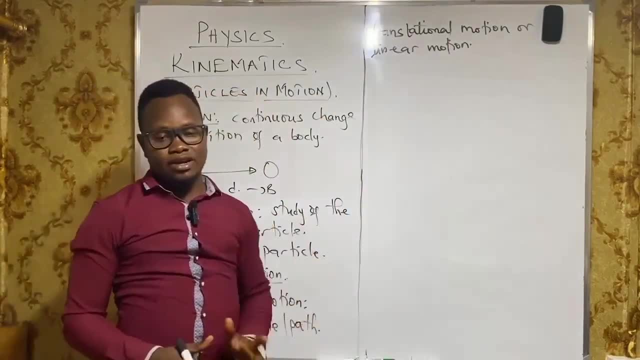 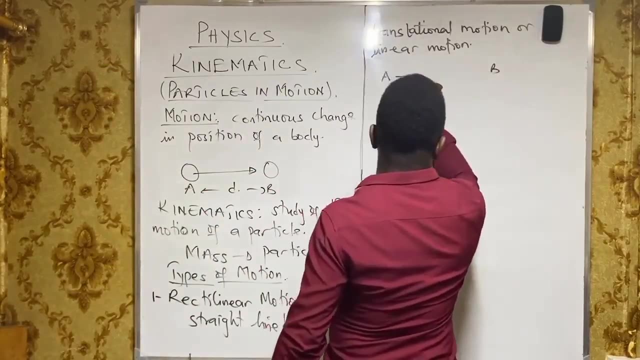 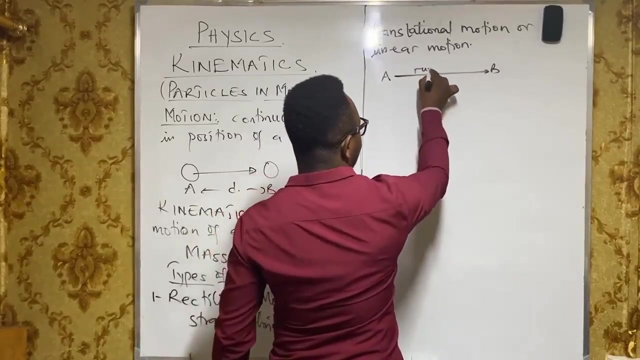 So we say it is either translational motion or we call it a linear motion motion. okay, for example, let's say you have a point here, point a and point b- there is a straight path existing. if a boy runs along this path running a race, okay, you run a race in a straight path. 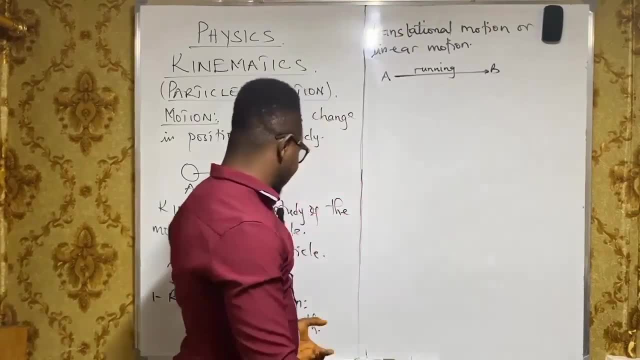 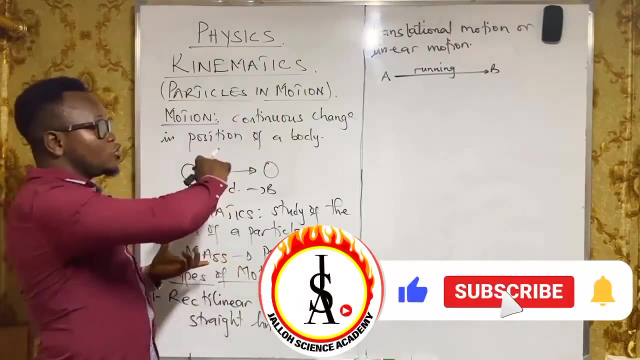 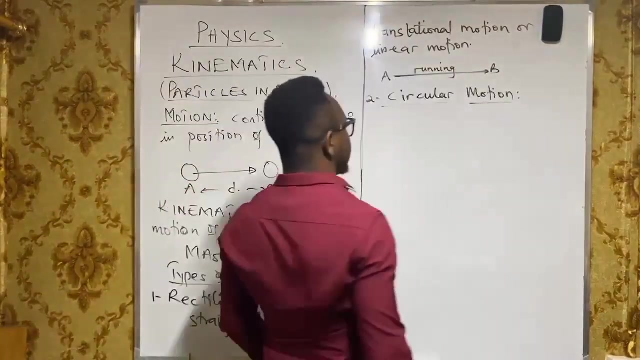 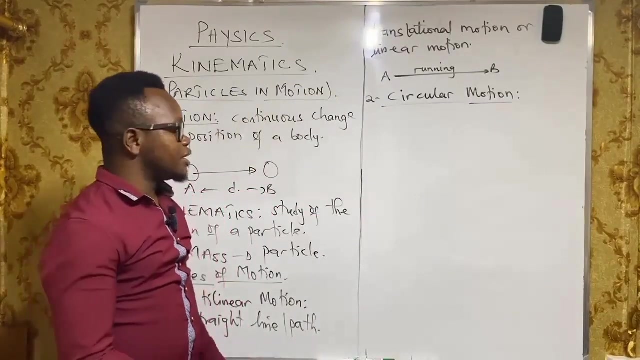 then that motion is referred to as a rectilinear motion, we call it a translational or a linear motion, so it's a motion of an object along a straight path or along a straight line. second circular motion: this is a motion of a body that's traveling in a circle. okay, for example, 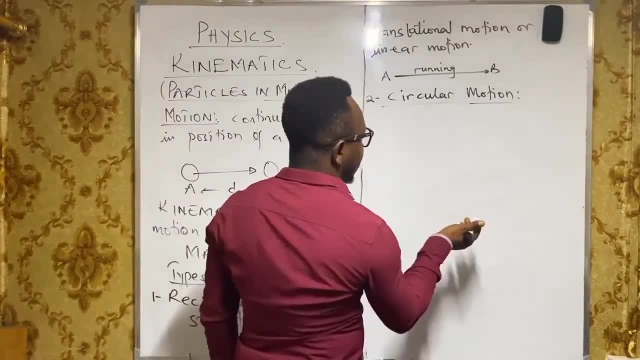 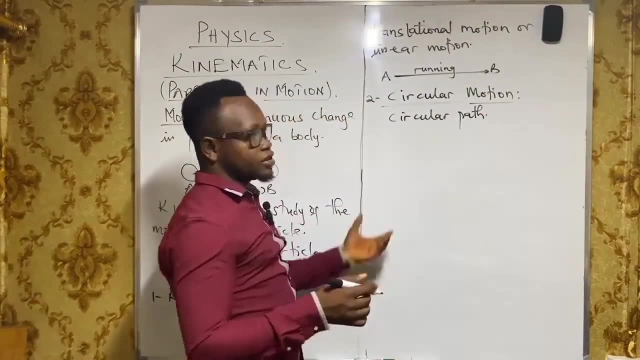 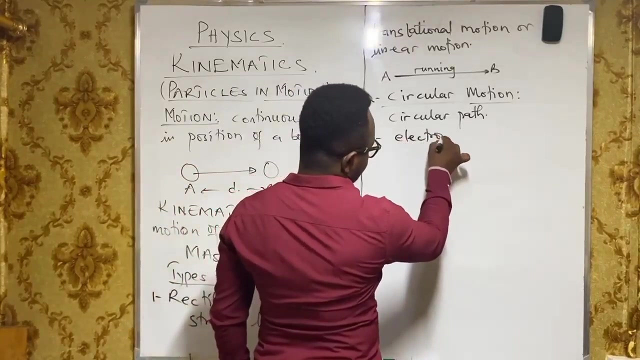 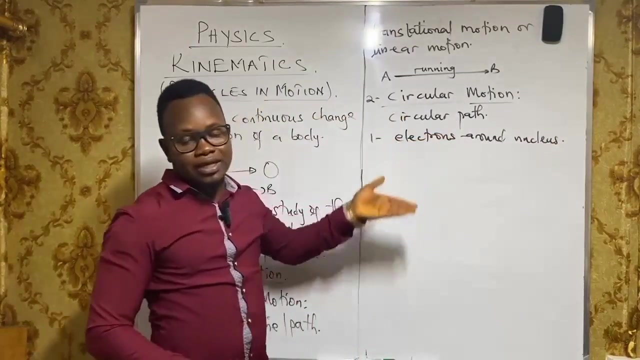 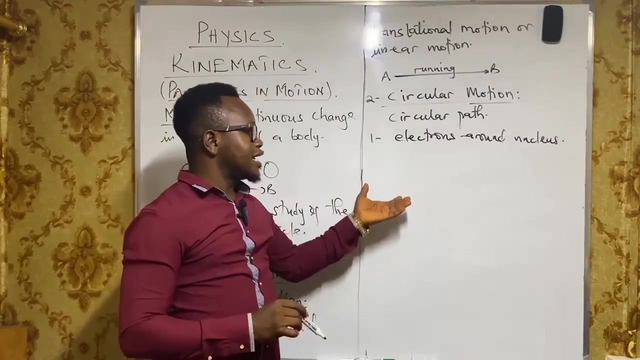 if a motorist is negotiating a curve, so here the motion of a body in a circular path. so this is motion around a circular path, one we can look at the electrons around the nucleus. okay, the electrons moving around the nucleus is an example of a circular motion. or you have satellites that are orbiting the planet, going around the planet. that is a 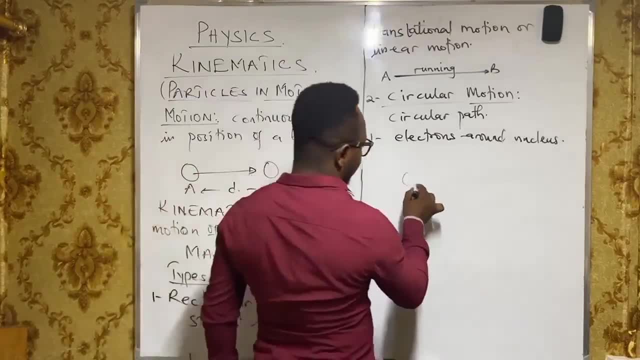 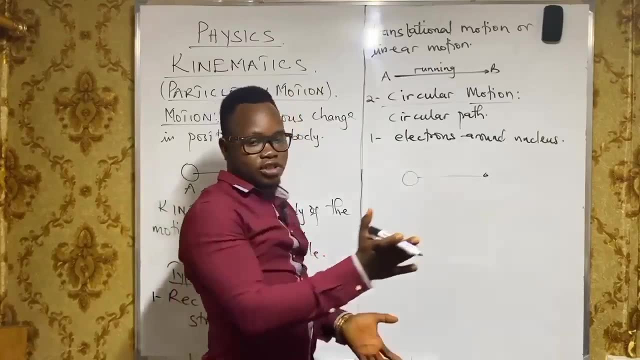 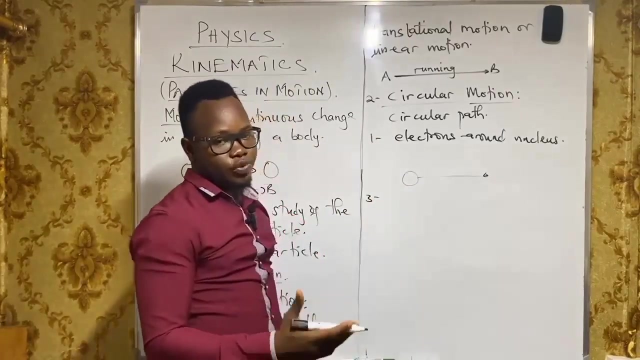 circular motion. or you tie a stone to a string and you wield it around, so it's moving in a circle, or you have a motorist negotiating a curve, or you have a motorist negotiating a curve. those are all examples of circular motion. and the third type of motion we can look at is rotational motion, or we call it spin motion. 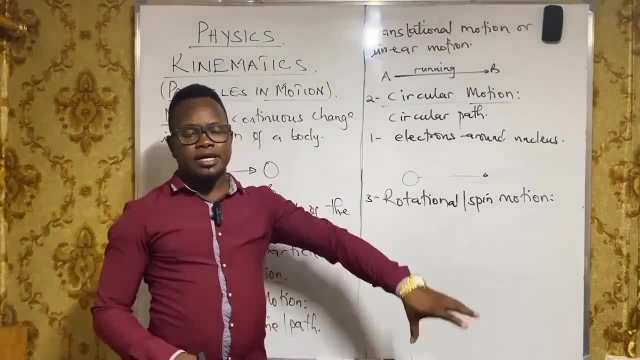 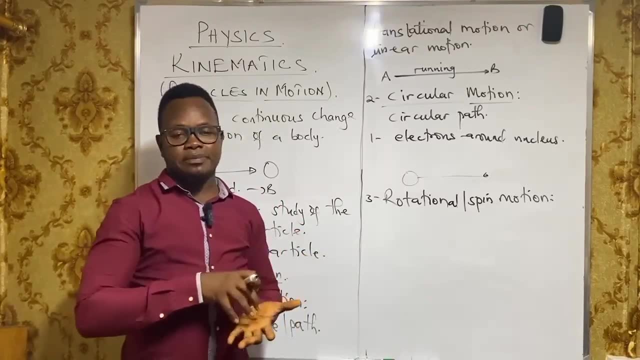 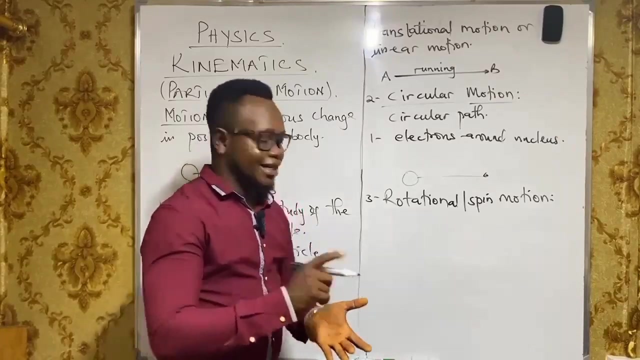 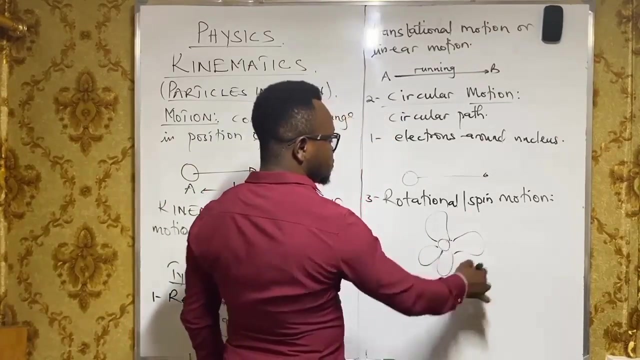 now, this is a type of motion wherein you have a body rotating or spins about its axis. okay, if a body spins about it axis, then we can refer to that as a rotational motion. for example, the blades of a fan. you have a fan here, this is the center and you have the blades around this, so these blades are. 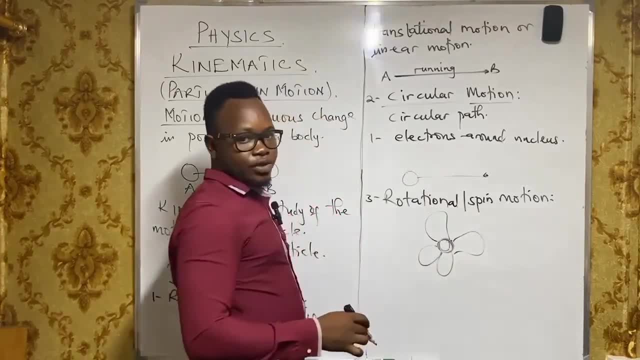 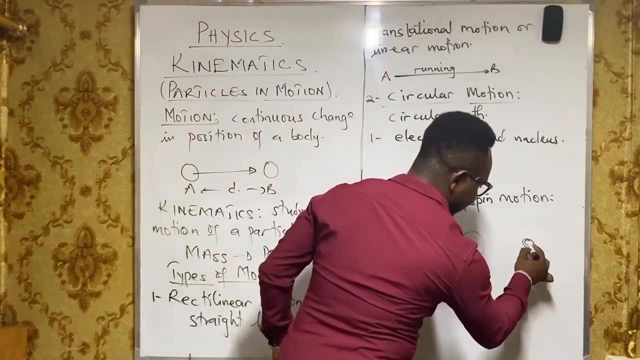 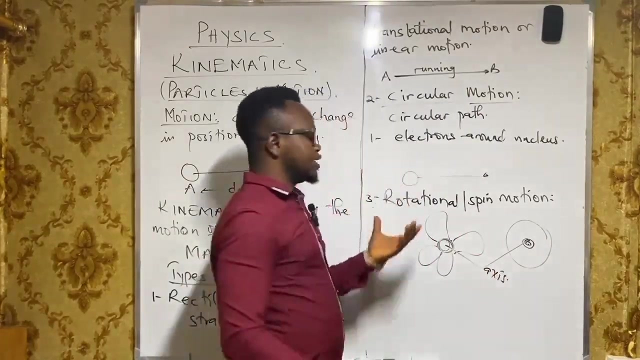 rotating or they are spinning about this axis- okay. or the rotation of a windmill: okay. or the rotation of a wheel, a tire- you have the center here. it rotates about this axis. so if a rotation is taking place about the axis, that type of motion is referred to as irrotational or a spin motion, and 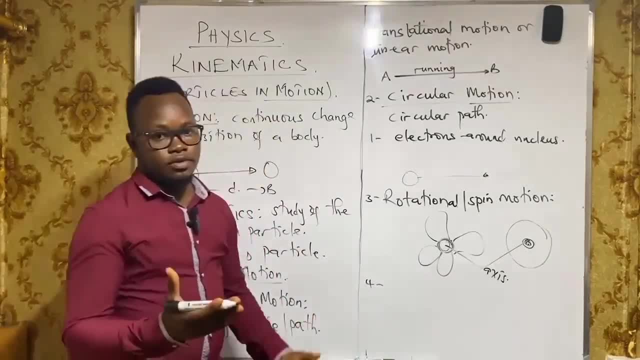 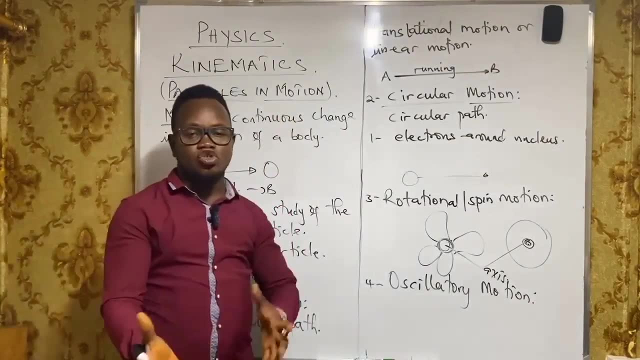 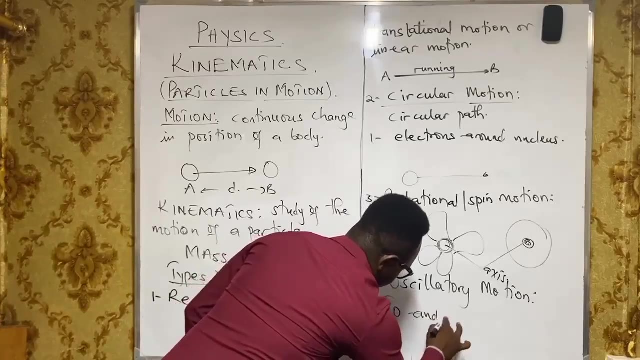 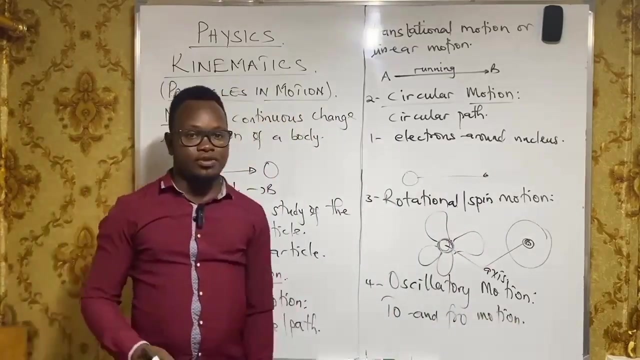 the fourth type of motion we're going to look at is the oscillatory motion. oscillatory motion we can simply put it as a toe and throw motion. if something moves like this, toe and throw, okay. so and throw motion is an example of an oscillatory motion. the simple harmonic motion is a simple example. the shm- okay. 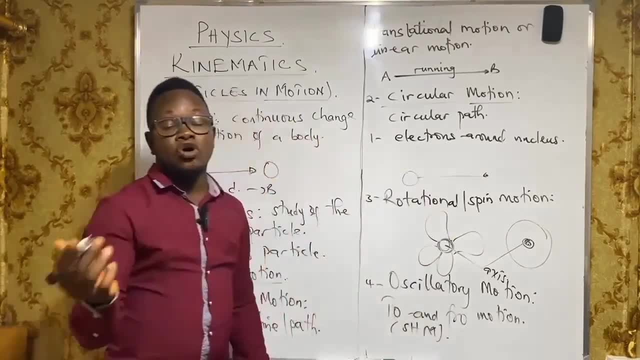 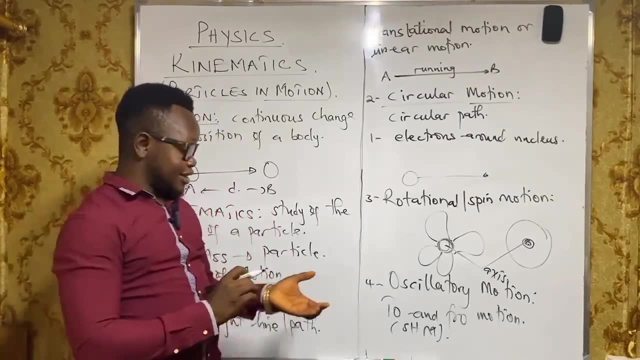 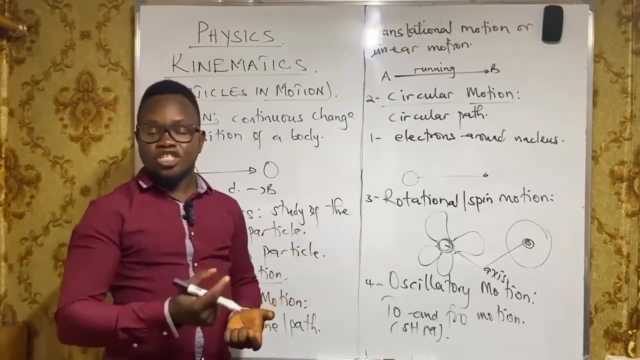 is an example of an oscillatory motion example. we look at the vibrations of atoms at a lattice. that's an example, okay. or we look at the movement of pistons in an automobile engine. that's an example also of a toe and throw motion. or we look at a 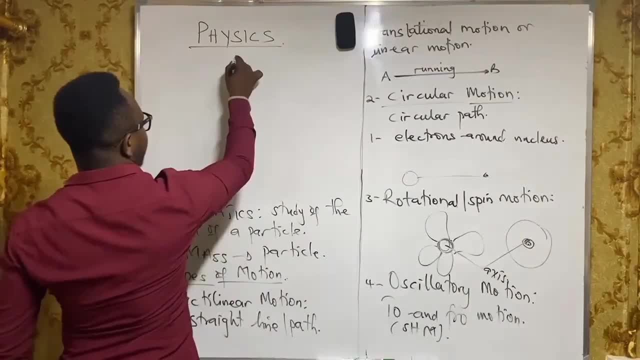 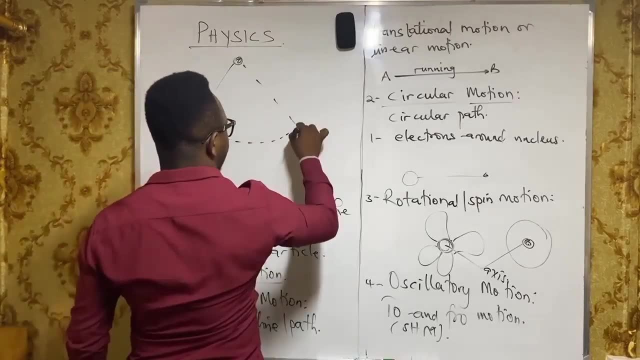 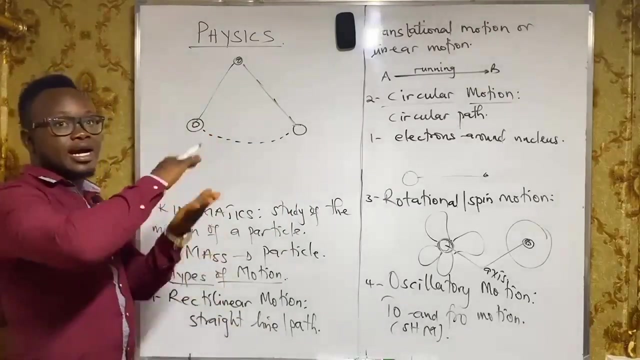 look at a pendulum. let's say, here you have a point of attachment and here you have a string. is the pendulum? this pendulum moves okay and comes here, so it moves to and through, to and through. this is an example. or the motion of a car wiper. you see how the wiper moves to and through in a. 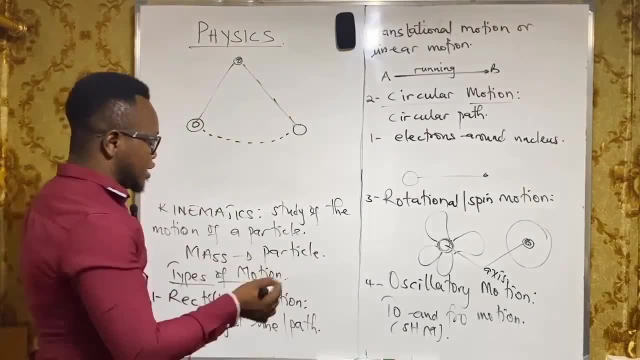 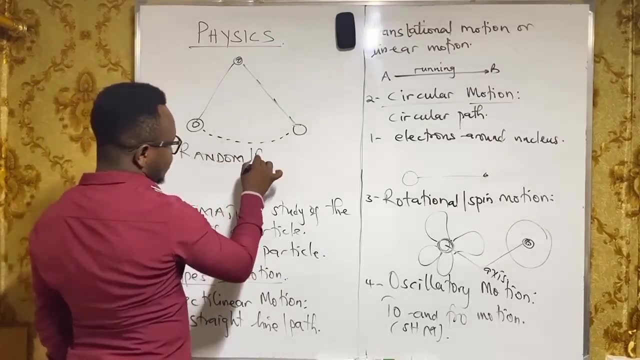 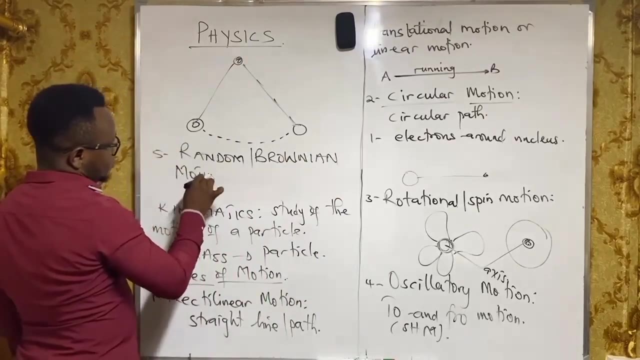 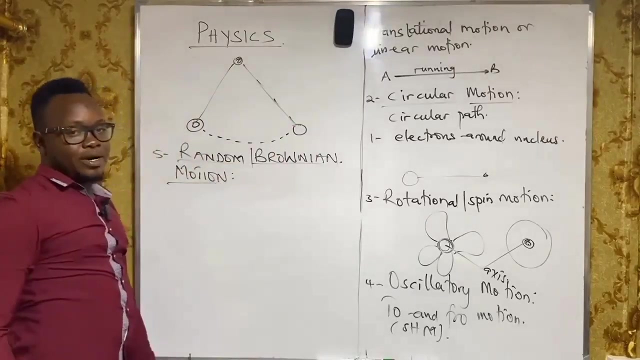 car. so those are examples of oscillatory motion, and the fifth type of motion we are going to look at is a random motion. random, we call it the brownian motion, random or brownian motion, as the name implies: random or brownian. this tells us of the irregular movements of molecules. okay, 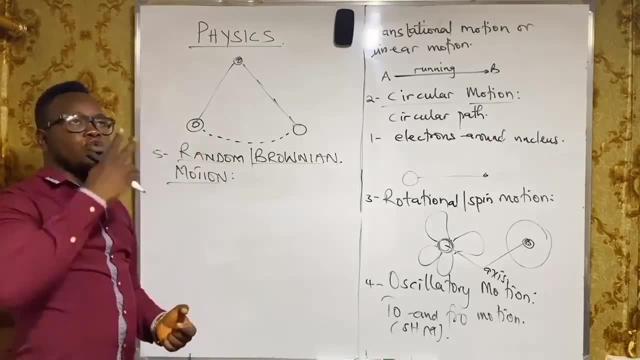 for example, a smoke bean puff in the air when someone smokes and puff it in the air. or, for example, a smoke bean puff in the air when someone smokes and puff it in the air. example: the suspension of particles in water. you see them just moving about in a random manner. 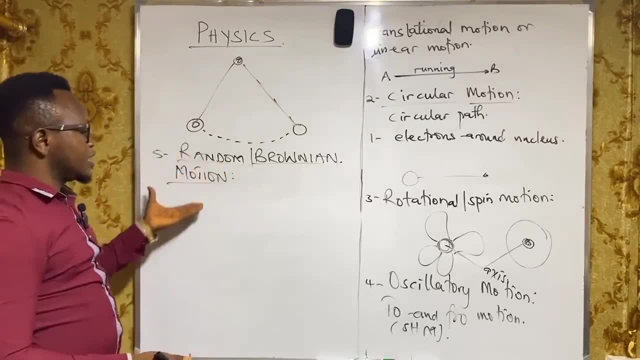 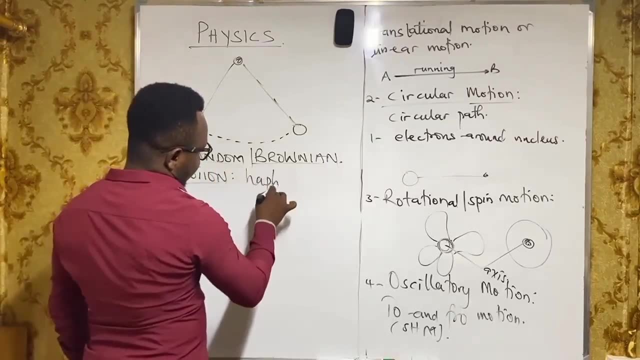 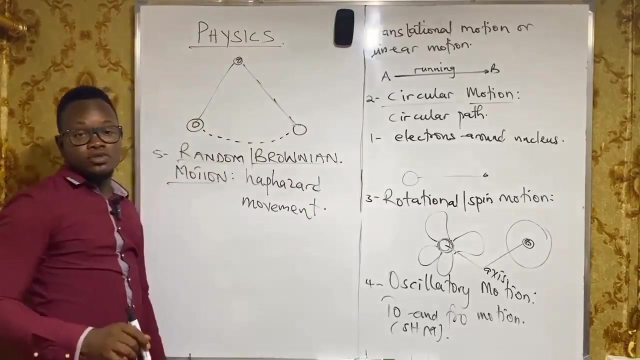 yeah, meaning there is no fixed path. okay. so this hair means random motion, motion that works havasadly, so there is a havasad movement of the molecules. so when there is havasad movement of the molecules or the particles, then we refer to that as a brownian or a random motion. so next we are. 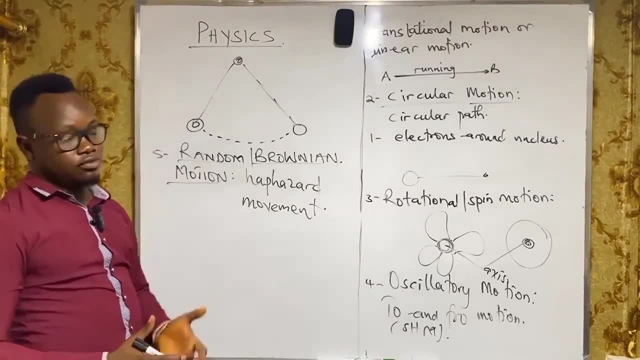 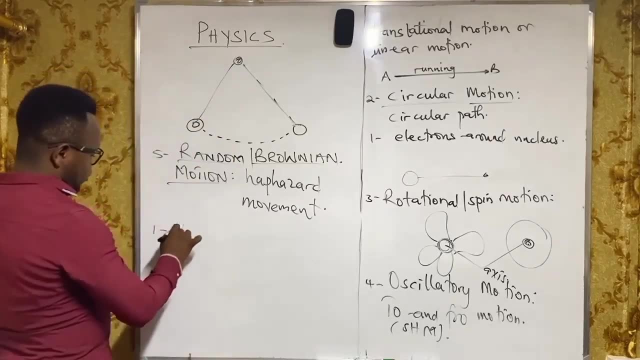 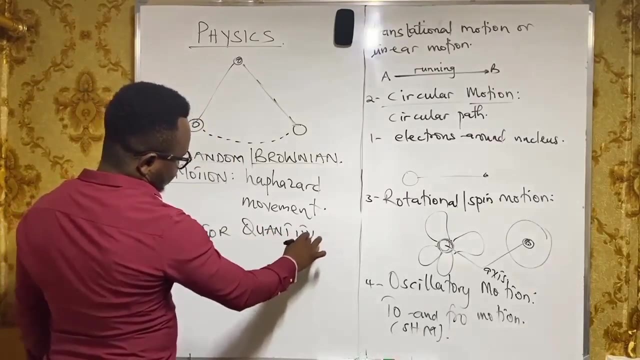 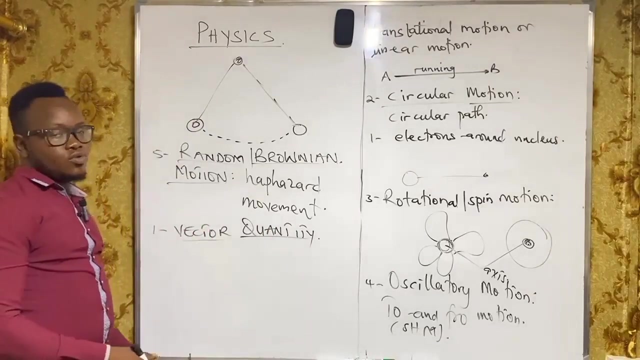 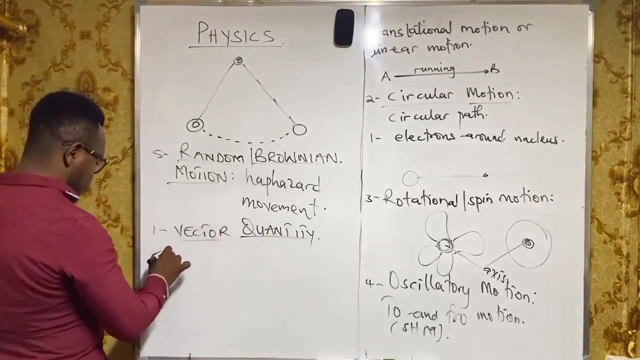 going to look at some basic definitions of some of the key things we'll be looking at under kinematics in key quantities. one we start with a vector quantity. now what is a vector quantity? a vector quantity is a quantity whose magnitude or size and direction are known. so a quantity of known magnitude. 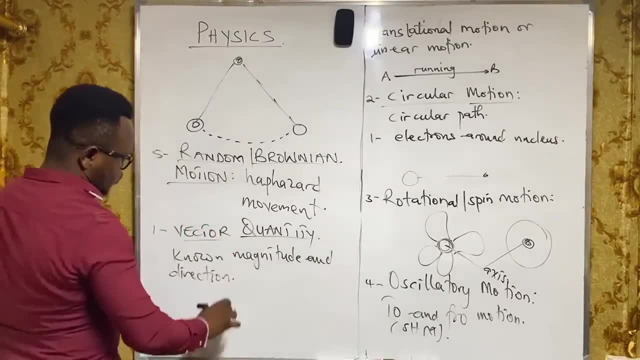 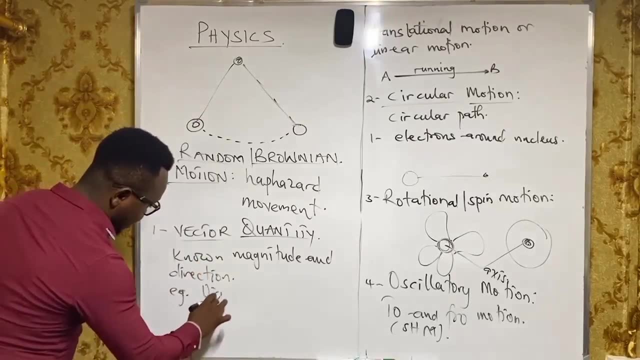 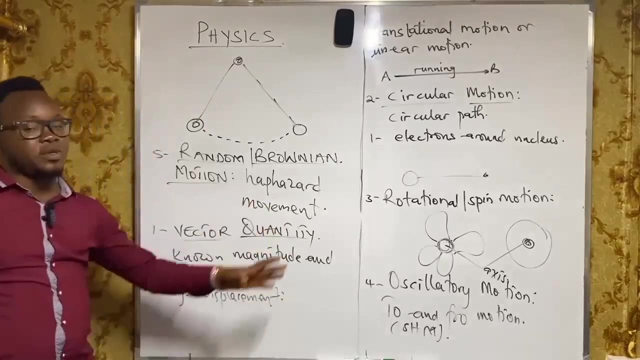 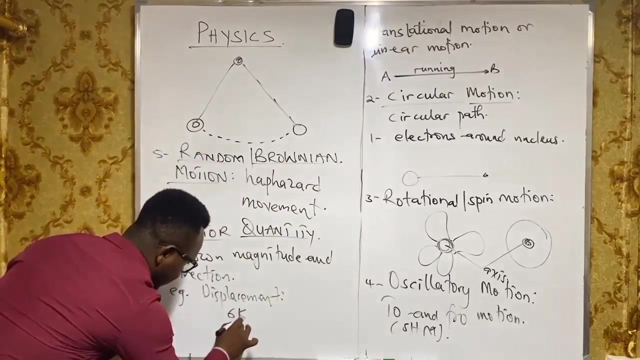 and direction. we can refer to that as a vector quantity. examples of vector quantity one we can look at displacement. okay, as we know, displacement is the distance moved in a specified direction. for example, we say a boy runs six kilometers due east. okay, six kilometers due closed east. this is an example of 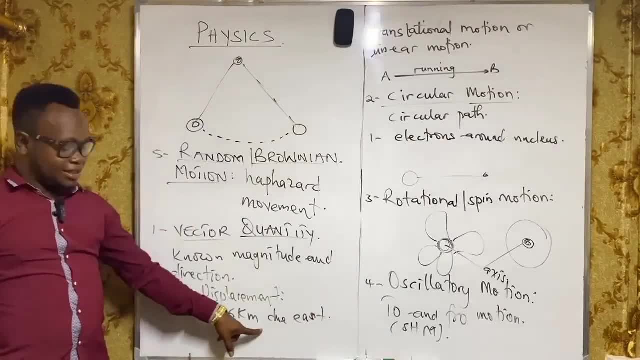 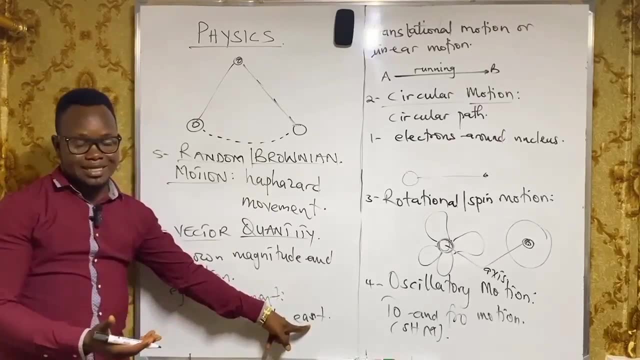 a vector quantity, because you are given the size or the magnitude of the distance the boy is covering and then the direction towards which the boy is heading. so this is an example of a vector quantity. we will look at that later in a moment. so for those of you who have had experience in law ofbringen and you don't know navigating, just like me- 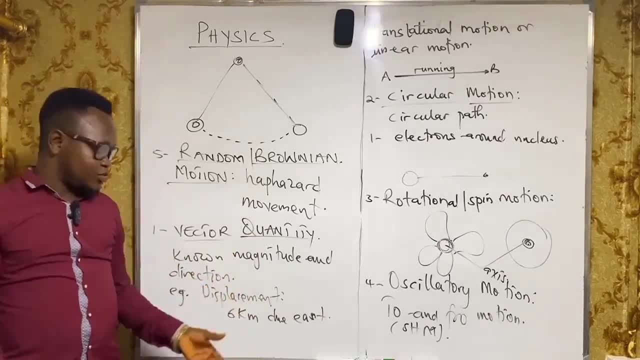 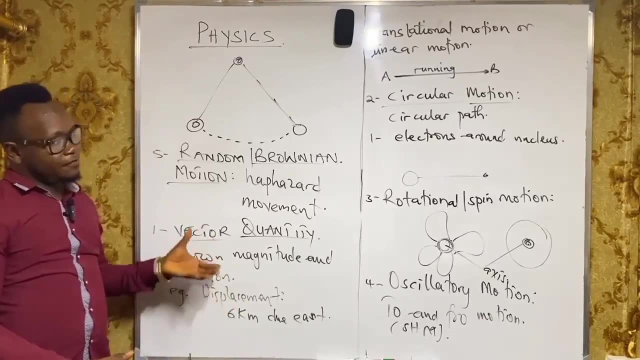 for any of you who have done backpacking before talking about advertising. now there is a question to be answered in the far African scientific point of view of a vector quantity. we can look at weight. as we know, weight is mass times gravity, so it is also an example of a vector quantity. so any quantity whose magnitude and direction are known, 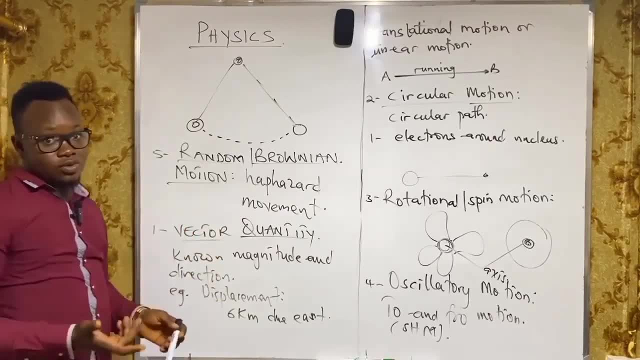 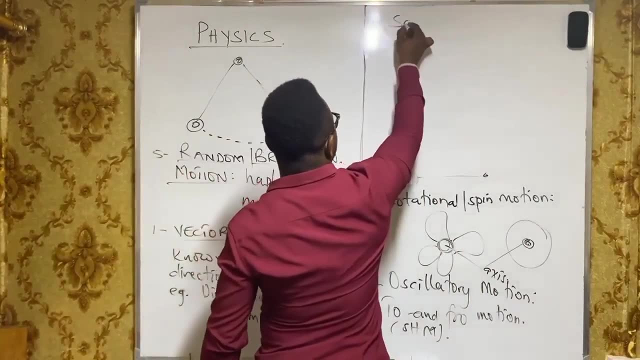 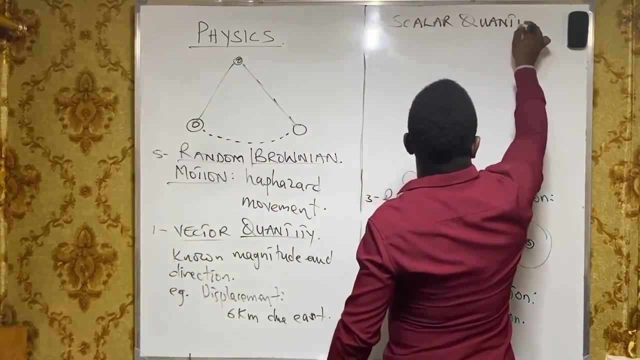 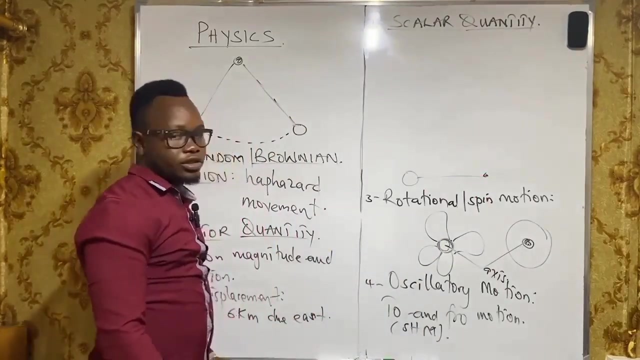 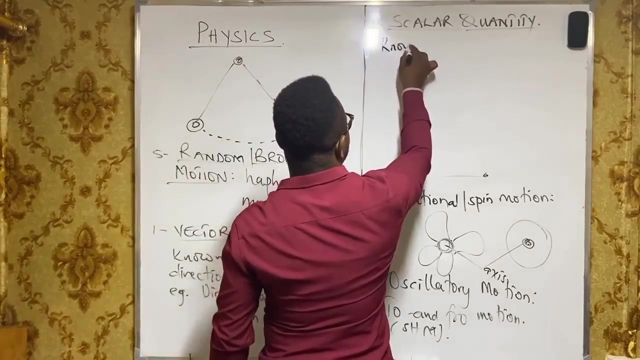 can be referred to as a vector quantity. so next we look at scalars. so next we look at scalar quantity. a scalar quantity is a quantity whose magnitude is known but has no direction. known magnitude is a quantity whose magnitude is known but has no direction or size. 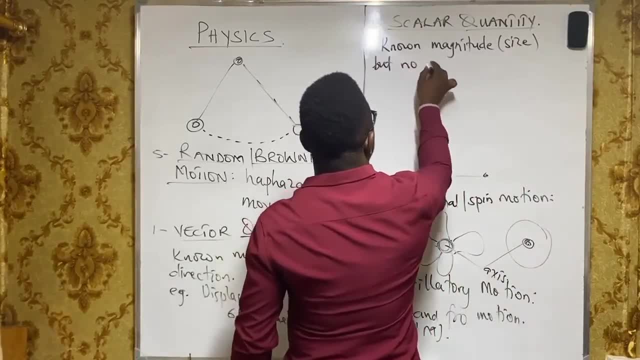 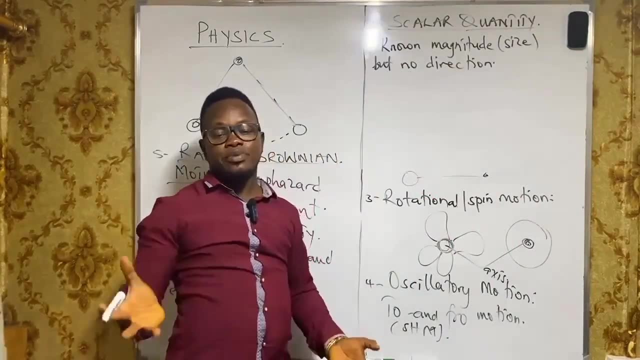 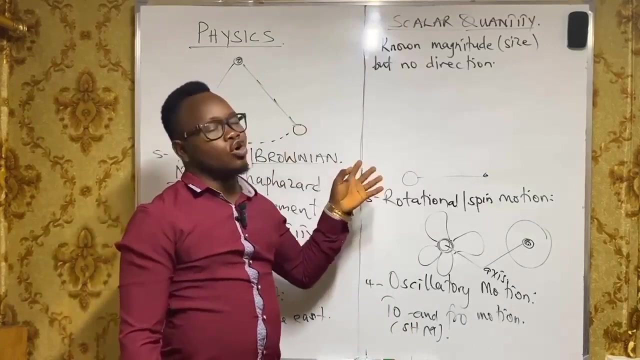 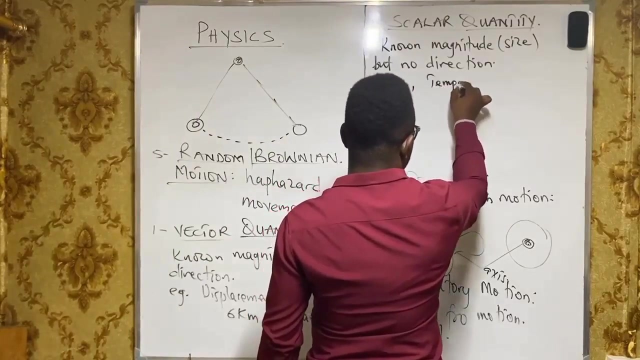 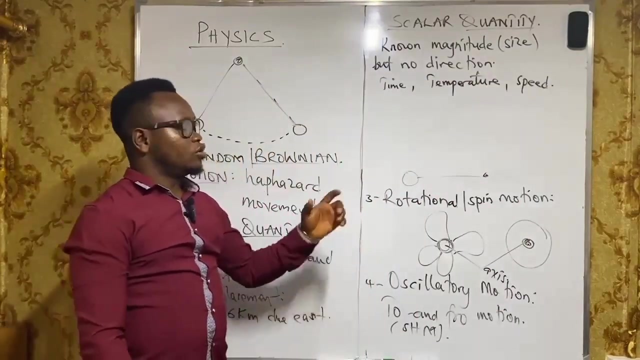 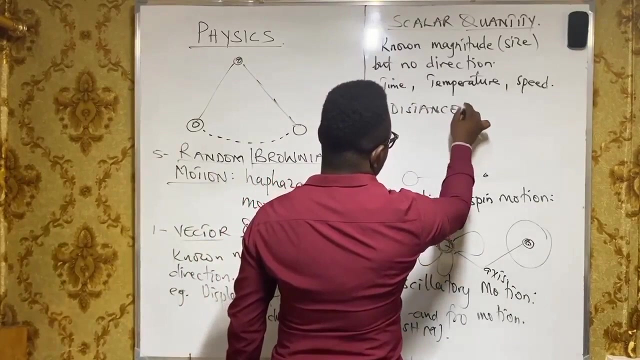 but no direction. for example we can look at here: we say temperature, okay. we say time, we say speed. these are all examples of scalar quantities. so time is an example, temperature, speed. so these are examples of scalar quantities. next we look at distance. distance we say is the interval? 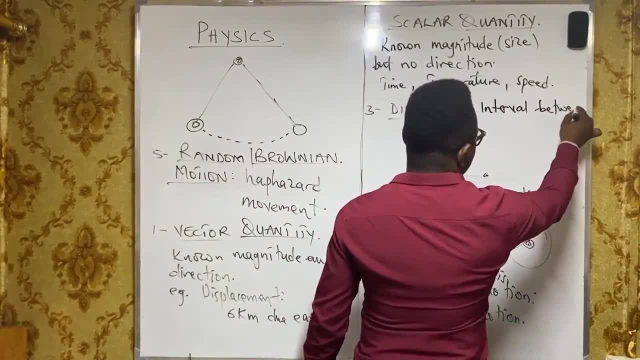 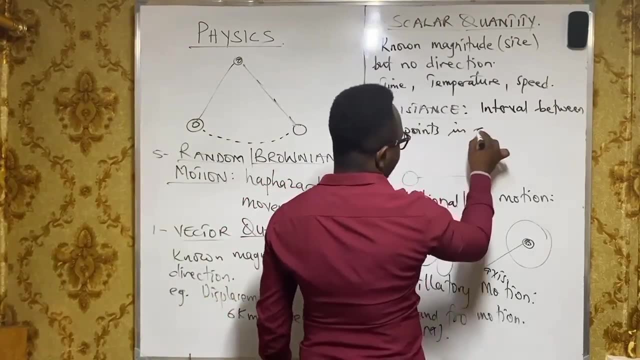 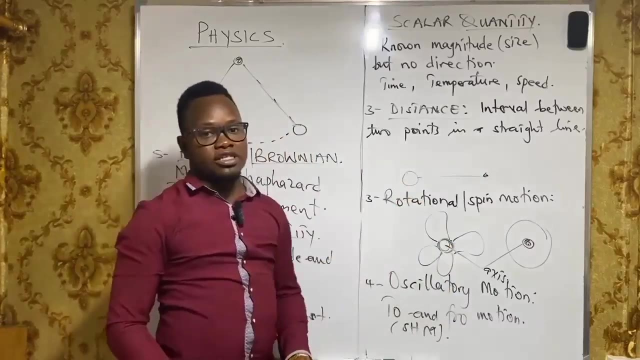 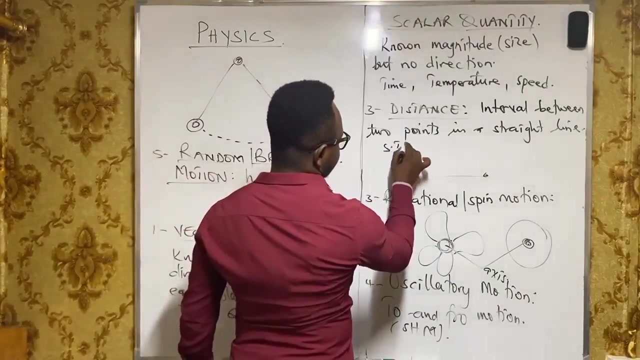 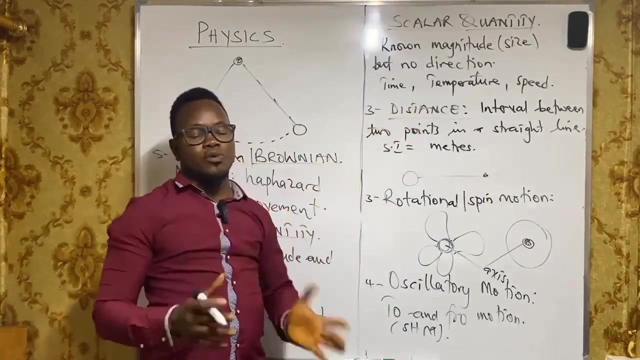 between two points in a straight line, between two points in a straight line. we refer to it as distance and it is measured in a standard unit. it si unit is the meters. okay, we measure it in meters. so the interval between two points in a straight line will refer to it as distance. 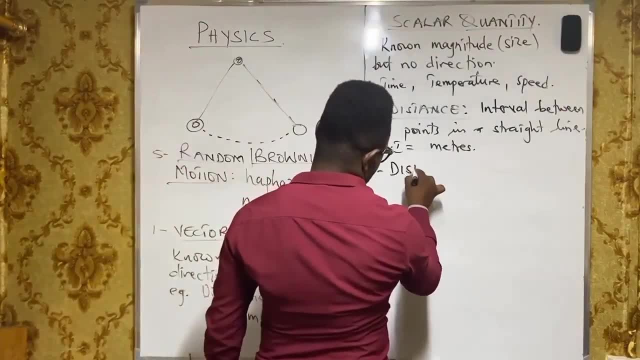 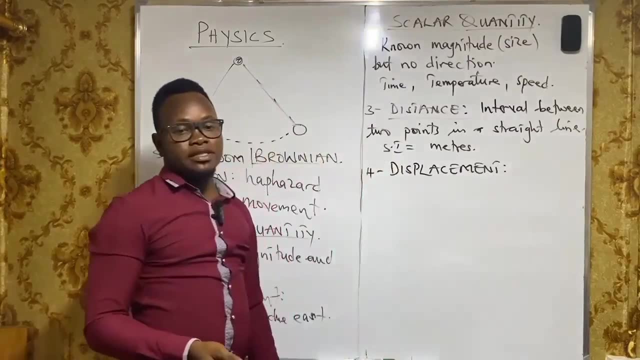 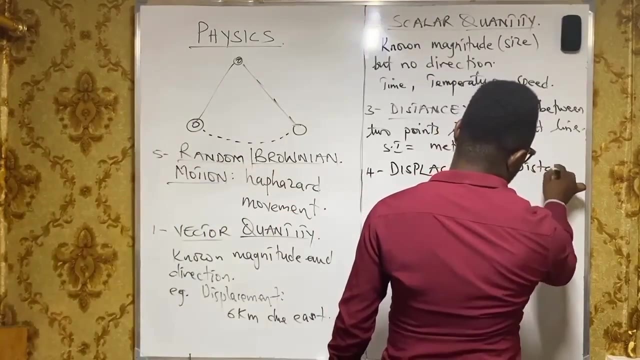 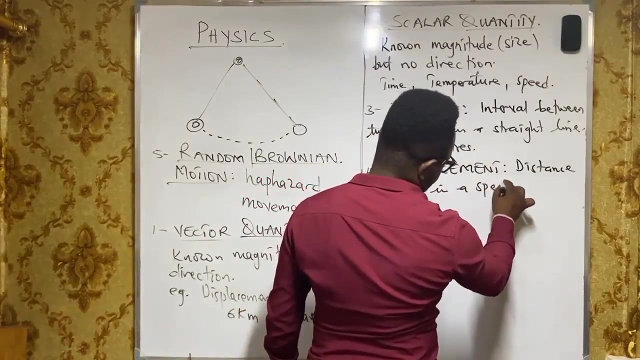 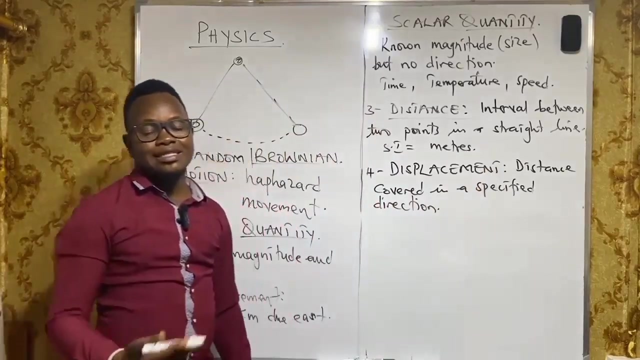 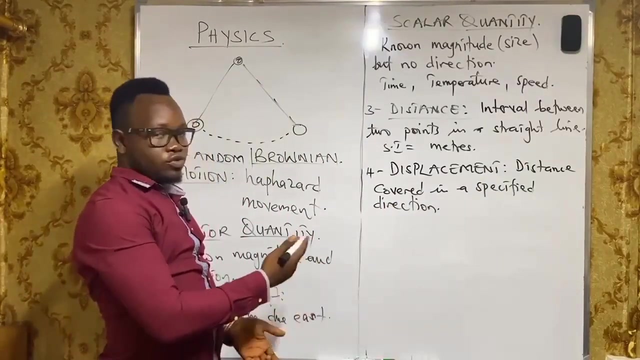 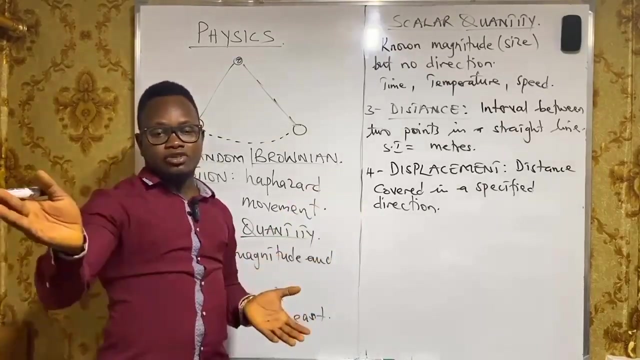 next we look at displacement. next we look at displacement. displacement simply means the distance covered in a specified direction, distance covered in a specified blue area, close choice. for example, we say the girl round 100 kilometers towards the west. so that is a displacement because you're given the distance and you're given the direction towards which the girl is heading. five, 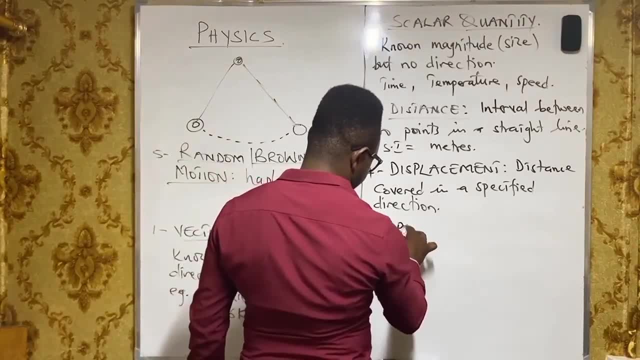 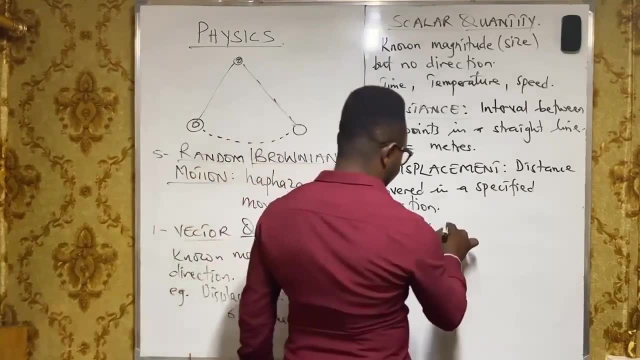 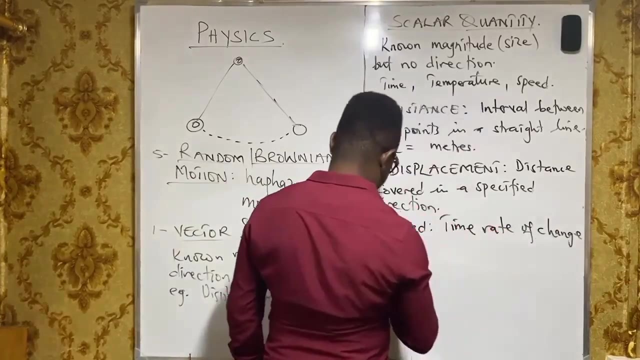 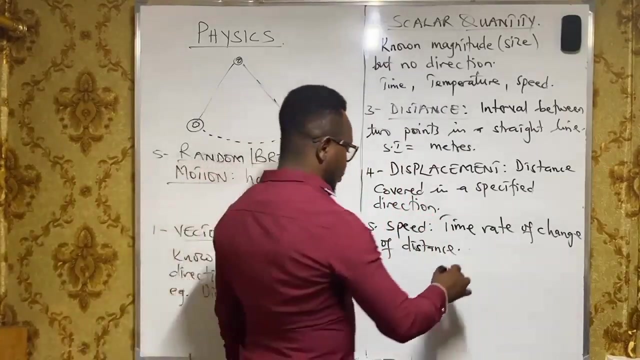 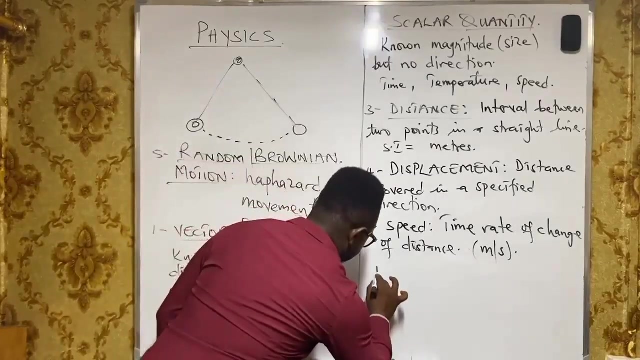 more plot. Forest five. Speed Speed is the time rate of change of distance, and speed is measured in meters per second. okay, It is measured in meters per second. So mathematically, speed can be stated as: so speed here will be equal to distance covered. 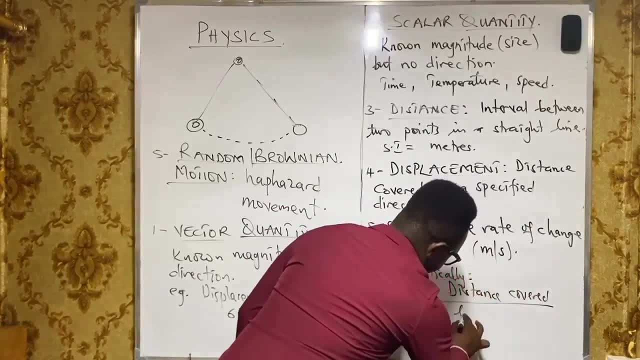 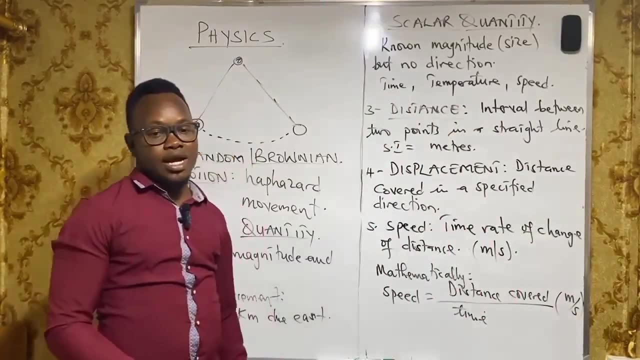 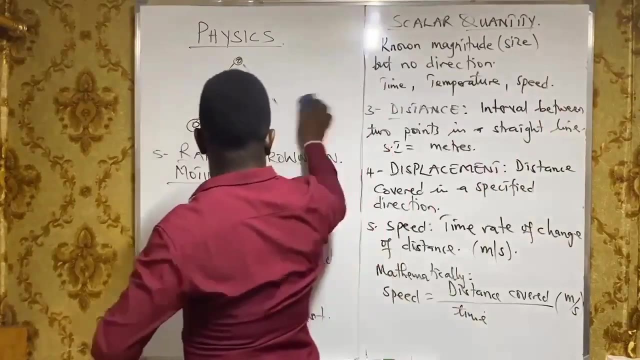 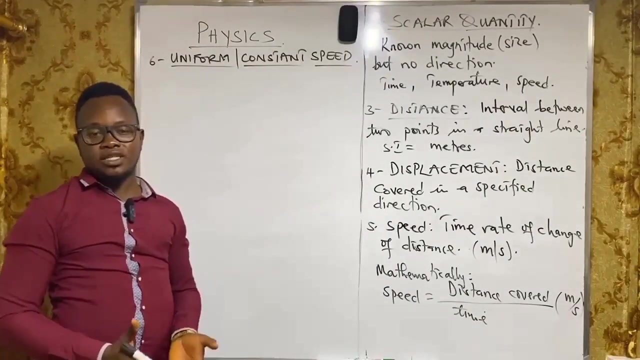 over the time will give us meters per second. So next we look at constant speed, or we call it uniform speed, Uniform or constant speed. A body is said to be moving with a uniform or a constant speed if it covers equal distances in equal 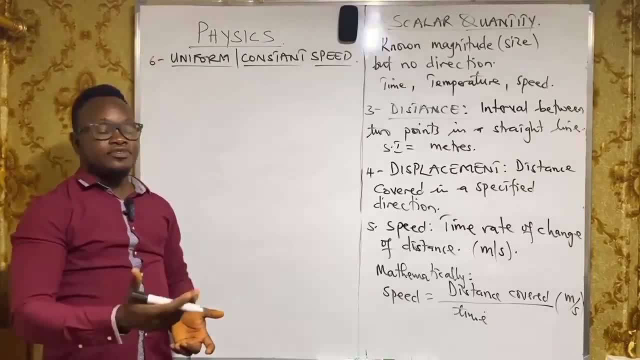 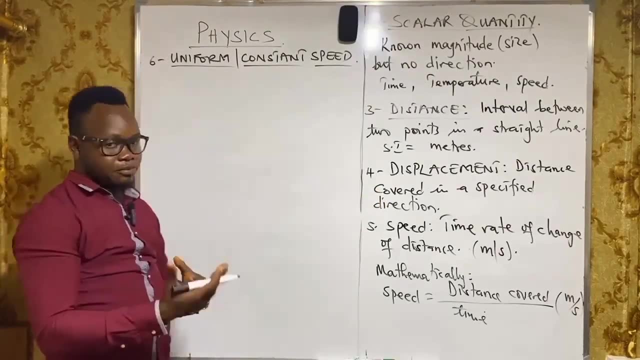 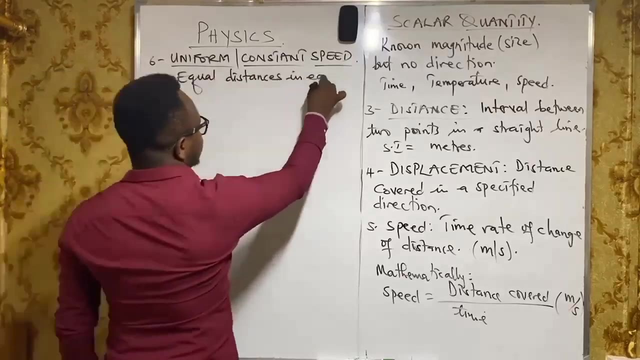 timings okay, Or if the time rate of change of distance is constant. When the time rate of change of distance is constant, then the body is said to be moving with a uniform speed. that we say the speed is uniform, So equal distances in equal time, or the time rate of. 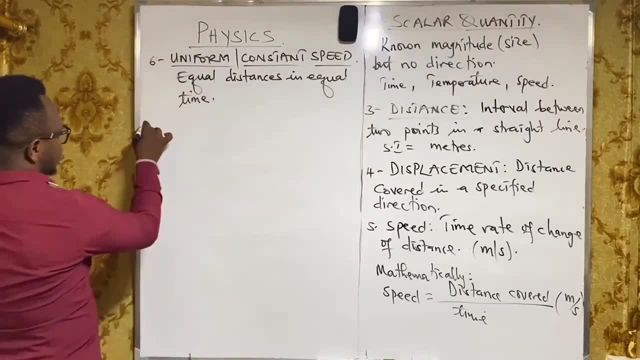 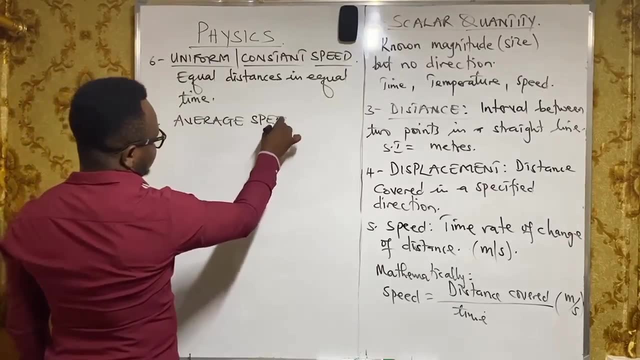 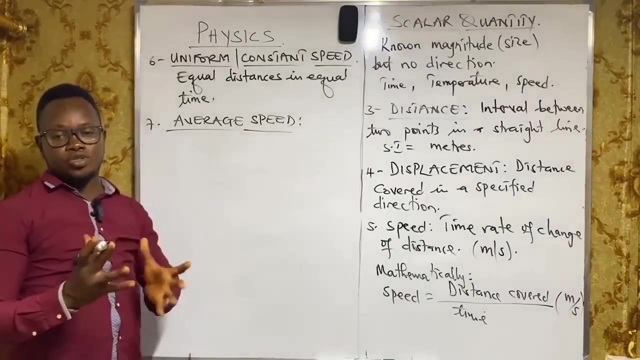 change of distance to be constant. Then we can say the speed is uniform or constant. Next we look at average speed. Of course this one here tells us of the ratio- okay- that exists between the total distance traveled, the total time taken. 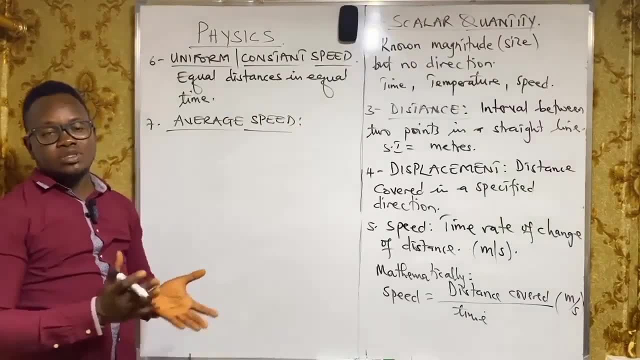 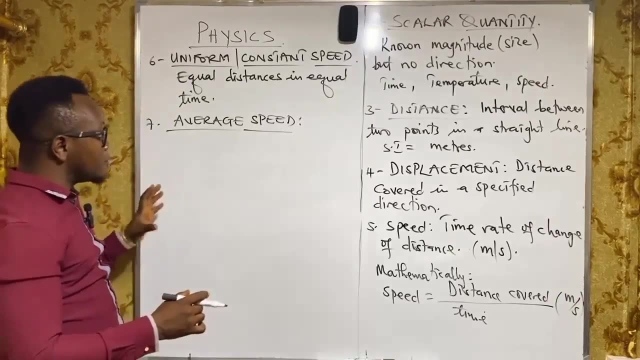 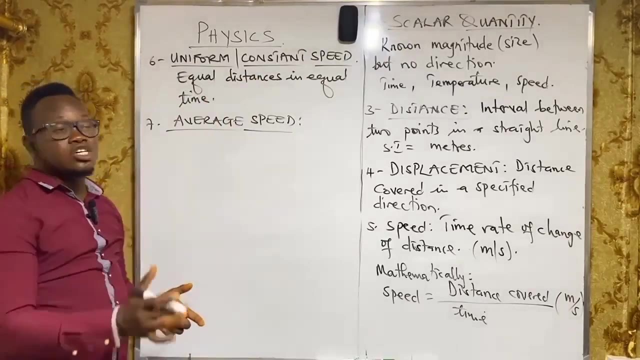 So the ratio of the total distance traveled and the total time taken to cover that distance is what we call average speed. okay, And we should note that if a body is moving with a uniform speed or constant speed, its average speed is equal to the uniform or constant. 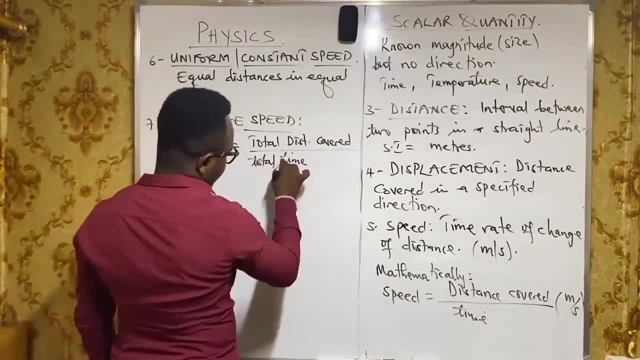 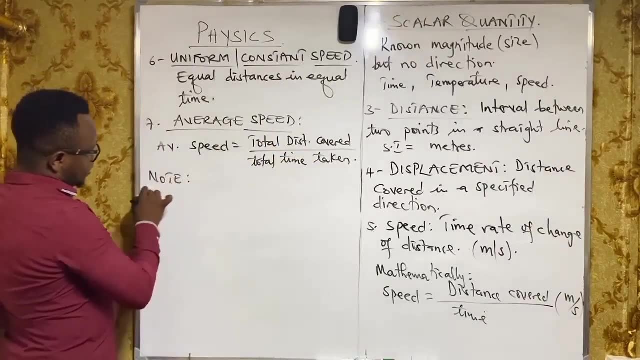 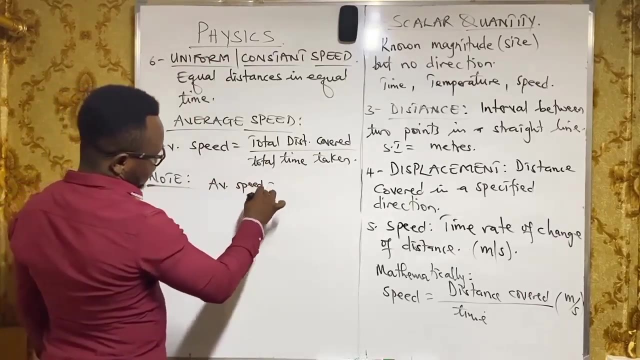 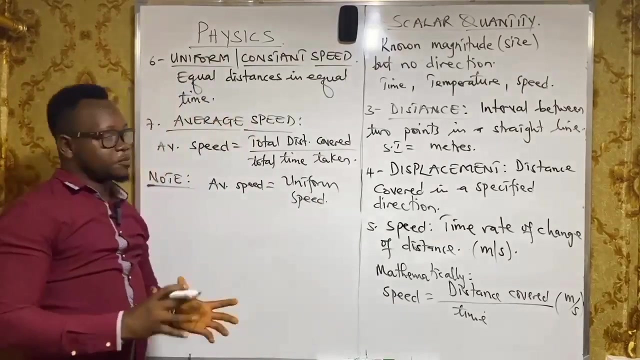 speed. So we have to note that. So the ratio of the total distance covered upon ratio of total time, And you notes that if it is moving with a uniform speed, then the average speed is equal to the uniform speed, meaning if the speed that the body is moving with is constant, 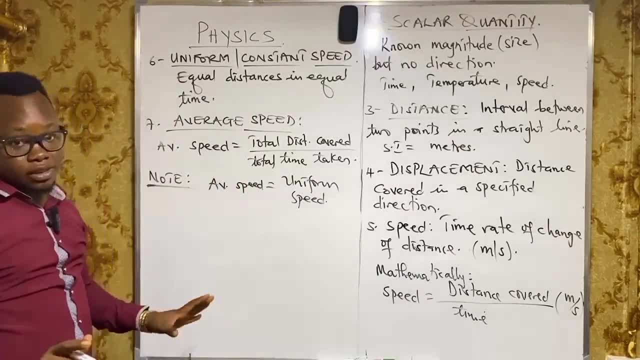 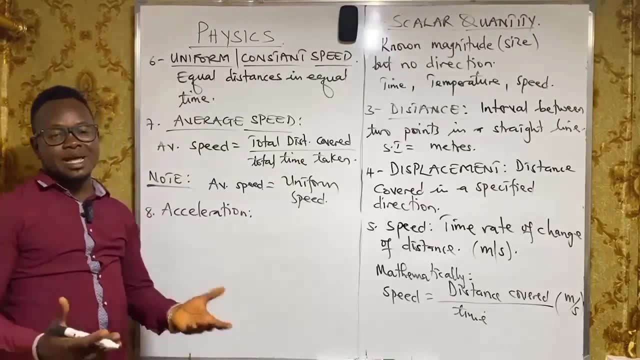 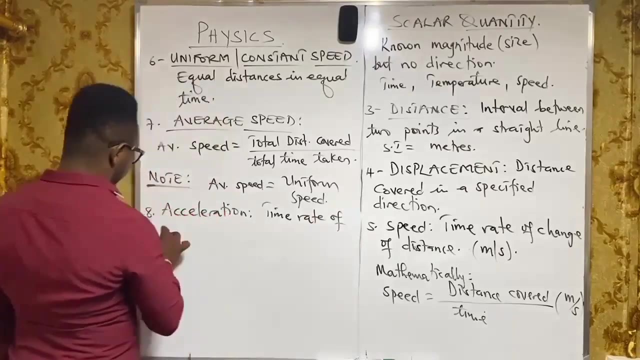 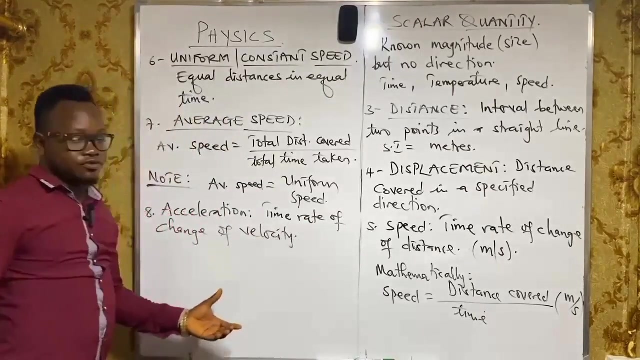 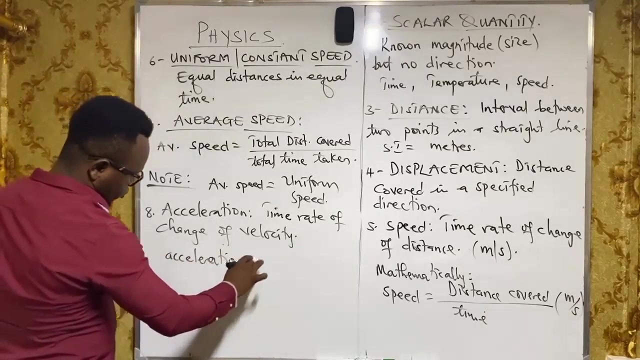 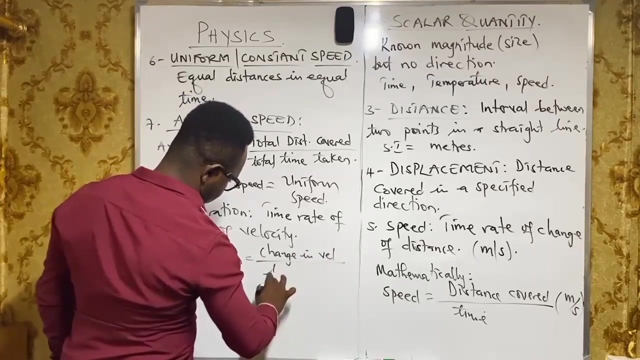 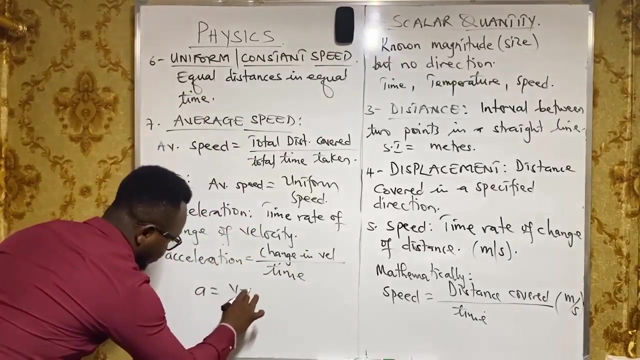 so the average speed and the uniform speed are going to be equal. eight acceleration. so acceleration tells us of the time rate of change of velocity. so the time rate of change of velocity is called acceleration. so acceleration is equal to change in velocity upon time. so it is the time rate of change of velocity, meaning acceleration will be equal to. 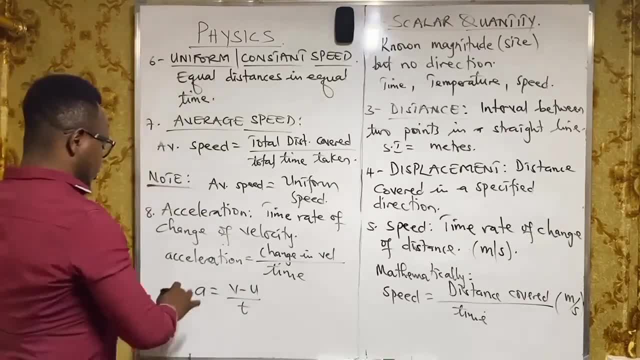 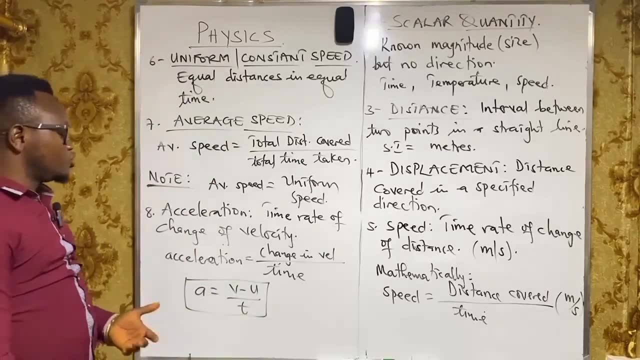 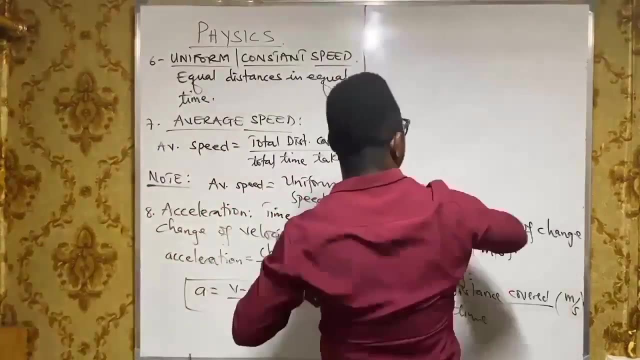 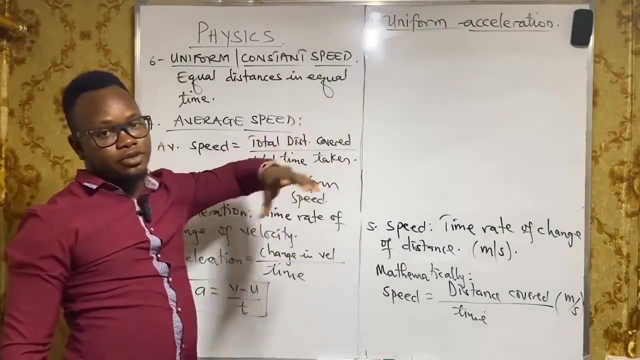 changing velocity upon time. okay, so next we look at uniform acceleration, and acceleration is said to be uniform or constant if the time rate of change of velocity is constant. so if the time rate of change of velocity is constant, then the then the acceleration is said to be a uniform or a constant acceleration. okay, 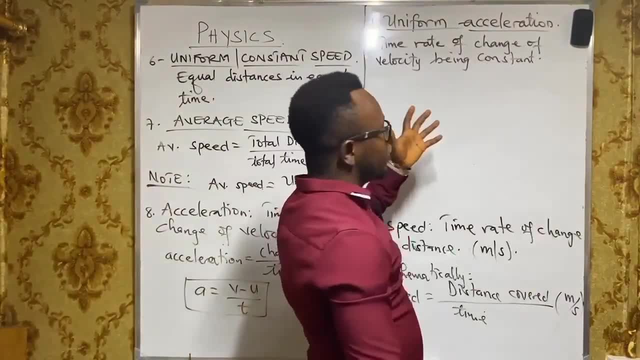 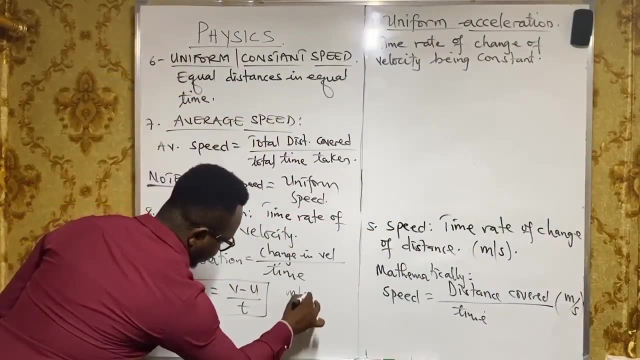 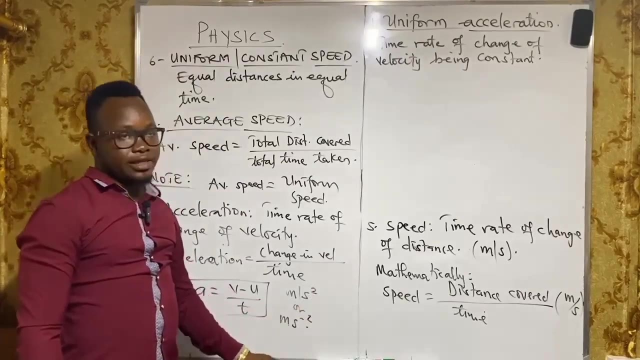 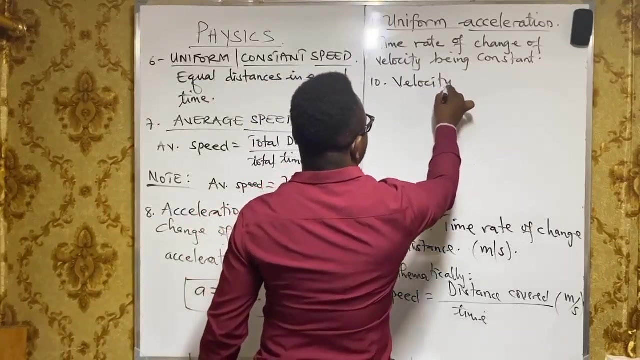 and we should note that acceleration is measured in meters per second square. this is meters per second square, okay, so either write it like this or write it like this. it means meters per second square. so then we look at velocity. velocity is the time rate of change of displacement. 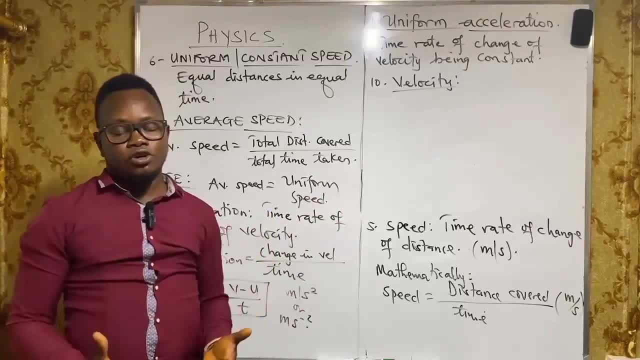 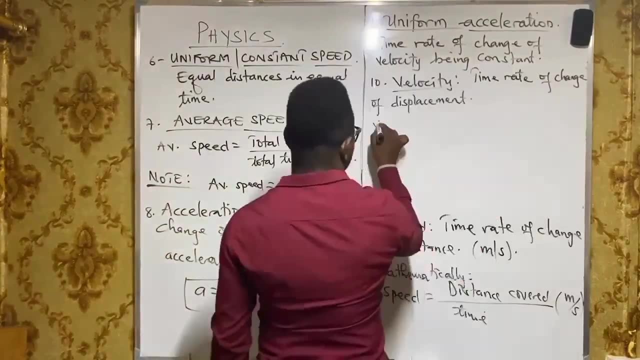 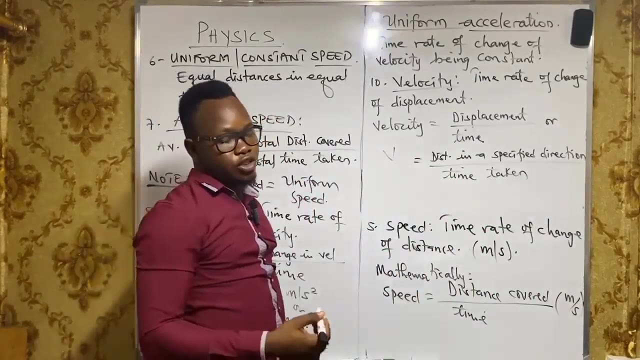 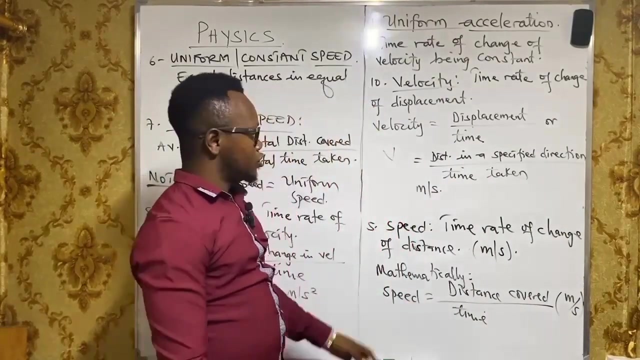 that is the displacement distance moving a specified direction upon time. that's what refers to us: velocity, the time rate of change, of displacement. or we say it is distance in a specified direction upon time and, mind you, it's that it is a short term that we are just moves about at that stretch of немножко. 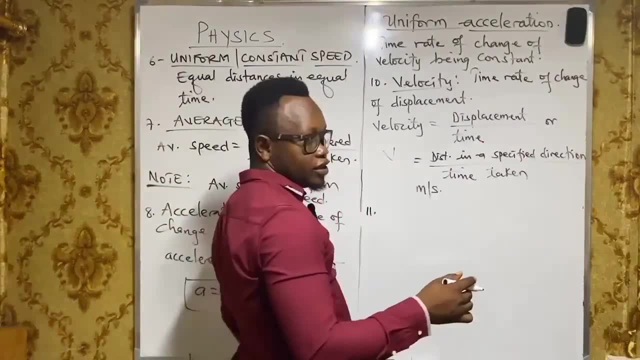 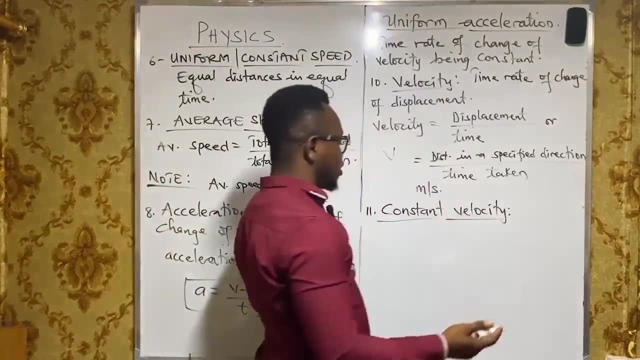 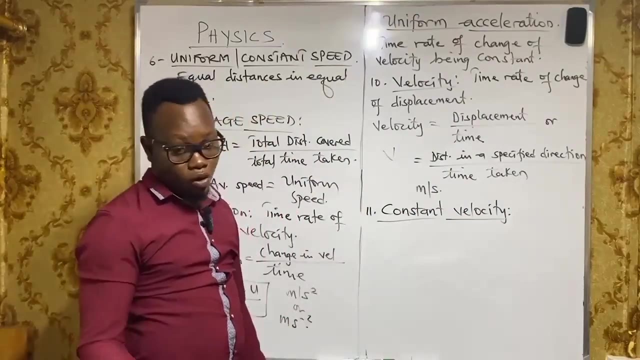 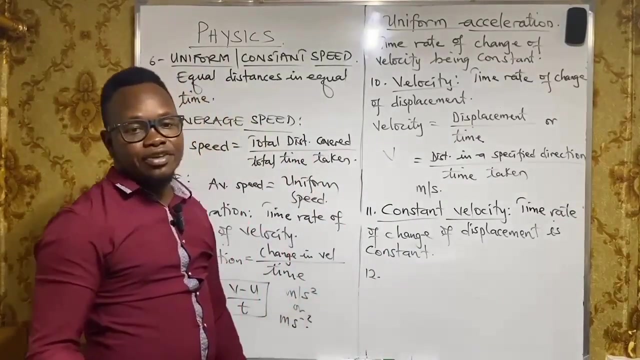 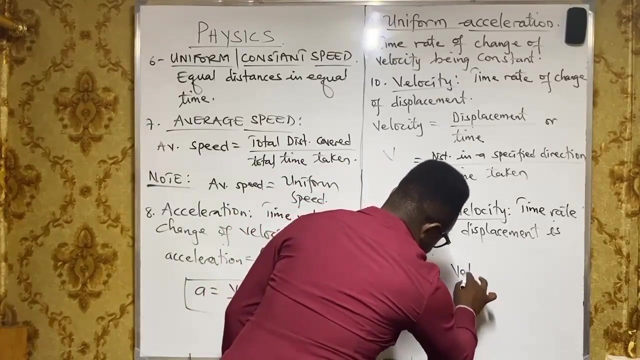 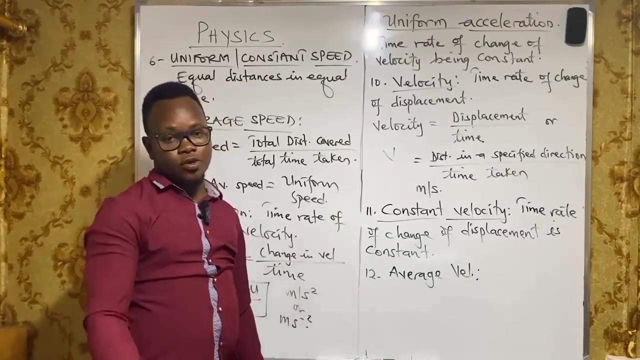 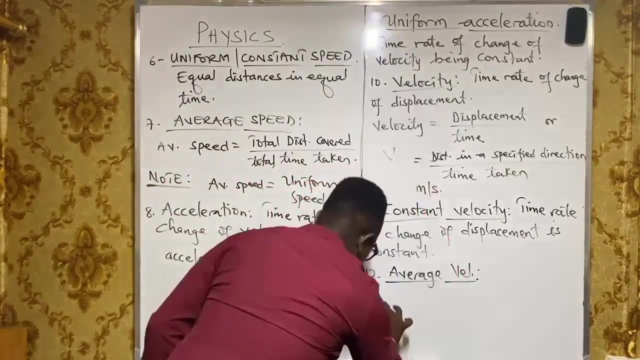 so let me see. yes, do you attribute? yeah, oh, so say, if F going to my name now say differences, spin 're correct. running velocity: average velocity tells us of the ratio of the total displacement upon total time. so the ratio of the total displacement upon total time is what we mean by the average. so next we look at: 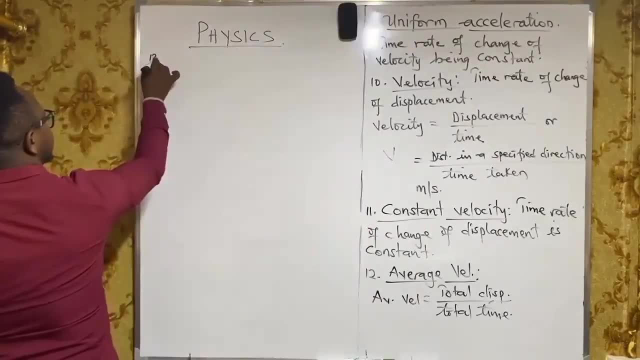 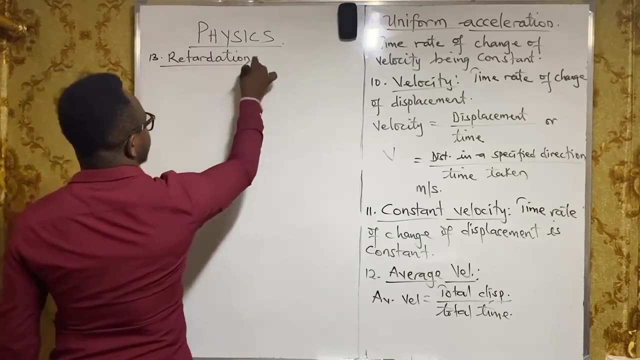 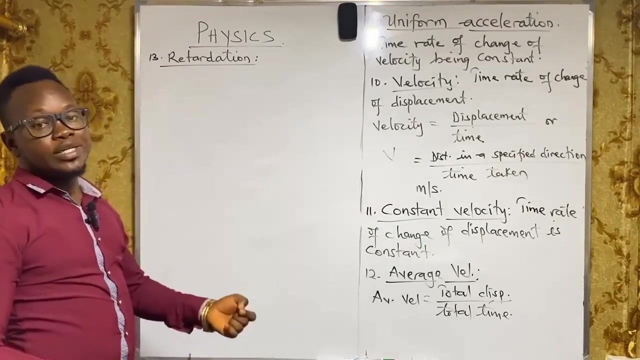 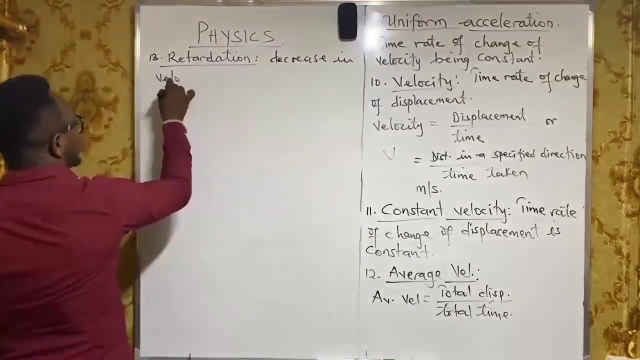 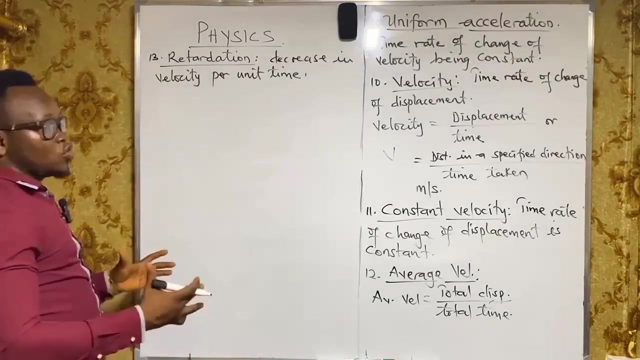 retardation, of course, rita dashon hair, simply means the decrease in velocity per unit time. when the velocity decreases per unit time, referred to it as retardation. so the decrease in velocity per unit time is known as retardation, and retardation occurs when the velocity goes down, so retardation, we should also know that is the. 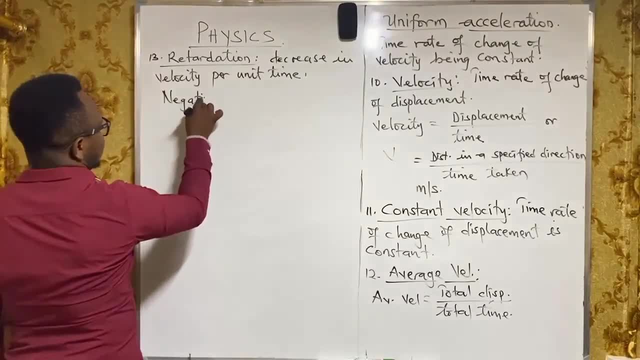 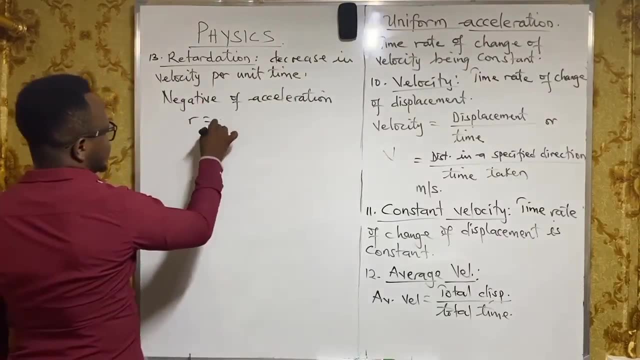 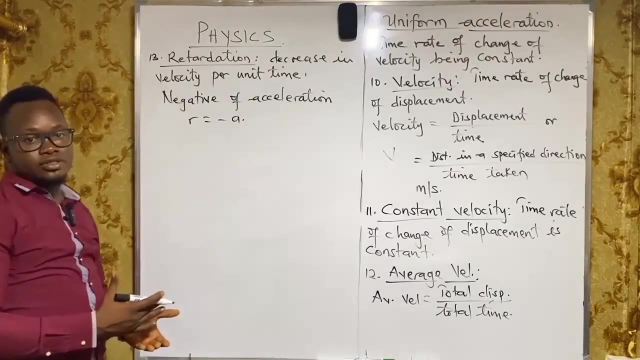 negative of acceleration, negative of acceleration. so meaning retardation r is negative a, so it is the negative of acceleration. because if acceleration tells us of the increase in velocity per unit time, and then this one here brings about a decrease in velocity by any time, then retardation is negative of. 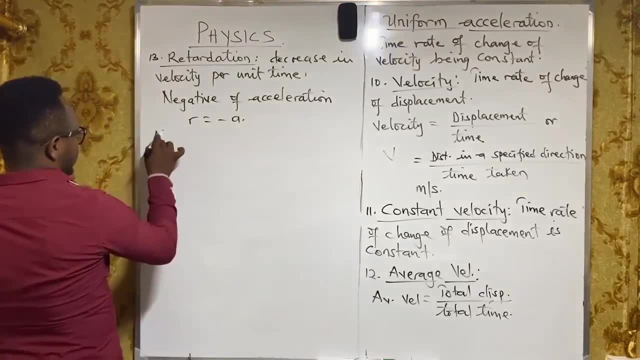 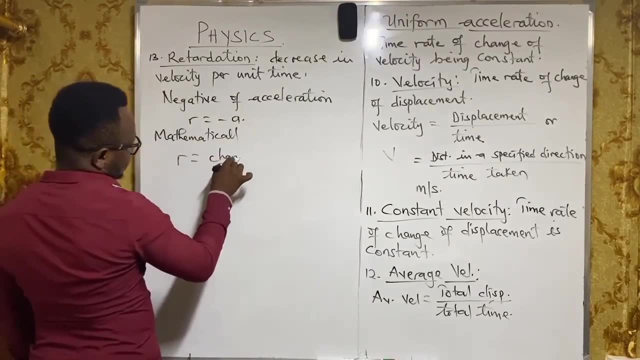 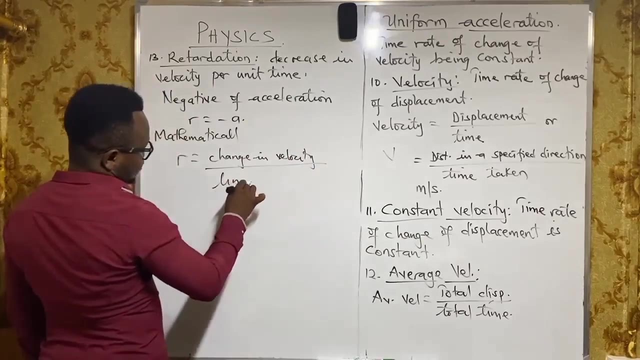 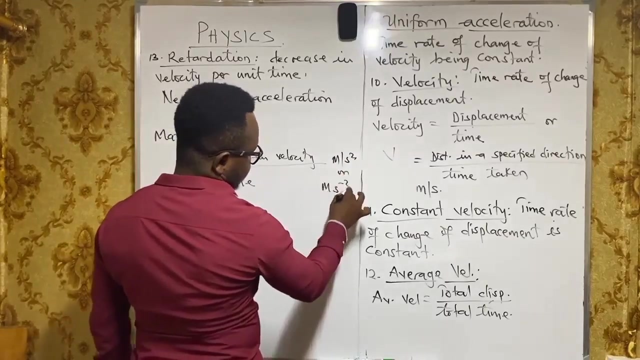 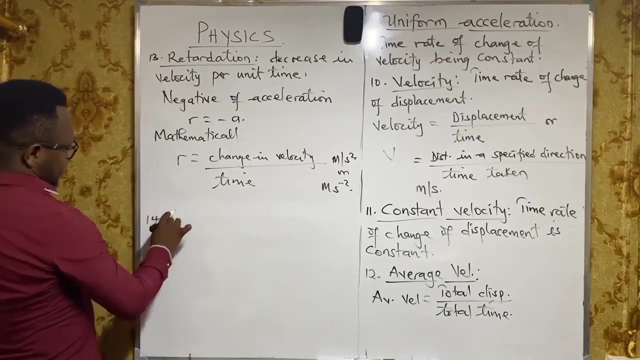 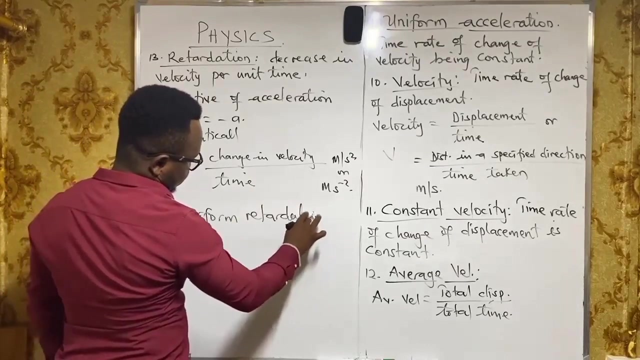 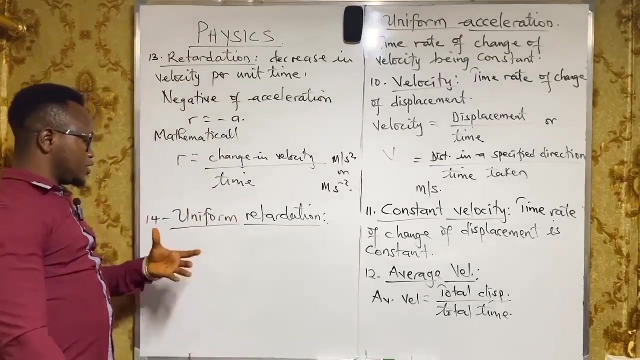 acceleration, meaning it is the reverse. so we can state this mathematically: the retardation is changing velocity over time. and if units is also meters per second square, okay, eight unit is meters per second square. next we look at this uniform retardation. a body is said to be retarding uniformly, or a body is said to have a uniform retardation if the 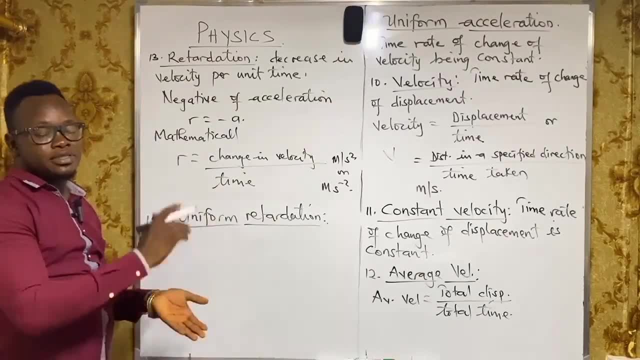 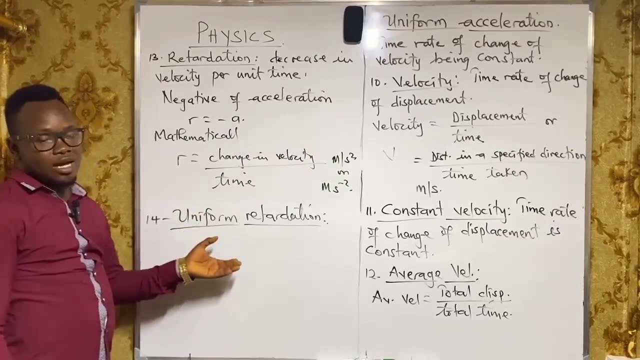 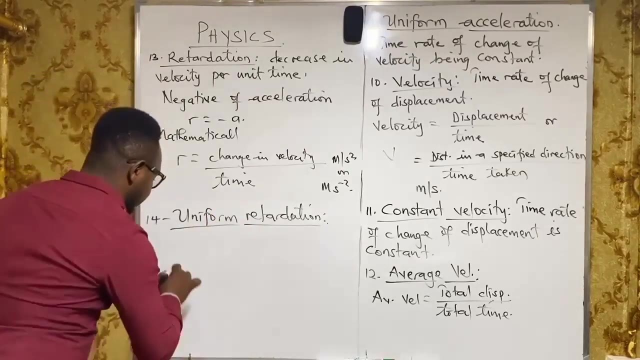 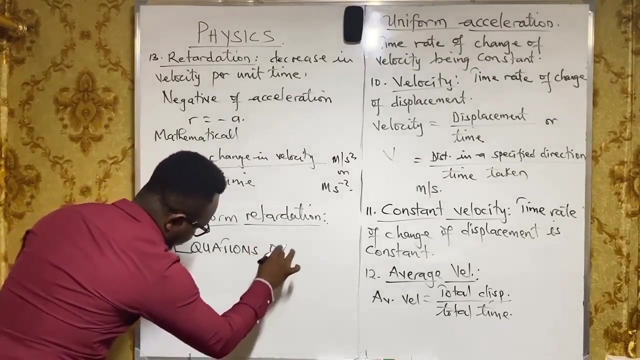 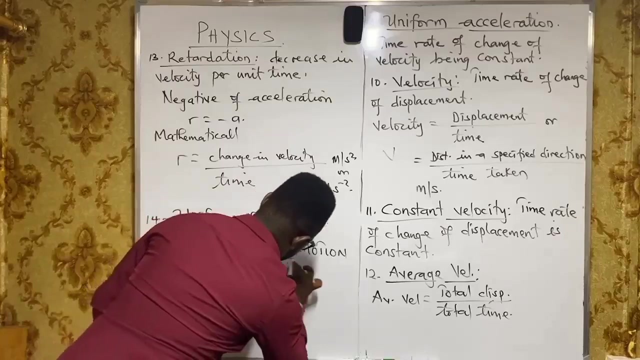 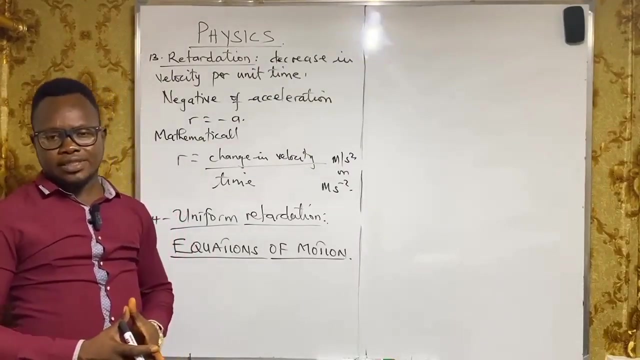 velocity is decreasing by equal amount in equal time. so the equal amount of decrease in velocity in equal timing is said to have a uniform retardation. okay, so from this we can look at the equations of motion. so for us to look at the equations of motion we are going to consider. 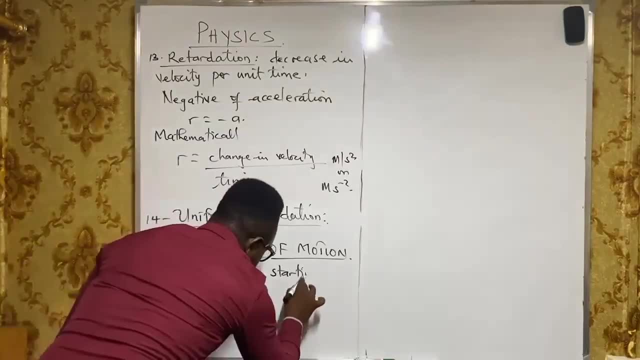 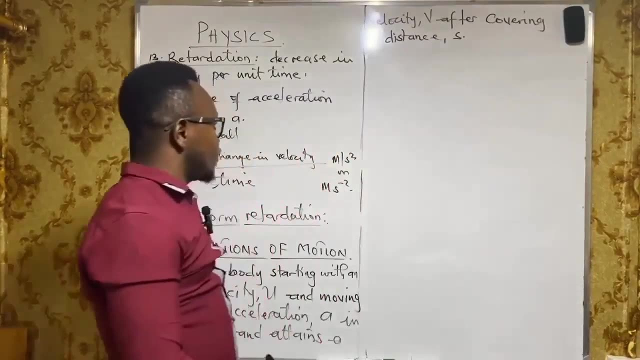 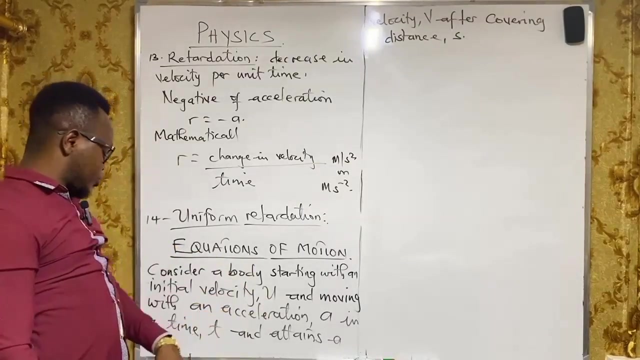 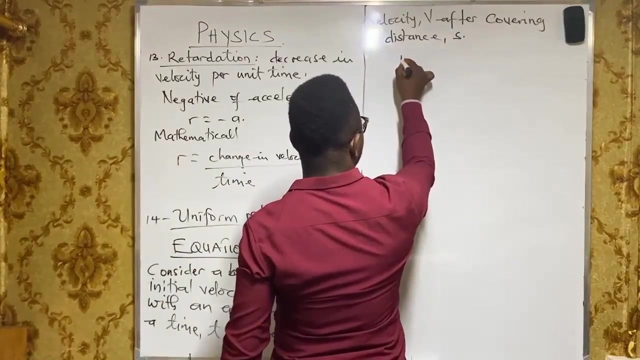 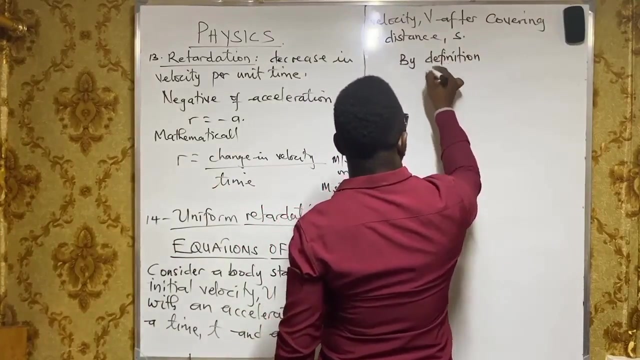 a particle or a body starting. so now we say: consider a body starting with an initial velocity u and moving with an acceleration a in a time t and attains a velocity v after covering a distance s. so if we look here, by definition we want to look at acceleration. 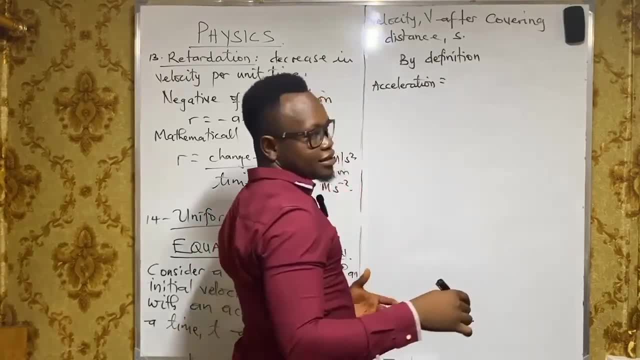 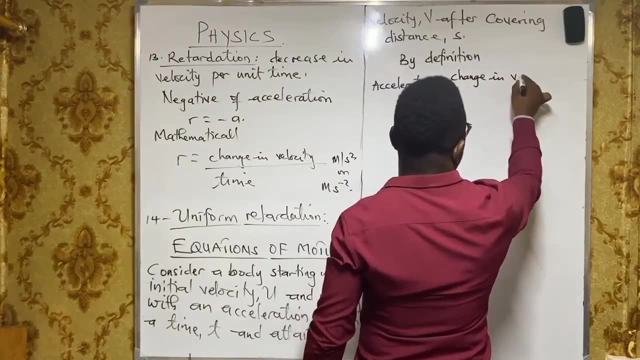 we said, is a time rate of change of velocity over the time. acceleration we know is to say that theying of velocity from fashion, chapter ec, child, if there is any type of Prix f of any type of speed, and that is if n is greater or he is greater than v. and then, while saying acceleration, actually we want to look at acceleration. we said which set is the rate of change of velocity, at which correlation variation? these are negative. acceleration, we know is equal value of velocity. the actual number of times p is greater than the average glauble. 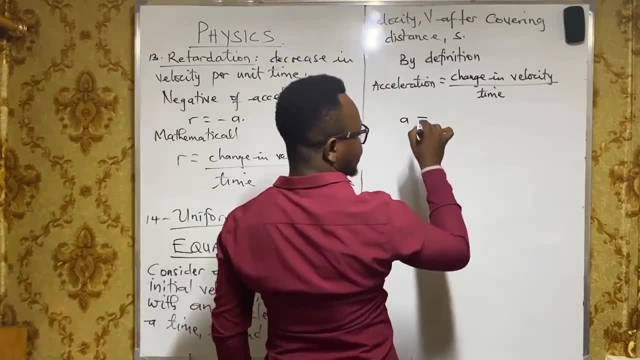 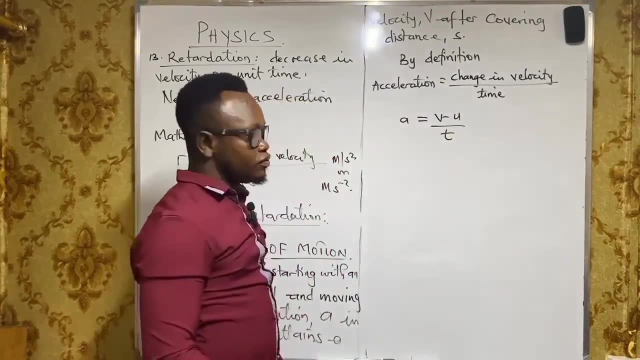 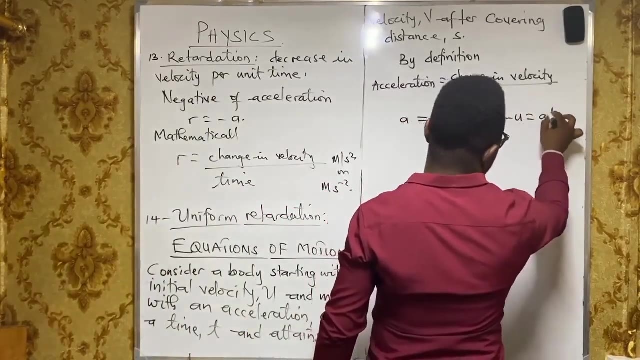 over-the-clock verstehen a and changing velocity as the final velocity minus the initial velocity expressed over the time. so we can cross multiply here and this implies we will get v minus u to be equal to 80. so we can say here v is equal to u. for transpose this becomes 80. 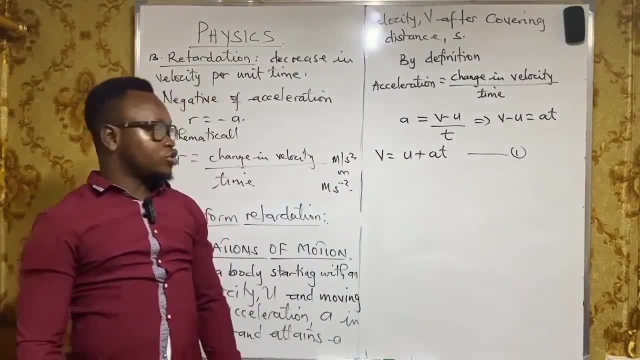 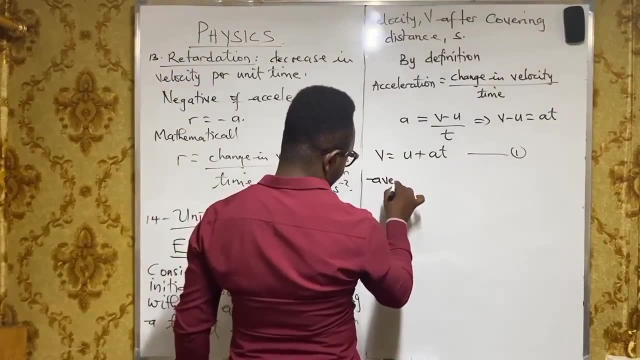 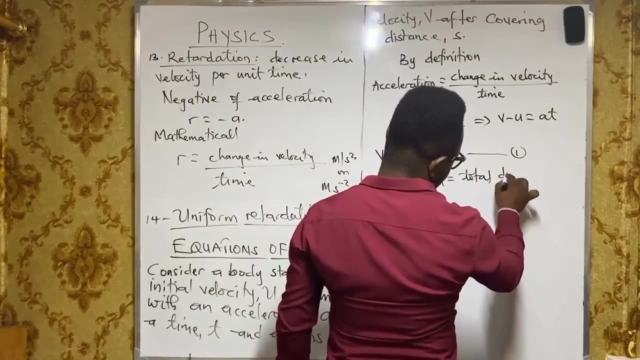 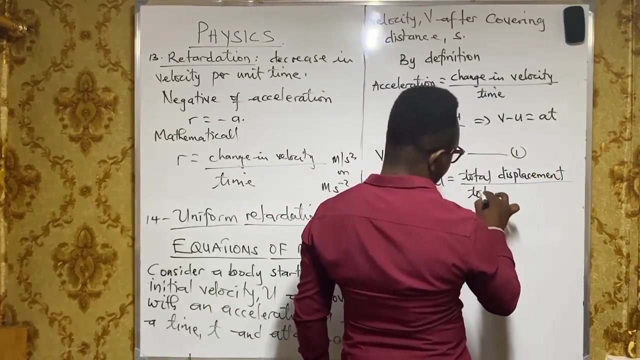 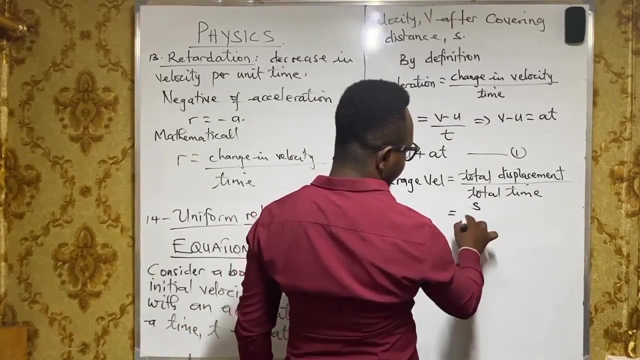 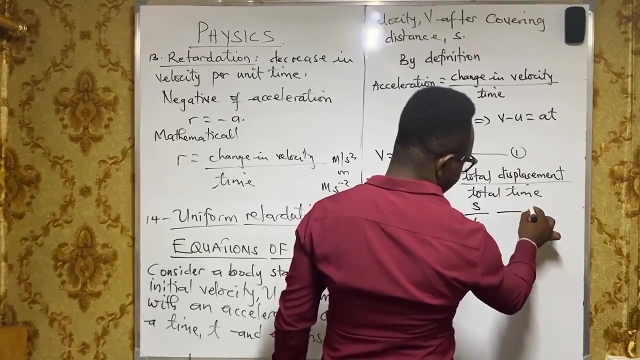 so this becomes our first equation of motion. that v is equal to u plus 80, okay, and we also know that average velocity is total displacement upon total time. so average velocity here is equal to u plus 80 is equal to u plus 80 is equal to total displacement s upon total time. so this we can refer to it as a. let's call this a. 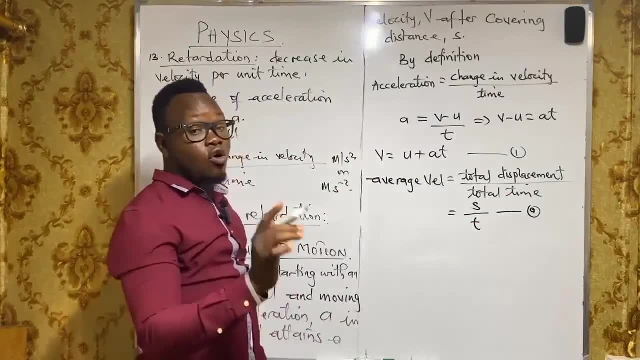 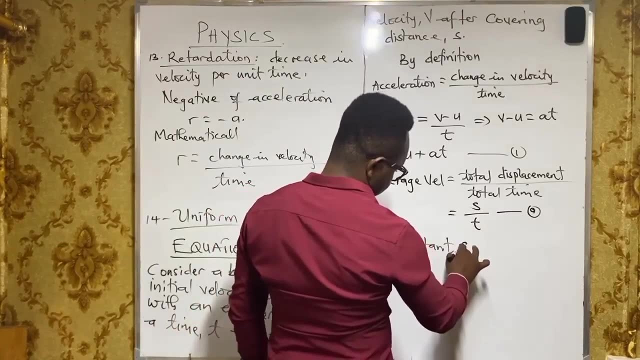 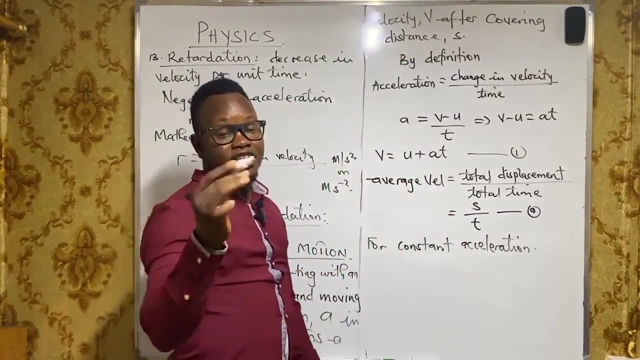 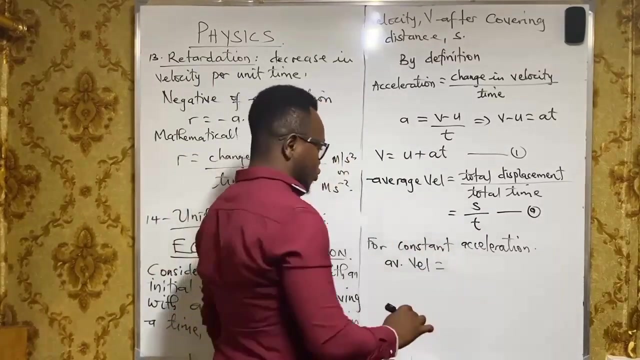 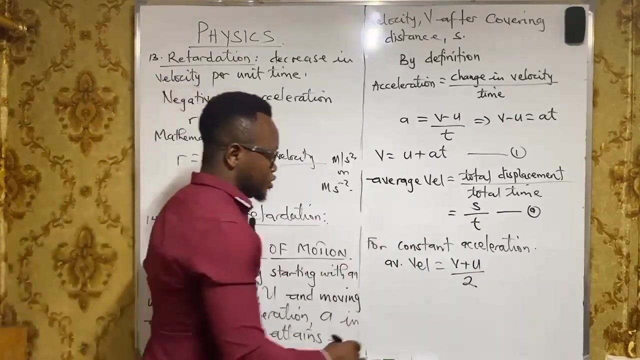 and we know, if a body is moving with a constant acceleration, so we say: for constant acceleration, if the acceleration is constant, the average speed or the average velocity is equal to, will be v plus u upon 2. so we say here thus: so we can refer to this as b, meaning average velocity is v upon u. 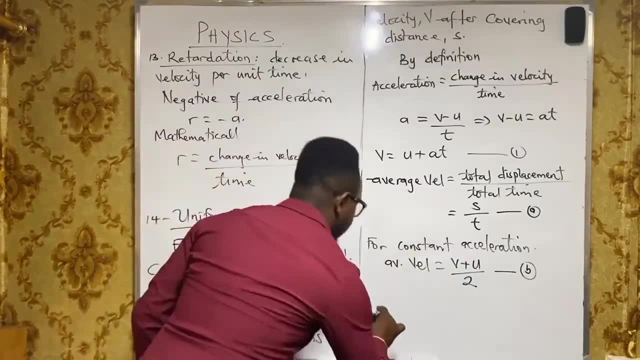 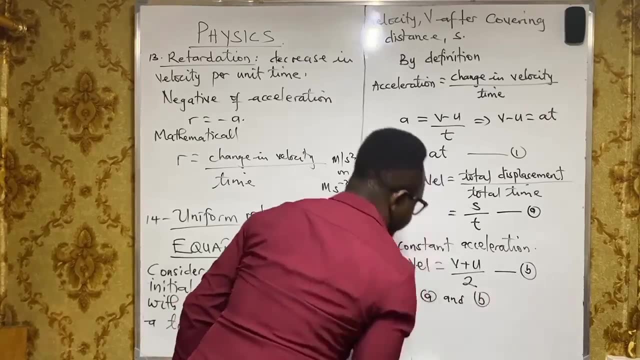 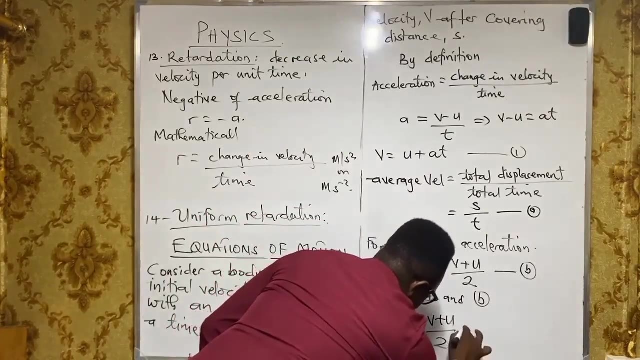 but if you look here, a and b are equal, so we can equate. equate a and b. so we'll now have: s upon t is equal to v plus u upon 2.. This implies, if we multiply here, we'll have s is equal. 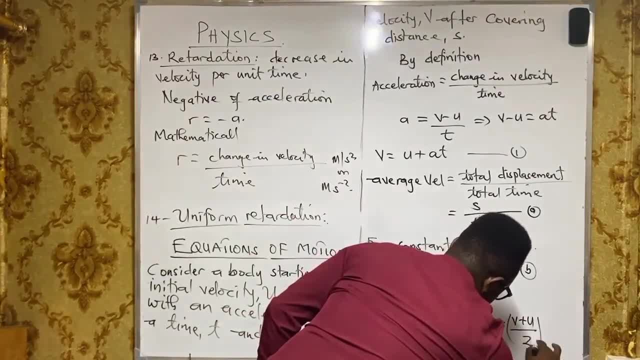 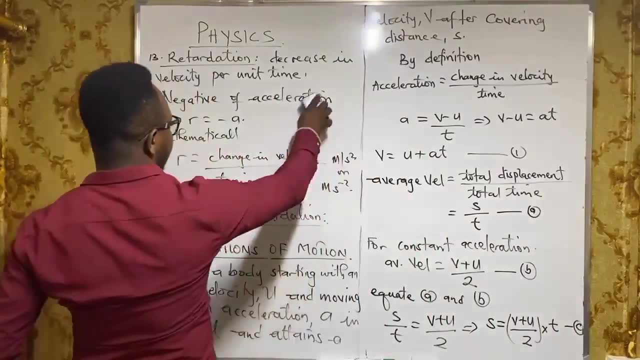 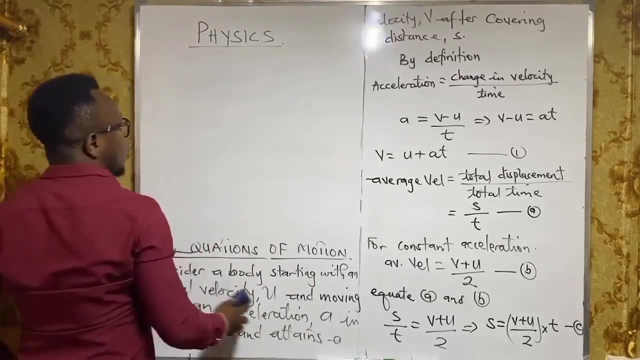 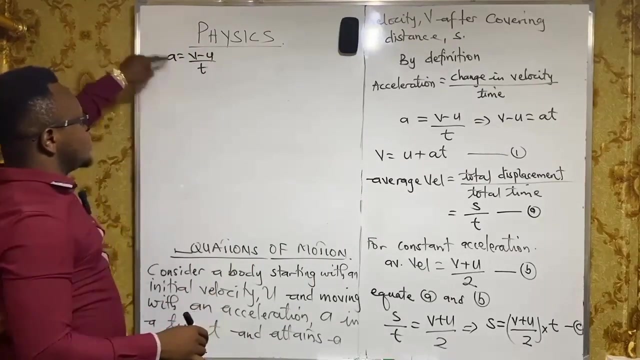 to v plus u upon 2, and then we multiply here by t, So this we can refer to it as our c From the definition of acceleration. acceleration is the changing velocity upon time. So from this a is equal to v minus u upon t. We can make t the subject. So making t the subject, we get t is equal. 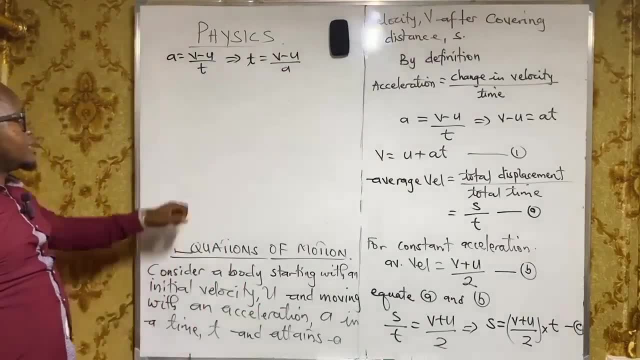 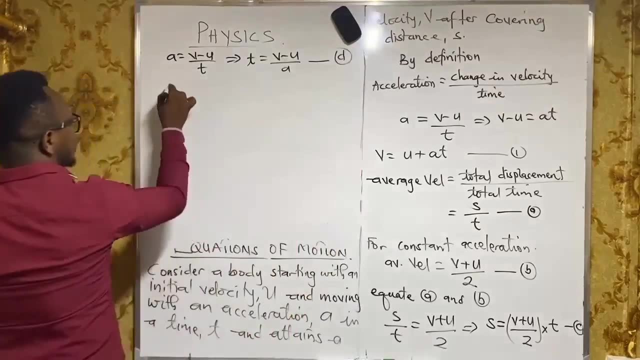 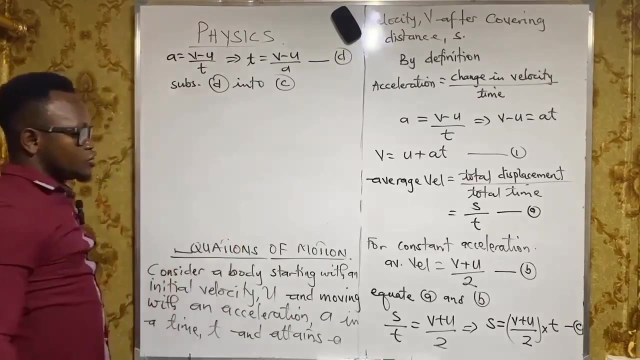 v minus u upon a. So we get here. t is equal to v minus u upon a, So we can refer to this as our d. So now, what we do, We can Substitute d into c. Substituting d into c, we'll have. s is equal to v plus u upon 2,. 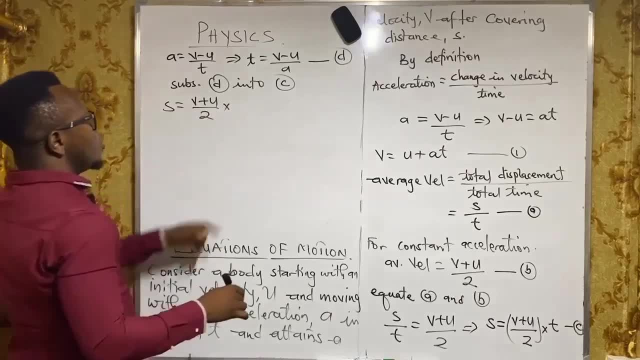 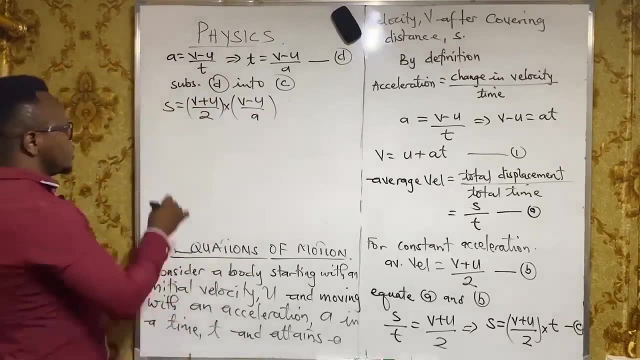 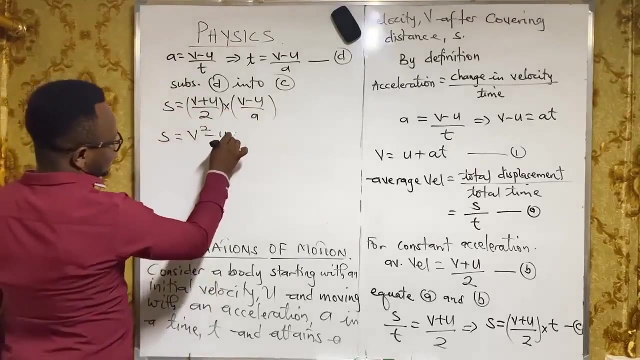 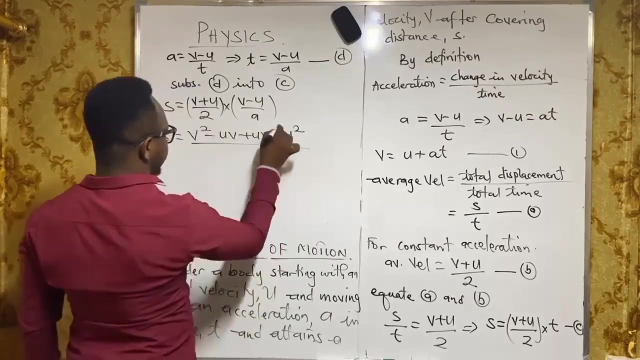 v plus u upon 2, multiplied by v minus u upon a, So if we work this one out, s will be equal to. this- will give us v squared, and this, multiplied by this, will give us minus uv, and this will give us plus uv, and then we'll get minus u squared, all expressed over 2a. 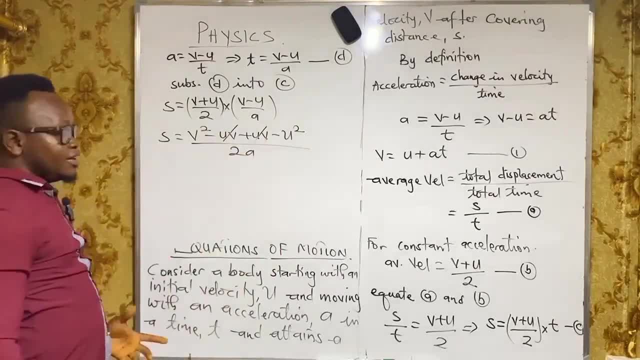 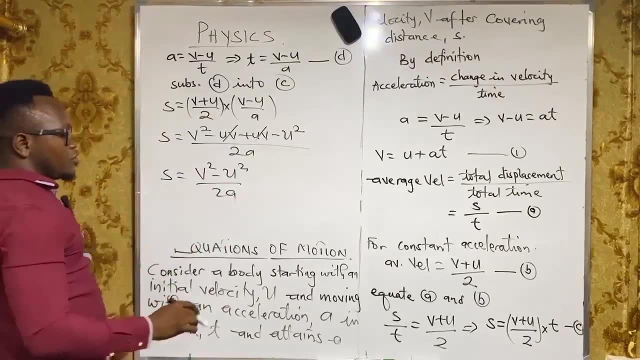 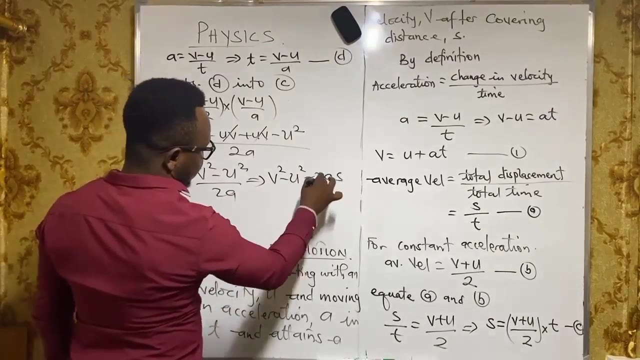 So this guy and this guy will cancel, because plus uv, minus uv, they cancel. So s will be equal to v squared minus u squared upon 2a. So if we cross multiply, this implies we'll get v squared minus u. squared is equal to 2a multiplied by s And making v squared. 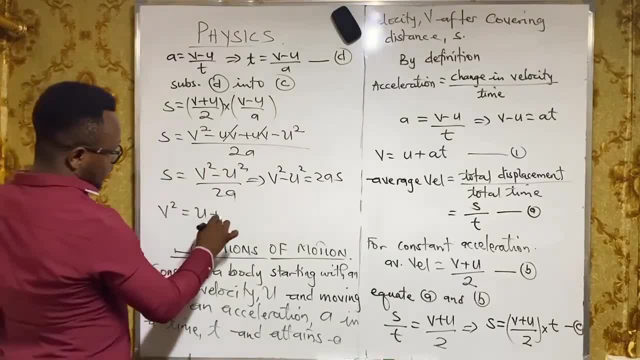 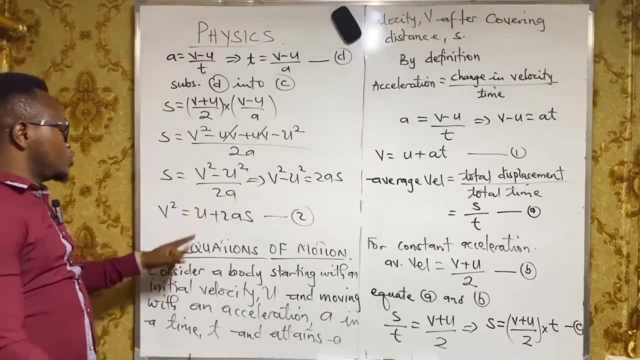 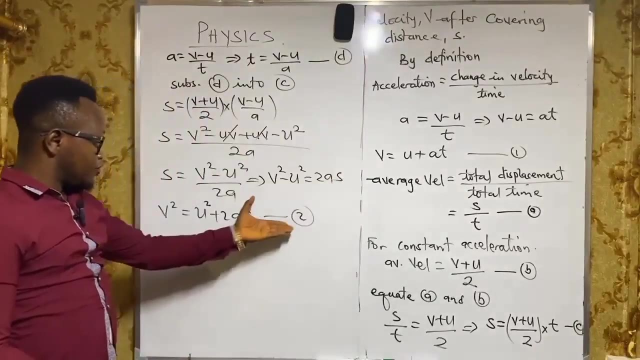 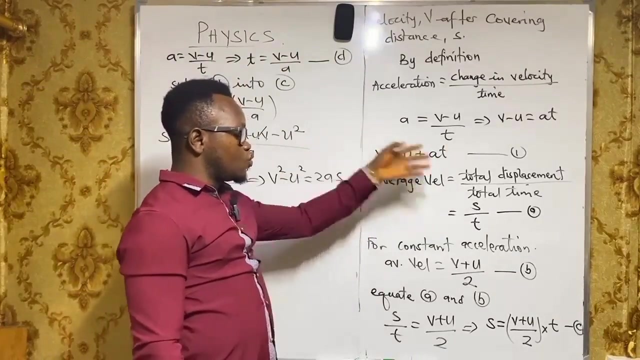 the subject. So v squared will be equal to u squared plus 2a s. This becomes our second equation of motion. So v squared is equal to u squared plus 2a s. So now we've gotten equation 2.. So if you look at equation 1, v is equal to u plus 80.. If we substitute equation 1 into c, 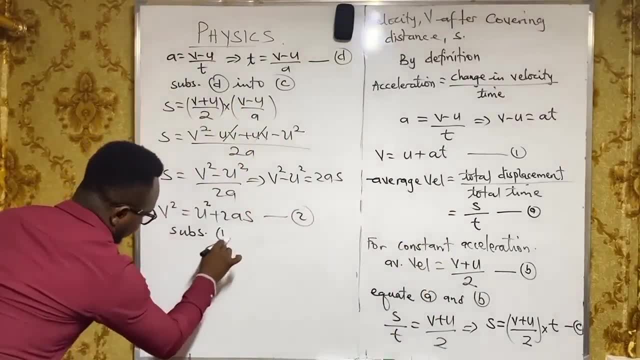 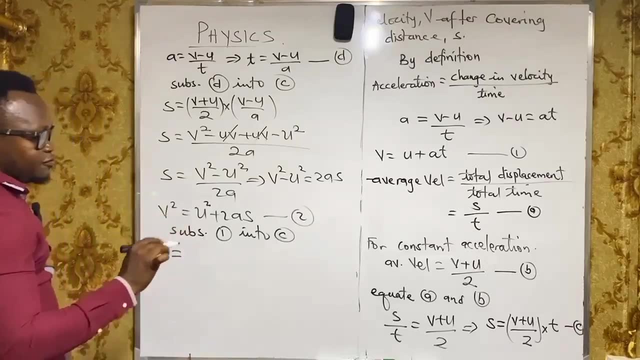 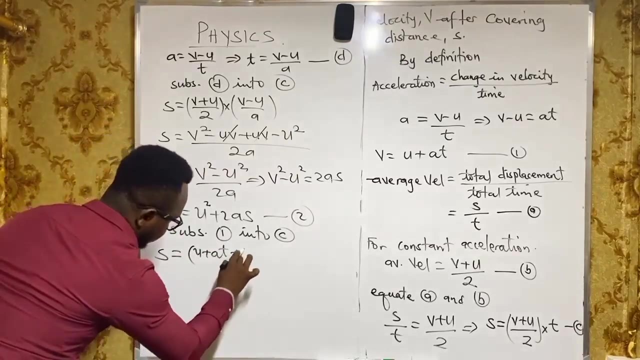 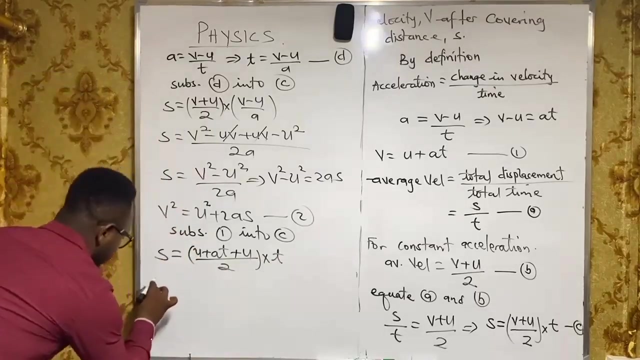 so substitute 1 into c and it becomes c is s is equal to v plus u upon 2.. So where we see v, we put u plus 80, and then plus u upon 2 multiplied by t. So this means s will be equal to. 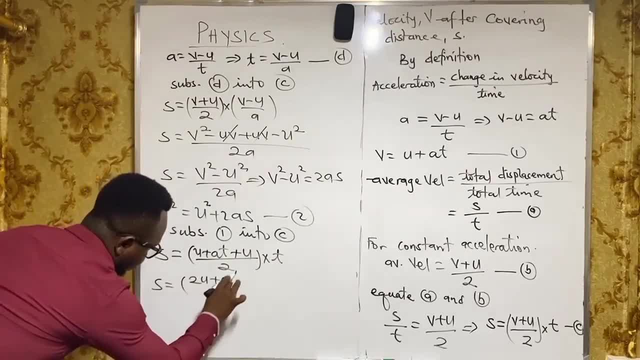 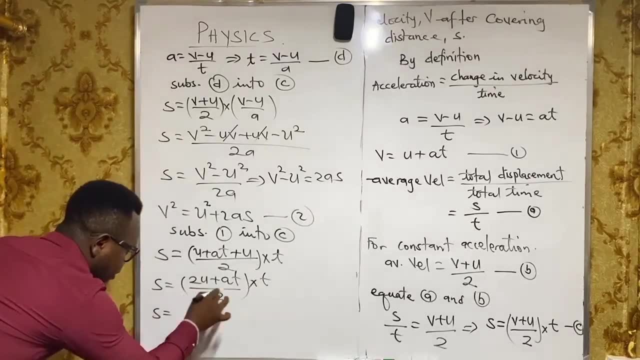 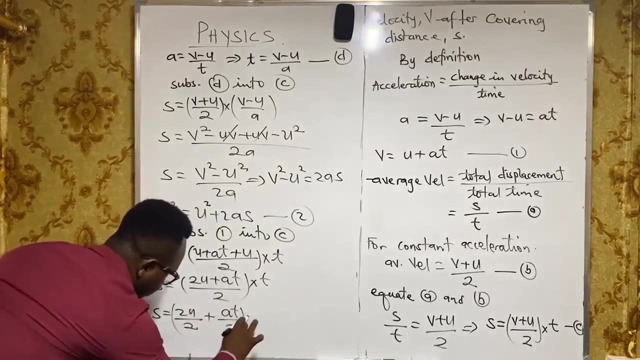 in this bracket. we get here 2u plus 80, all divided by 2 multiplied by t. So this implies s is equal to. we can split this one up into 2u upon 2 plus 80 upon 2 multiplied by t. here 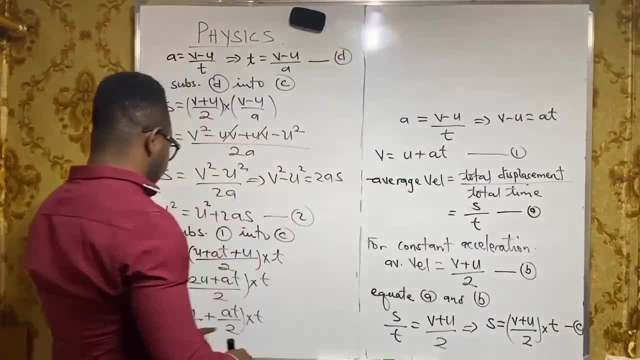 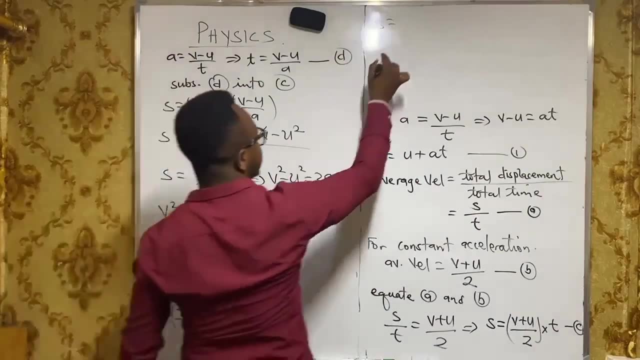 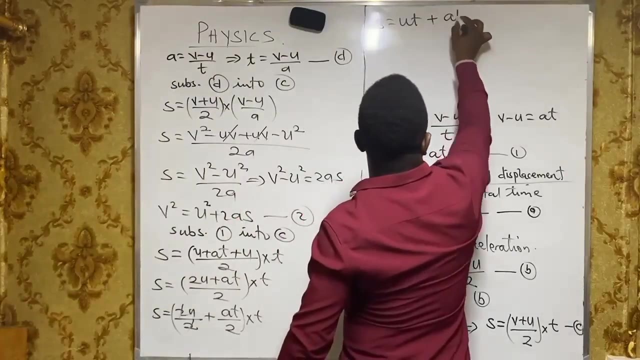 So we'll now have, so we will now have here. this will multiply. We get: s is equal to these two and these two cancels u multiplied by t. We get ut plus 80 multiplied by t gives us 80 squared. 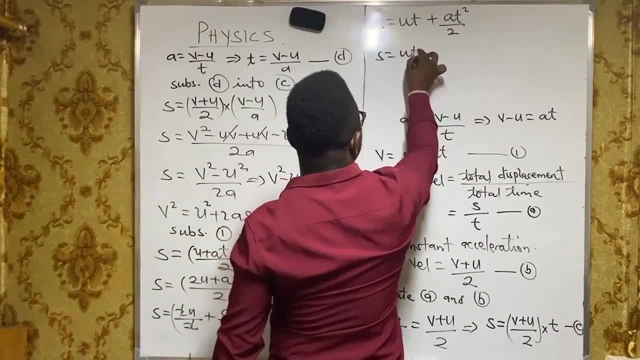 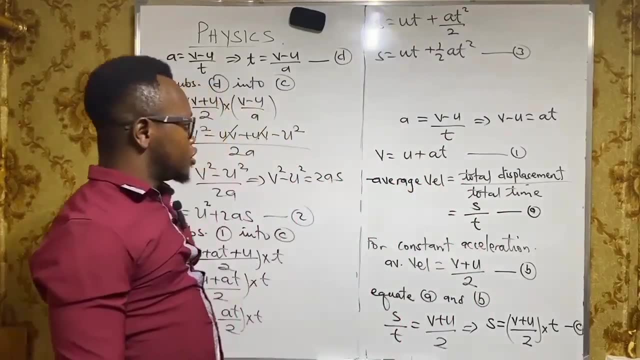 So we have it to be: s is equal to ut upon 2 is the same as half 80 squared. So this gives us our third equation. So these are the three equations of motion, So the equations. we can summarize them now to be this: 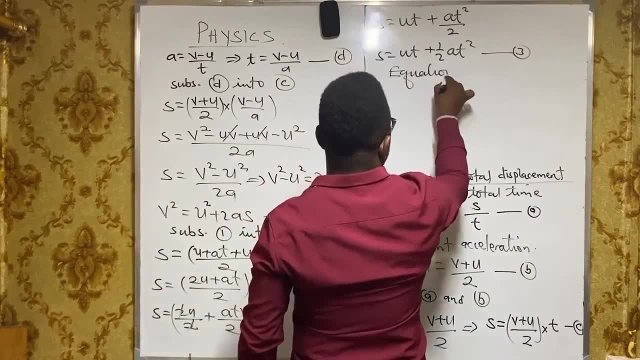 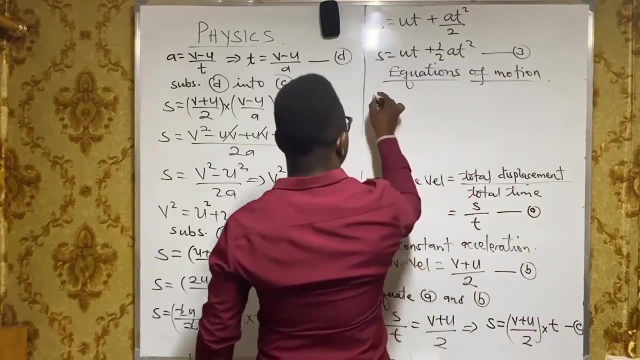 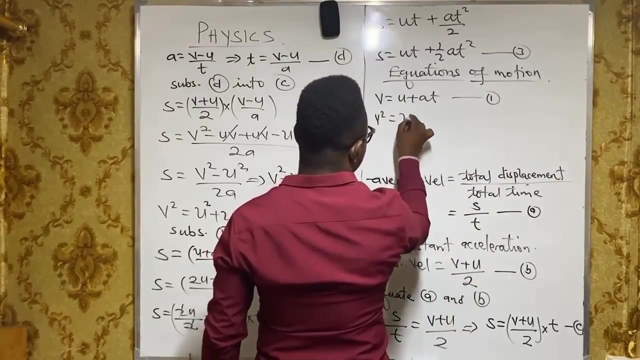 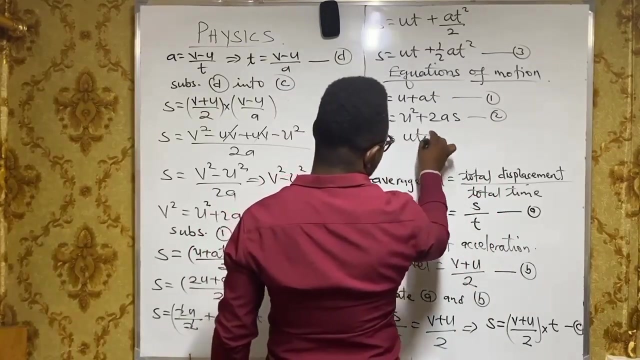 that the equations of motion are are: v is equal to u plus 80, equation one: v squared is equal to u squared plus 2as equation two. and s is equal to ut plus half 80 squared equation three. So these are the three equations of 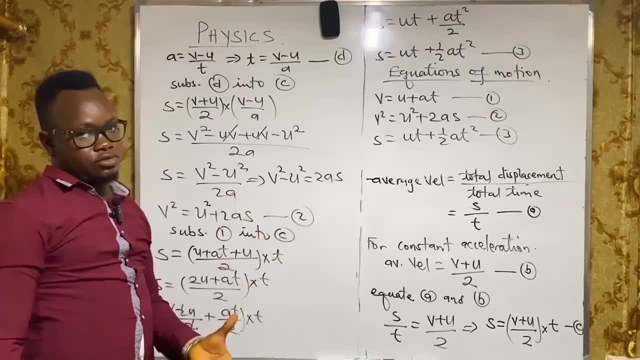 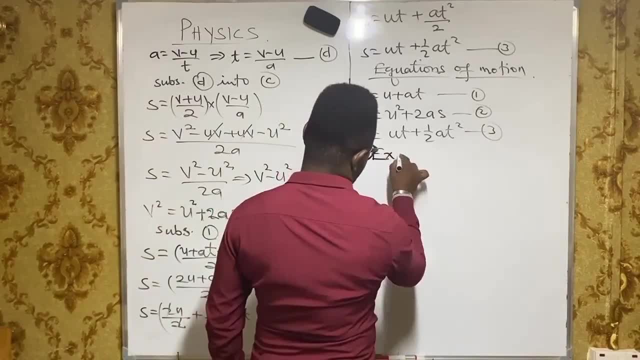 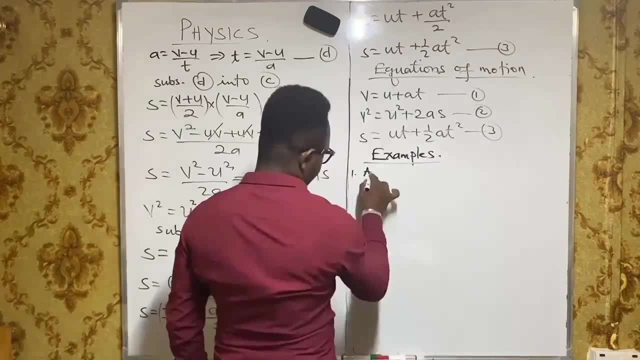 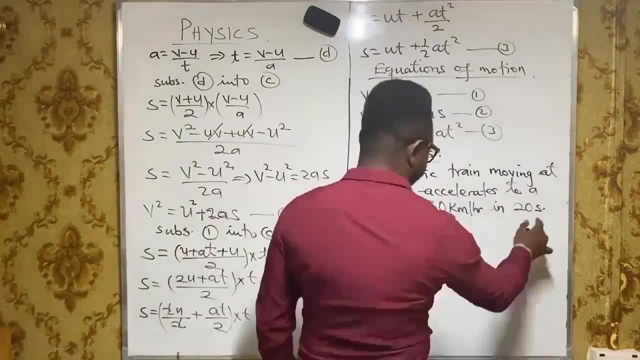 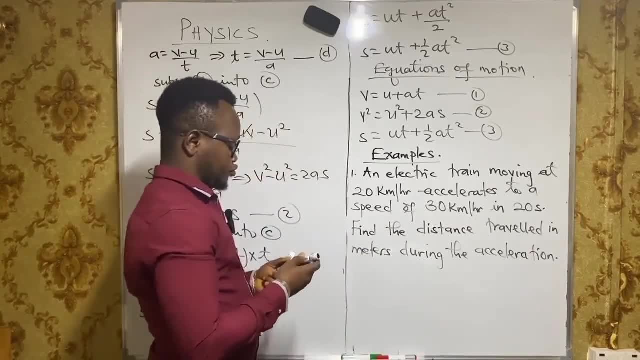 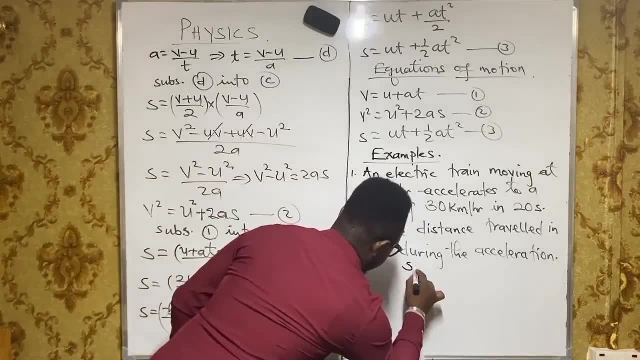 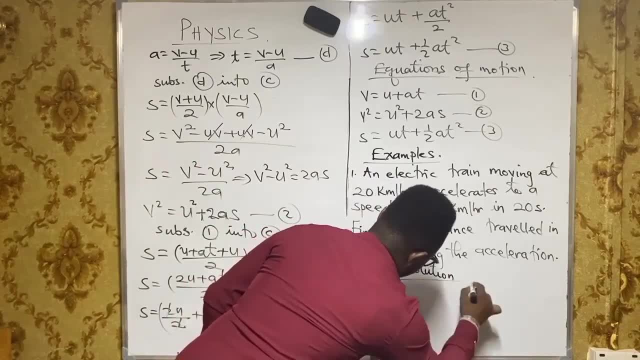 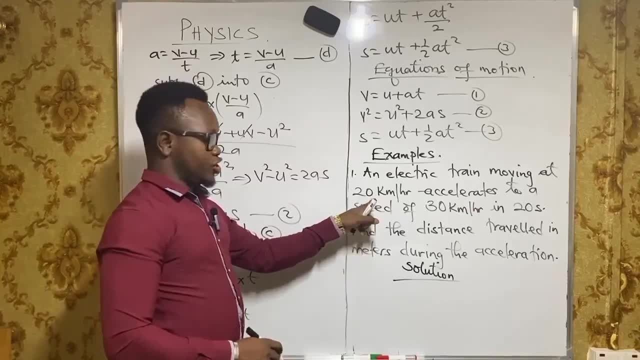 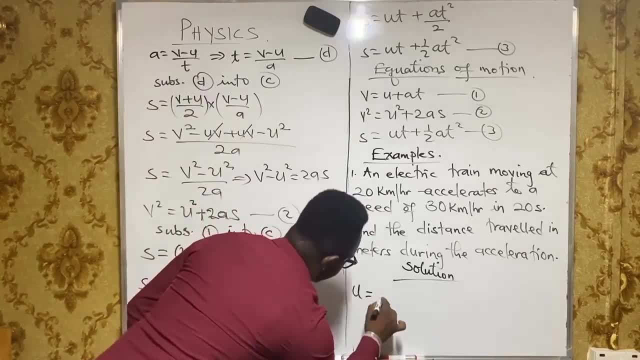 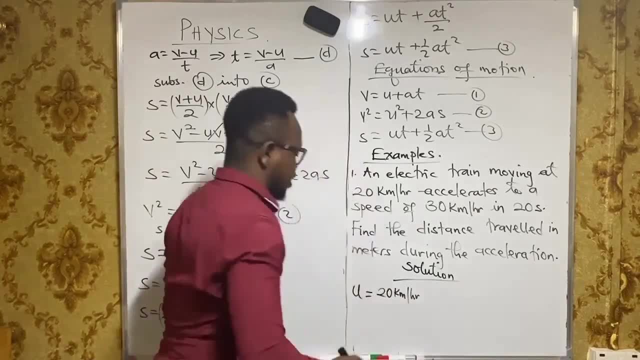 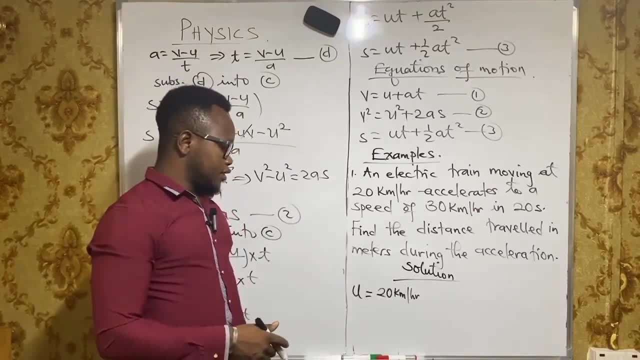 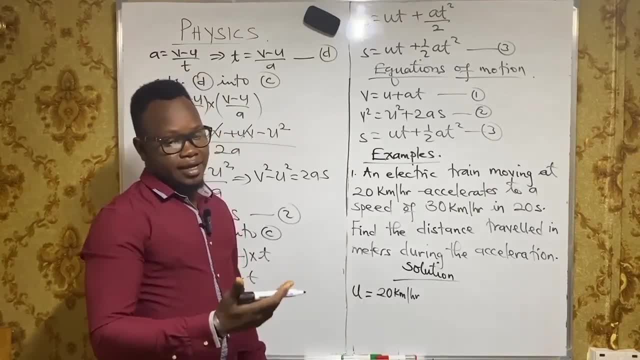 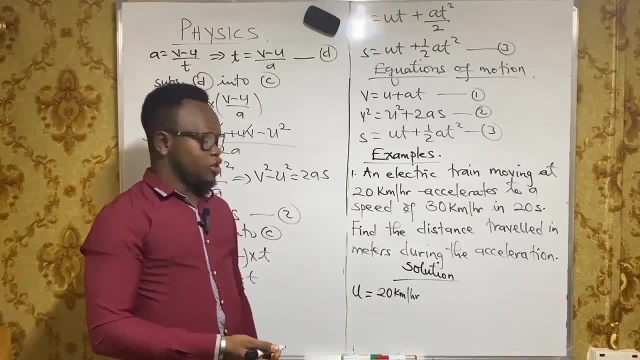 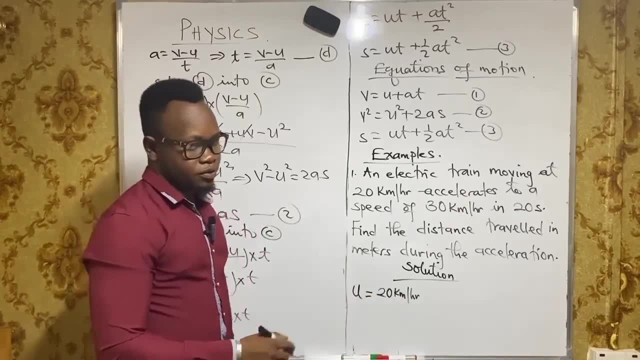 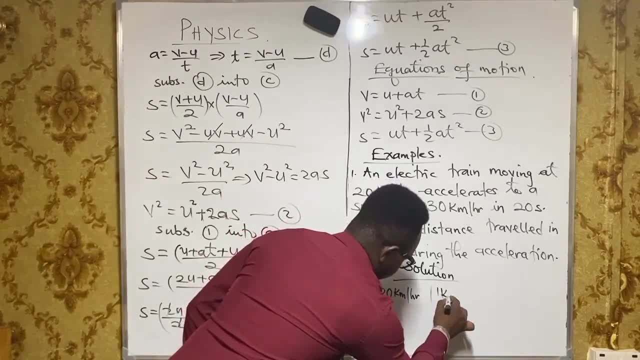 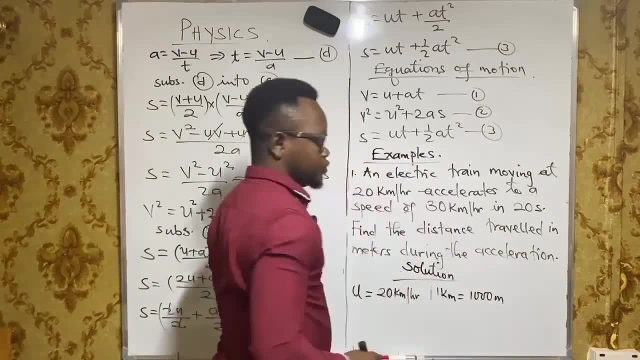 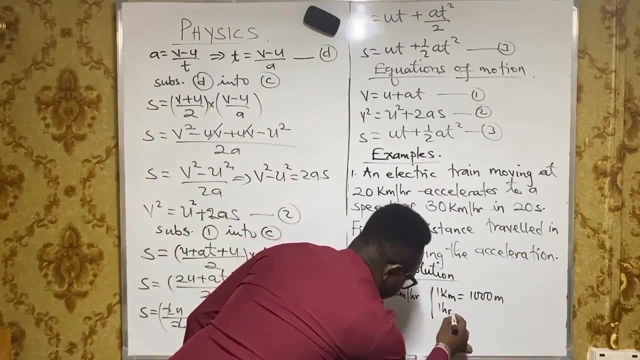 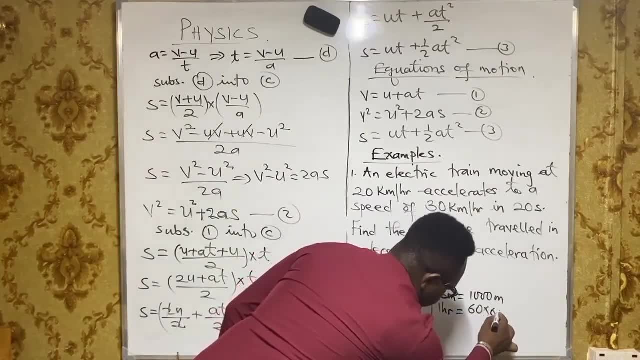 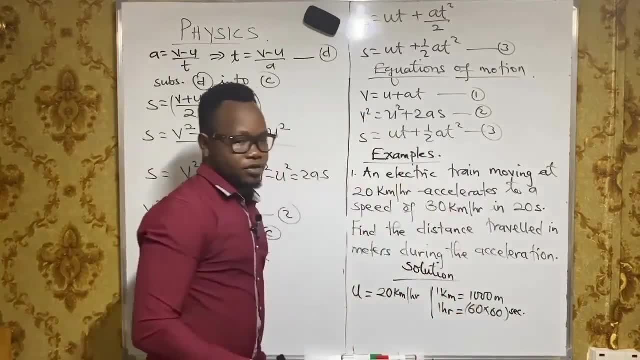 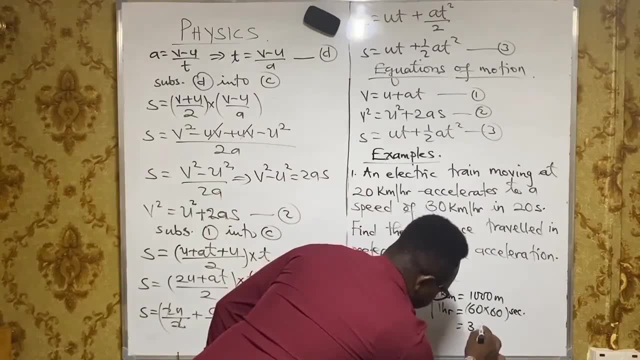 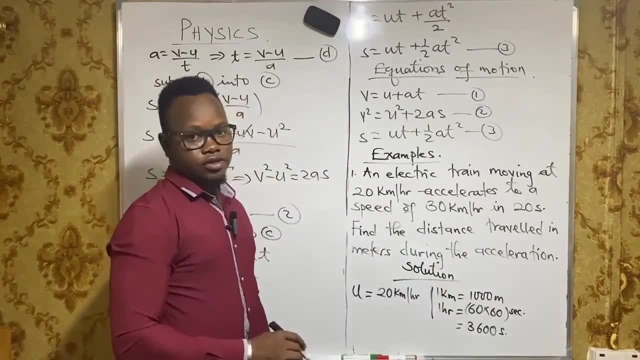 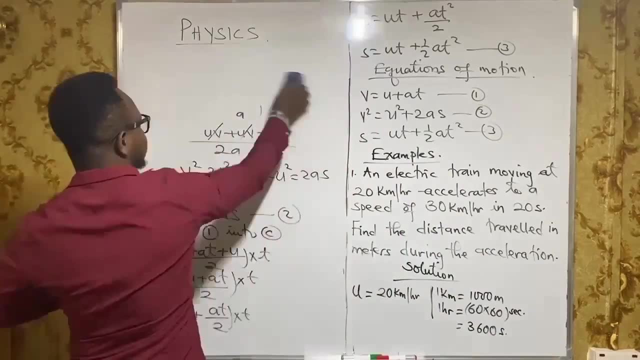 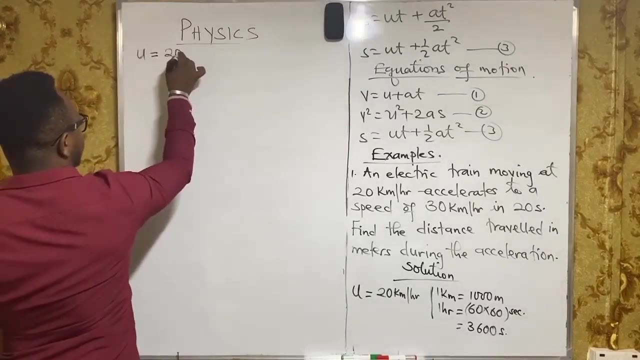 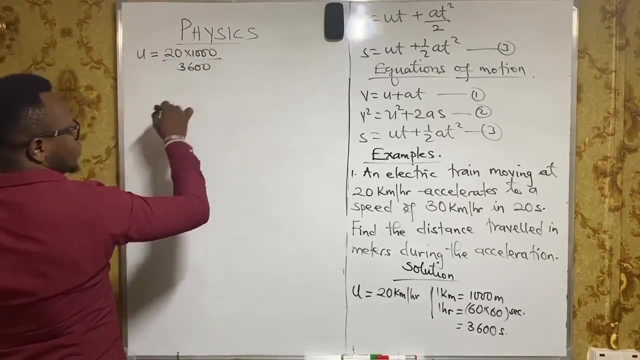 we have a equation of motion. we have a equation of motion, thousand six hundred seconds. so for us to convert this now to meters per second, it is now going to be that u equal to 20 multiplied by 1000, divided by 3600. okay, so this, this cancel this, and this cancels. 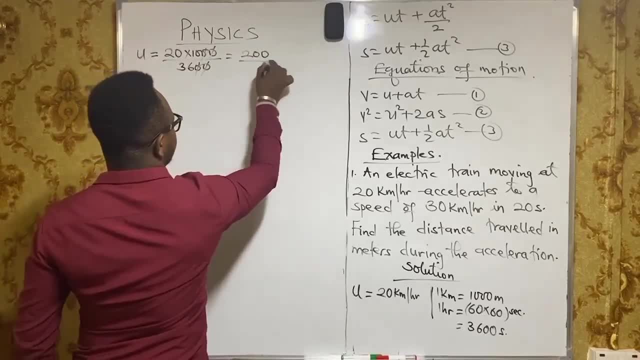 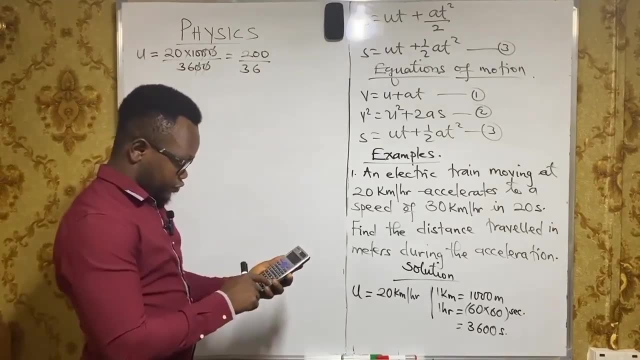 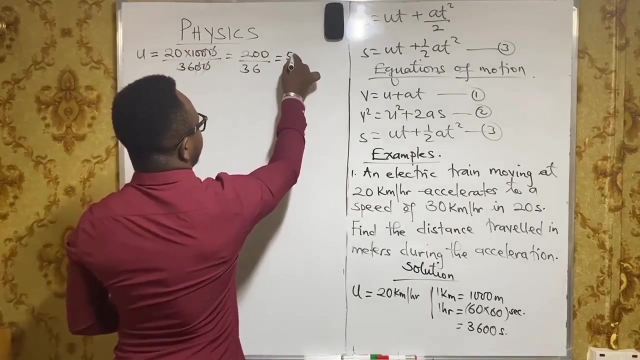 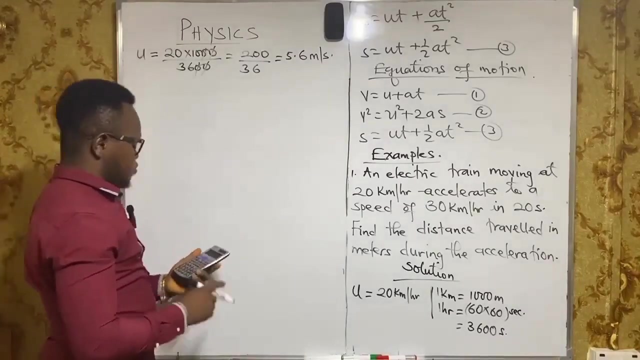 so you are left to it. 200 divided by 36 go for a calculator. so 200 divided by 36 gives us 5.55, so we can write this as 5.6 meters per second. okay, so this becomes the initial velocity. next we look at: 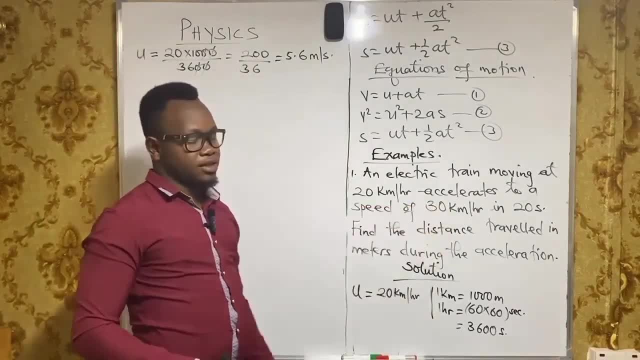 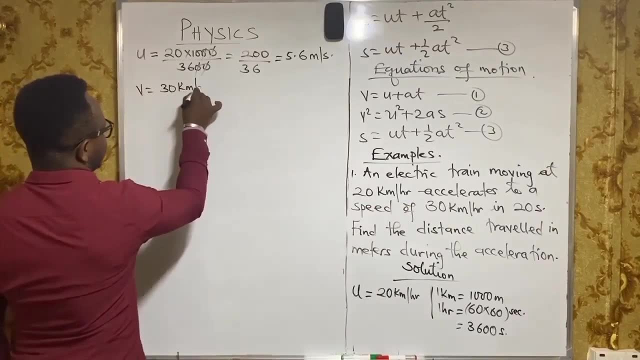 one say it accelerates to a speed of 30 kilometers per hour. so that's the final velocity. v is 30 kilometers per hour. so with this we can now say here: this is 30 multiplied by a thousand, divided by 3600, and it will now be in meters per second. so this zero and zero cancels this. 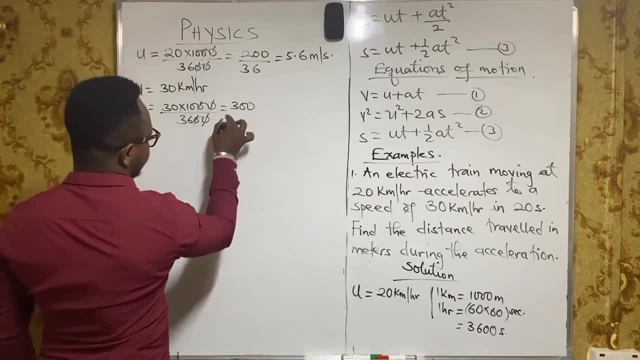 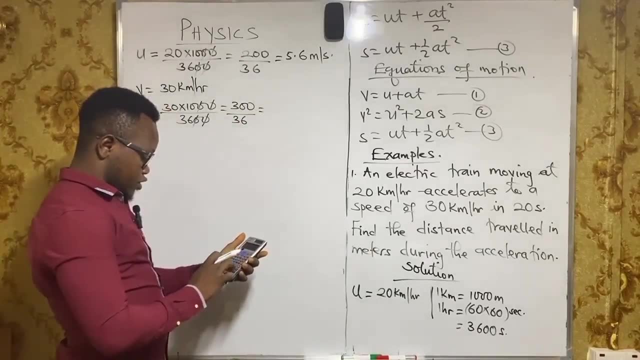 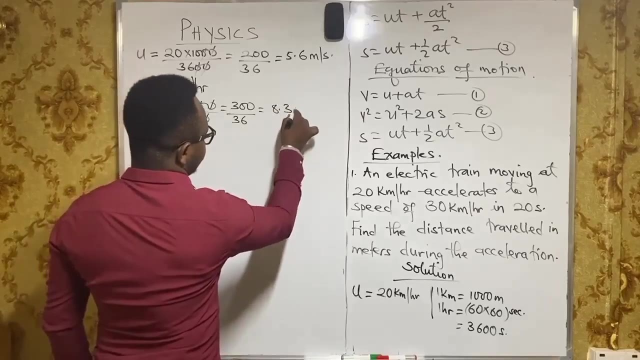 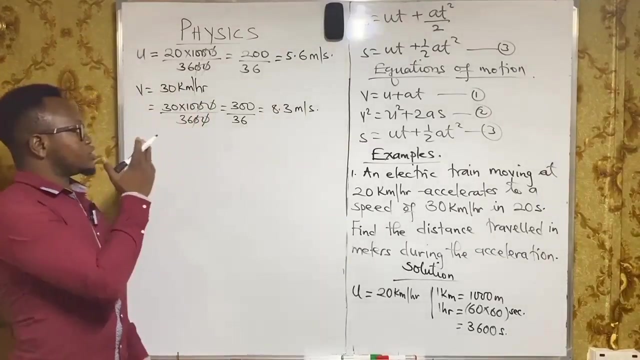 and this cancels. so you are left with 300 divided by 36, and 300 divided by 36 will give us 300 divided by 36, we get 8.33, so that is 8.3 meters per second. so now we've done our conversions. the u, which is the initial. 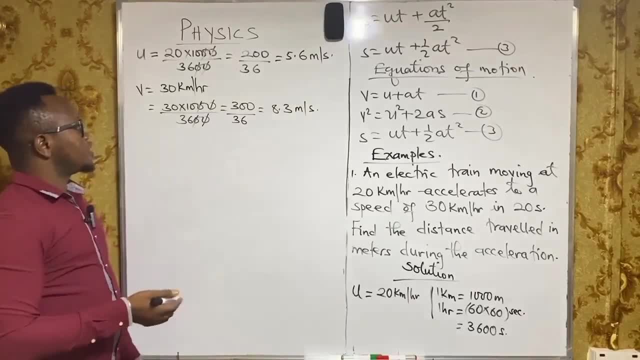 velocity have been converted to meters per second, and the v, which is the final velocity, have been converted to meters per second. so now the question is asking us to find the distance travel. but we can't calculate the distance if we don't know the acceleration. and we know from the definition of the term acceleration: it is the time rate of. 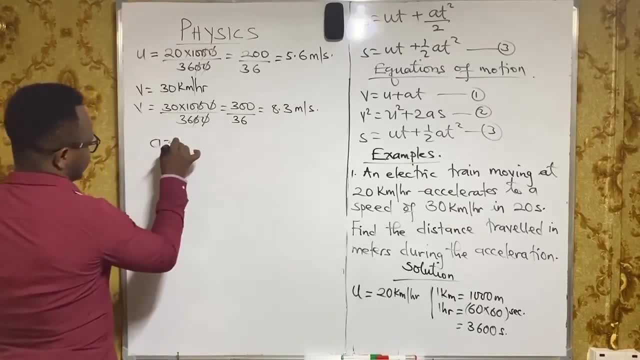 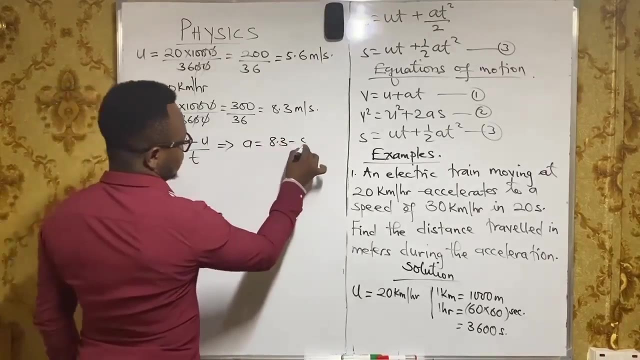 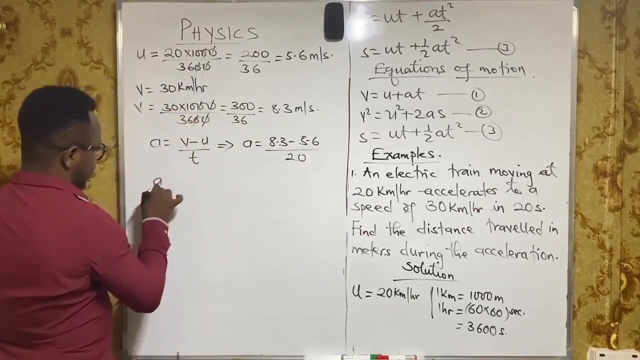 change of velocity, so meaning acceleration is equal to final velocity minus initial upon the time. okay, so this implies the acceleration a is equal to final velocity 8.3, initial velocity 5.6, divided by the time, that is, 20 seconds. so the acceleration will be equal to. 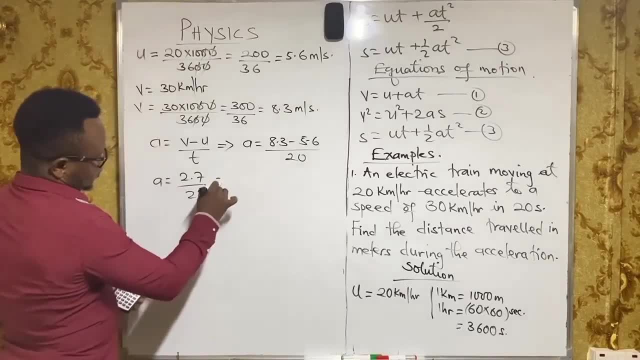 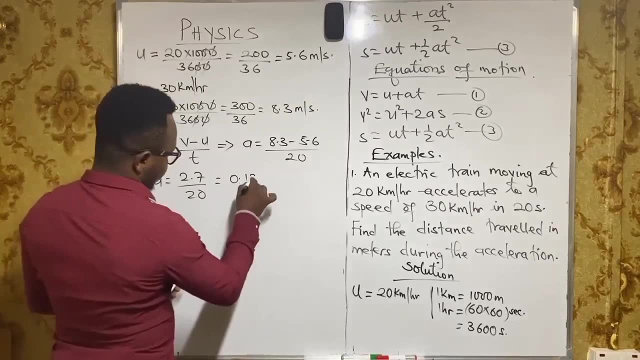 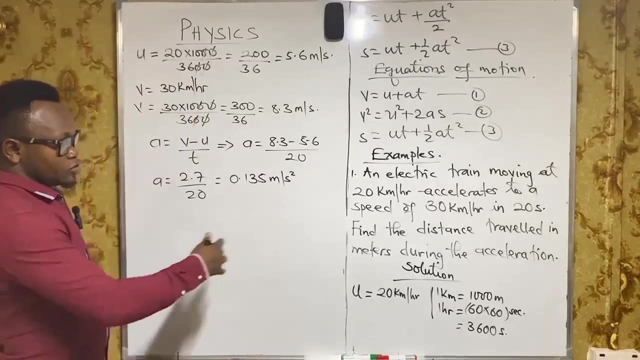 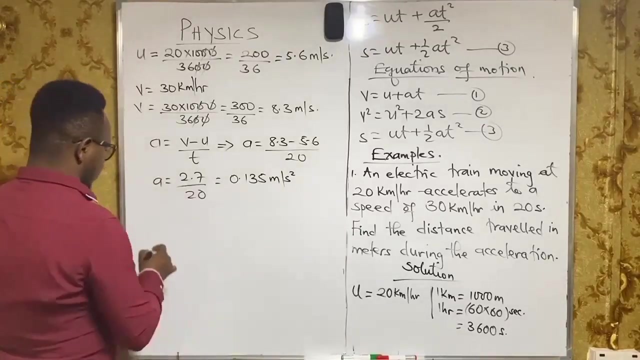 that gives us 2.7 divided by 20, that gives us 0.1, something divided by 20, so we get 0.135, and this is meters per second square. so that gives us our acceleration. so for us to find the distance covered. now it is up to us which of the equations of motion we will use. so 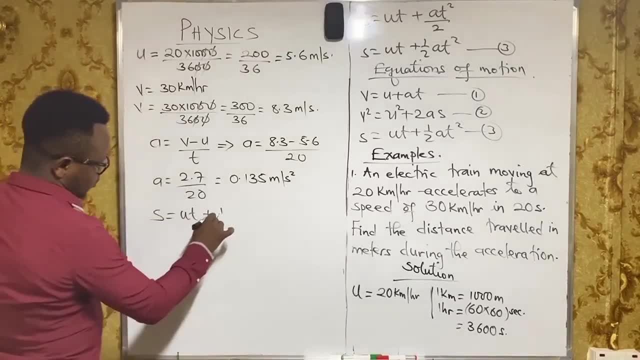 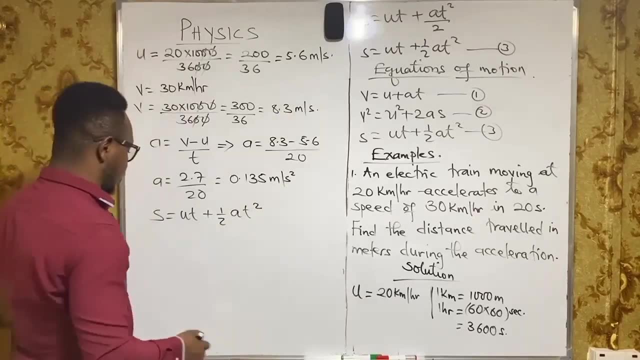 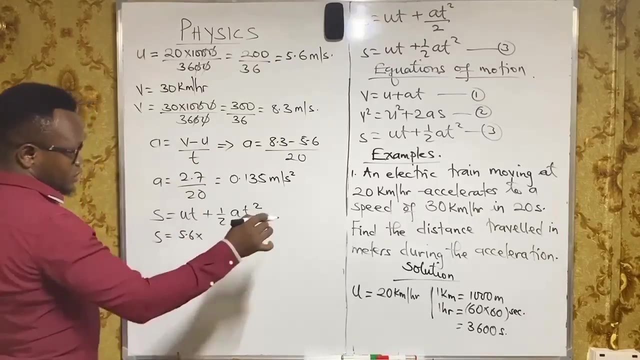 we can say here: s is equal to ut plus half a t squared. or you can use v square is equal to u square plus 2s. any one of the two. so s, which is the distance, is equal to the initial velocity. we have it as five point six, one square by the time it took to cover. it's 20 plus half multiplied by the acceleration. the acceleration is 1.5. they are 20, important here. and when u c summer is equal to u c plus is five and six. so we are seeing that how bunny is equal to u c plus us is光. you will use the two as one: a one times square v, square plus two s have multiplied by the ratio. all these did we've avaient. 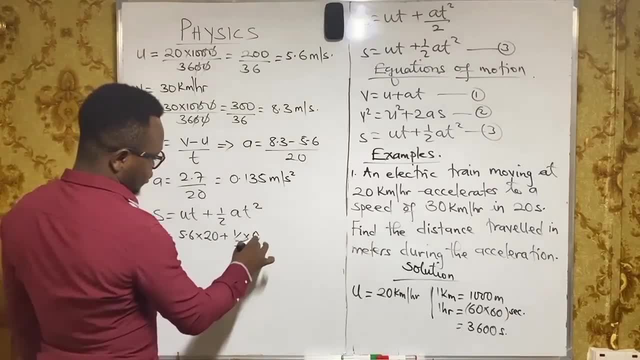 is equal to u squared plus 2a LไปisuOs. we have chosen the initial velocity, five point six multiply by the time it took to cover is 20 plus 1.5. the opening speed, the acceleration, have been calculated as 0.135 multiplied by times square, that is, 20 squared. 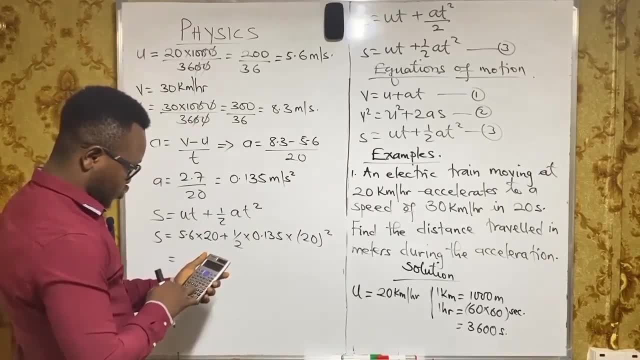 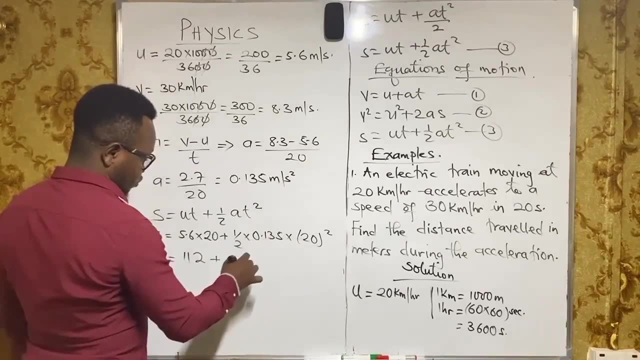 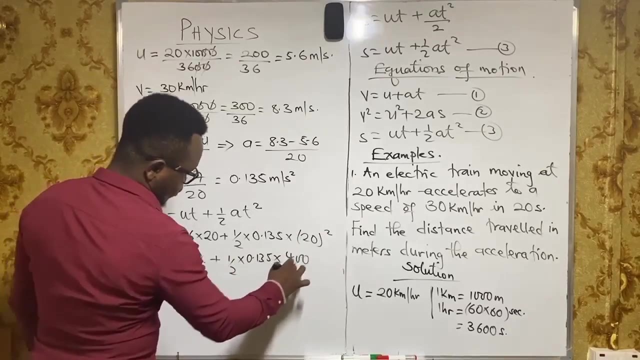 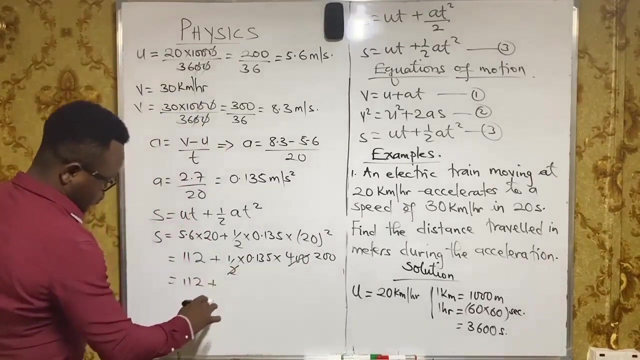 so 5.6 by 20, this gives us 112, so we have 112 plus. and then this becomes one upon two. multiplied by 0.135, 20 squared is 400. to integrate surface 1 into 400, here is 200 times, so we have 112 added. 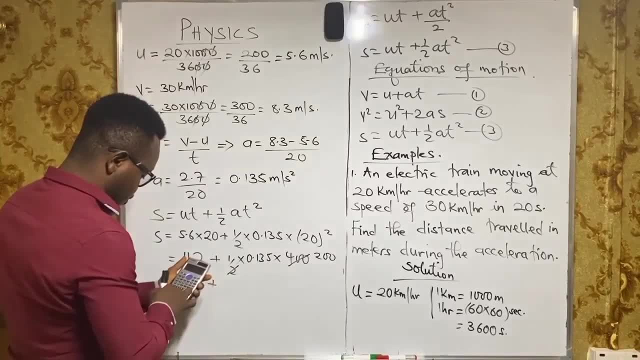 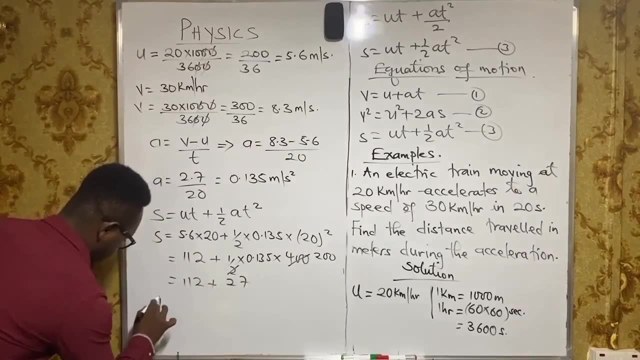 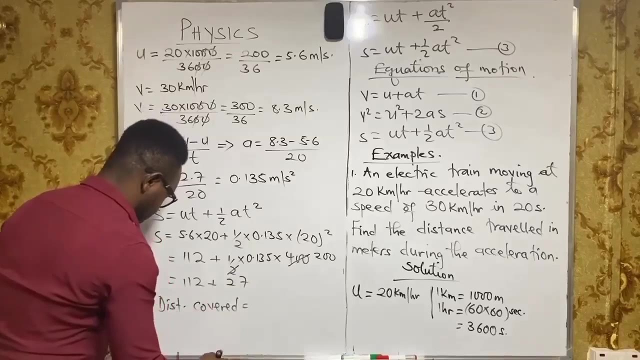 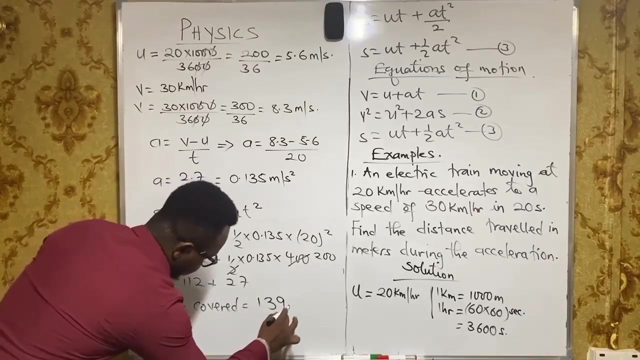 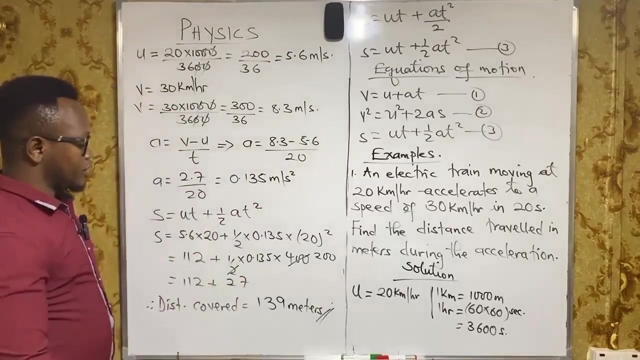 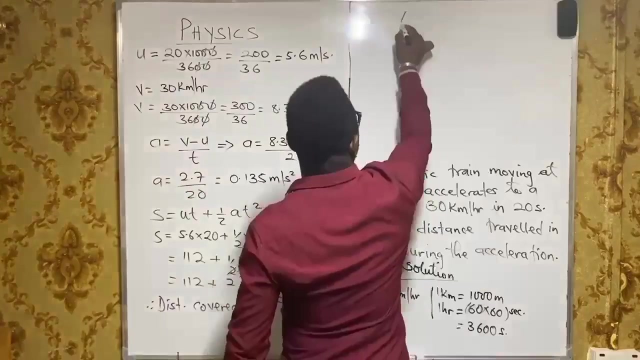 to this: multiplied by 200- 0.135 multiplied by 200, we get 27. therefore, the distance covered during the acceleration is equal to. you get 139 meters. so this is the distance that's the train covered within this. if you don't want to use this equation here, you can use an alternative method, and that is. 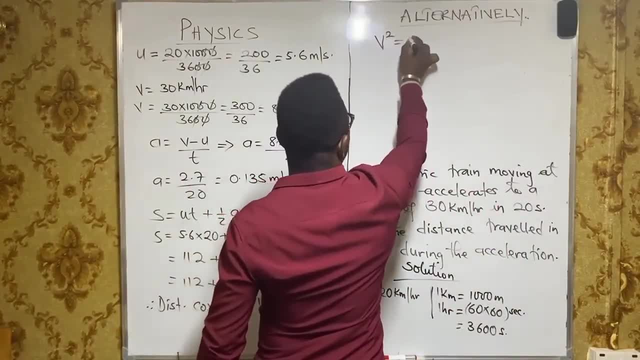 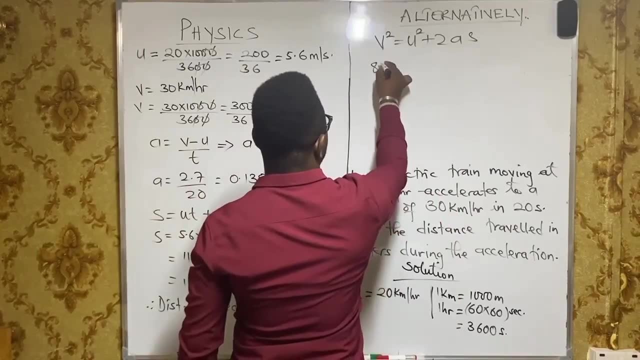 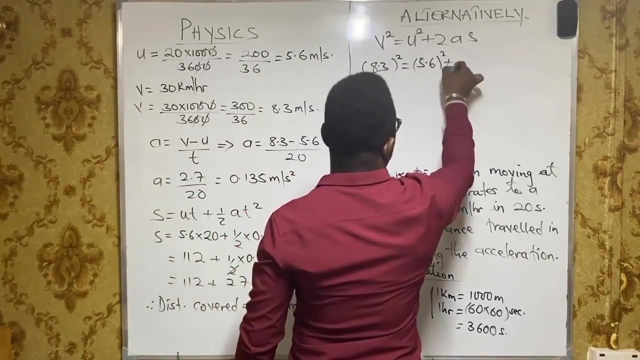 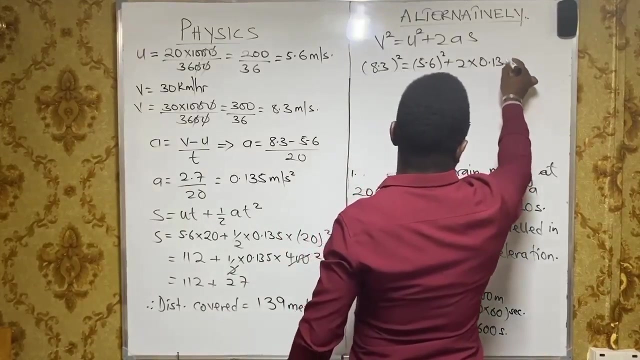 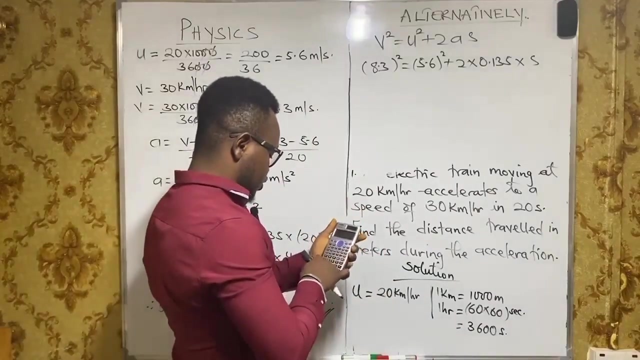 alternatively, you can use: v squared is equal to u squared plus two. a s v 8.3 does. 8.3 squared is equal to u 5.6 squared plus two multiplied by the acceleration. we've calculated. we have it to be 0.135 multiplied by the distance: s. so 8.3 squared. 8.3 squared will. 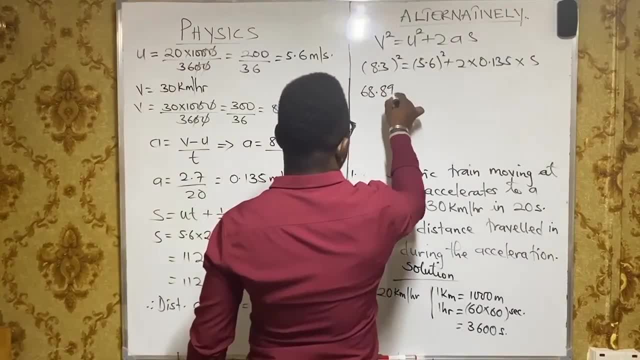 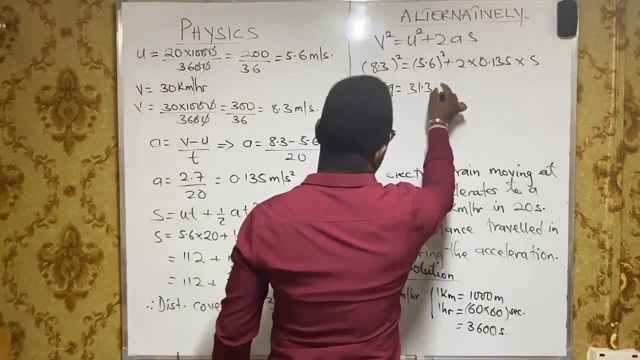 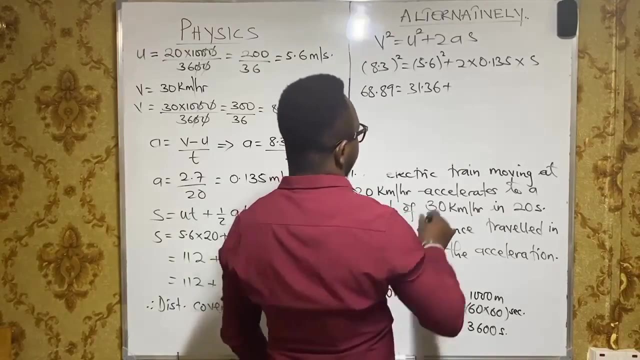 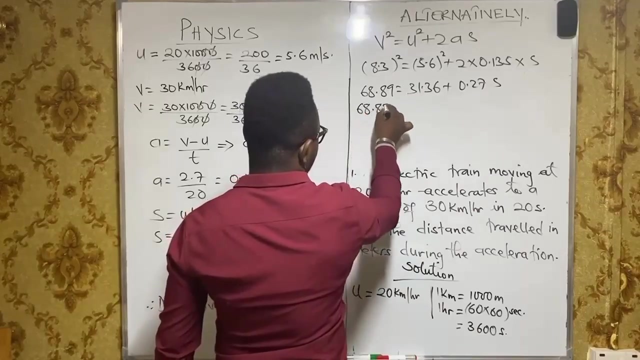 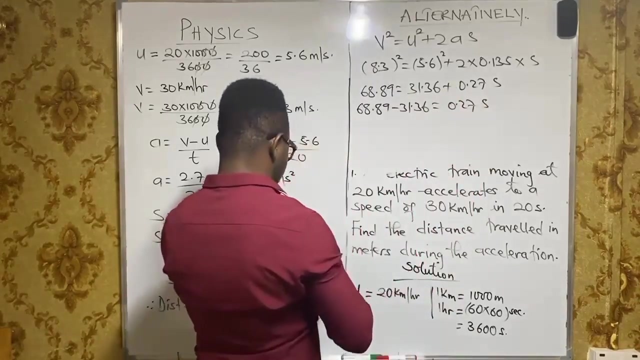 give us 68.89.. and 5.6 squared will give us 31.36. plus 2 multiplied by 0.135, that gives us 0.27. so we can transpose this: 68.89 minus 31.36 will give us 0.27 s. so if we do this subtraction here, 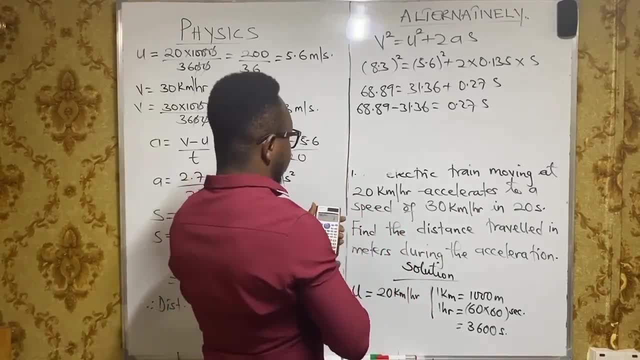 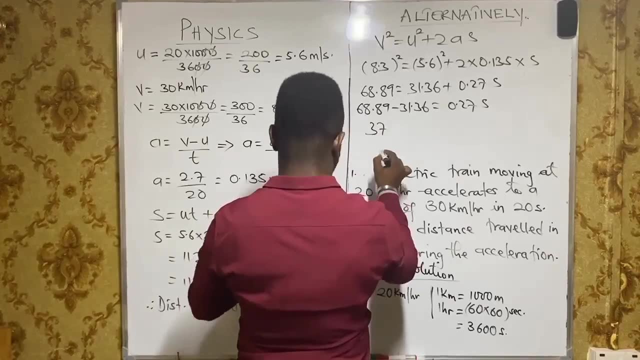 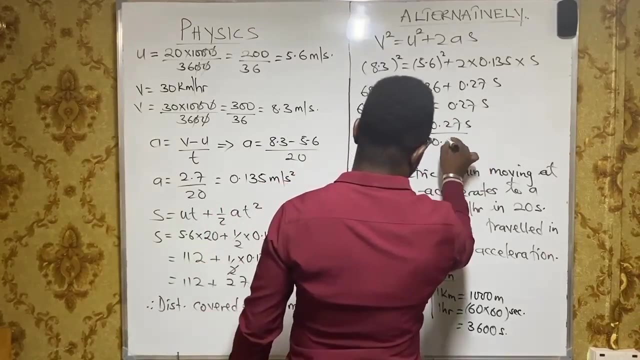 68.89 minus 31.36, this gives us 37.53 is equal to 0.27, the value of s that we want. we can divide here by 0.27, here by 0.27. so this guy and this guy cancels. 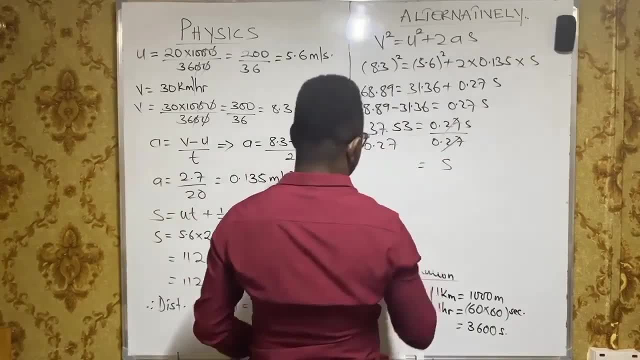 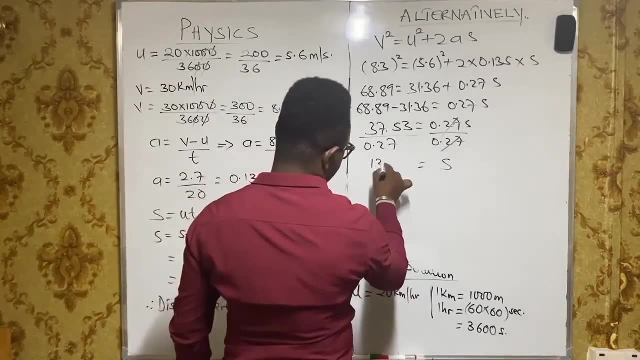 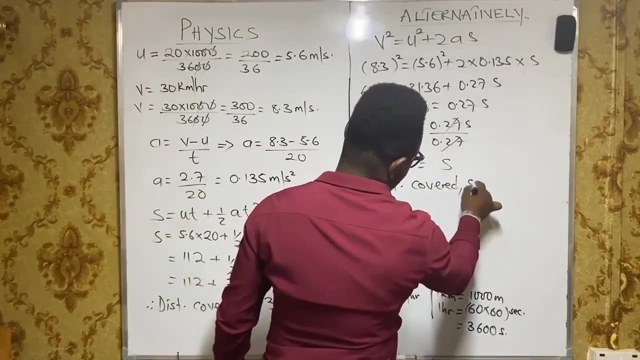 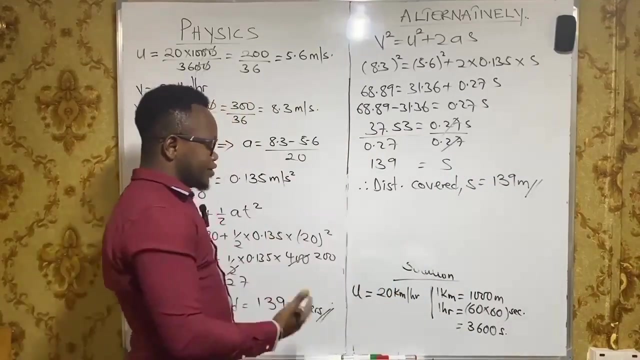 then s remains. so 37 divided by 0.27, 0.27 will give us 139. therefore, distance covered, which is s, is equal to 139. any of the two equations used, you arrive at the same answer. okay, let's look at another example. 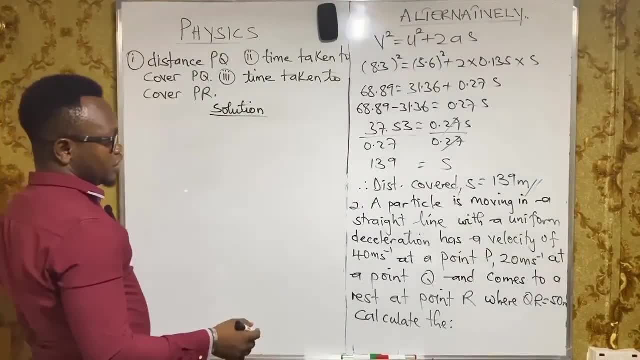 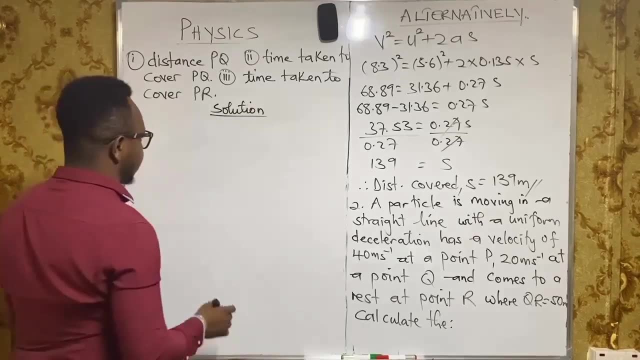 we are told that this particle is moving in a straight line. okay, with a uniform distance from the other particle. so we are told that this particle is moving in a straight line. acceleration has a velocity of 40 meters at a point p, so let's say it is starting at point. 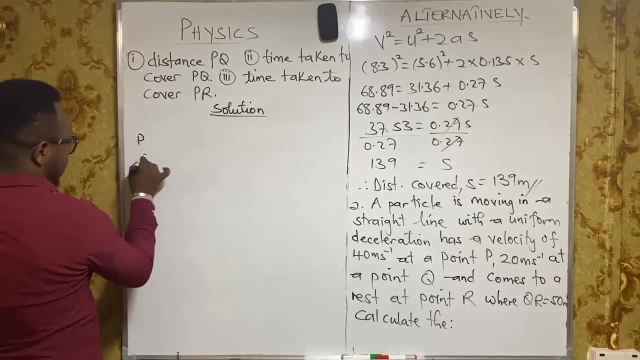 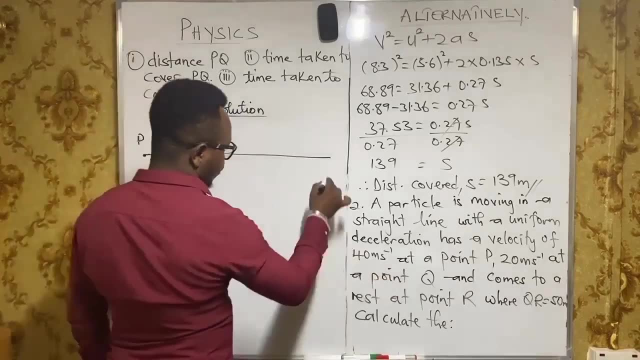 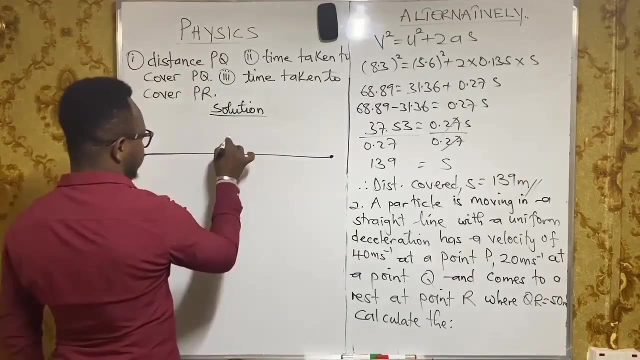 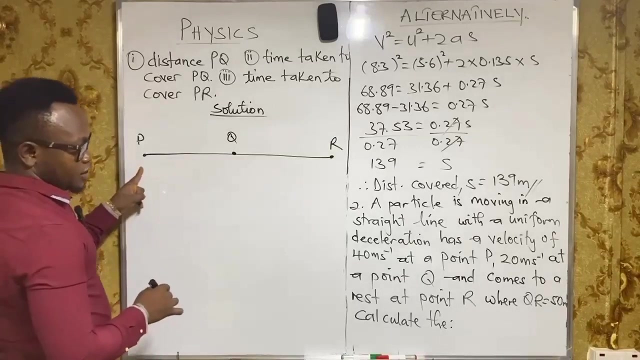 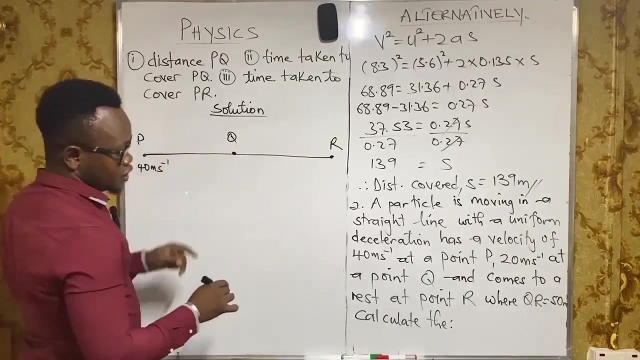 p here. this is point p, and then it is moving in a straight line onto a point where it comes at rest, at point r. so meaning there are three points: you have point p, you have point q and you have point r. these are points, so the initial velocity at point p here is 40 meters per second. 40 meters per second. and at point q 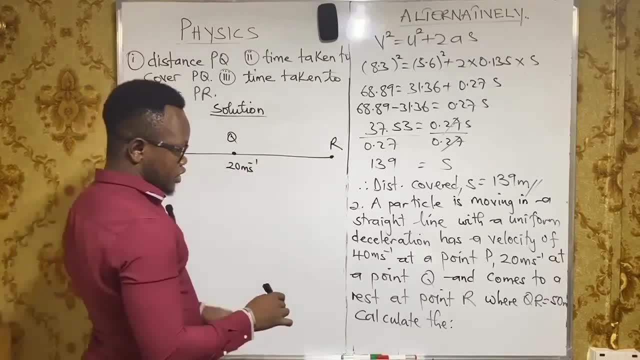 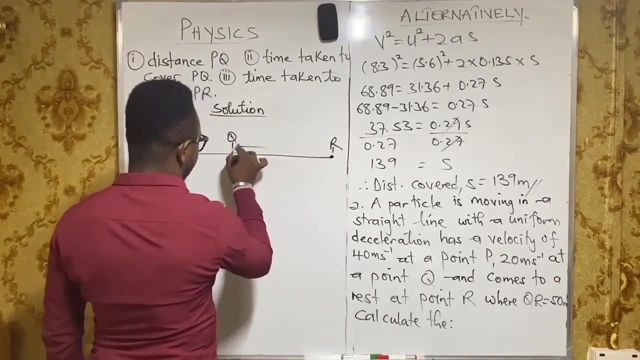 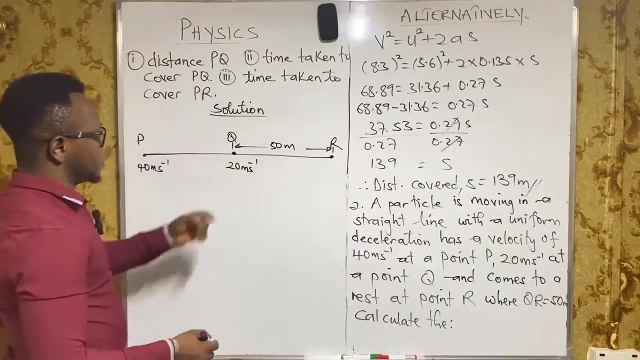 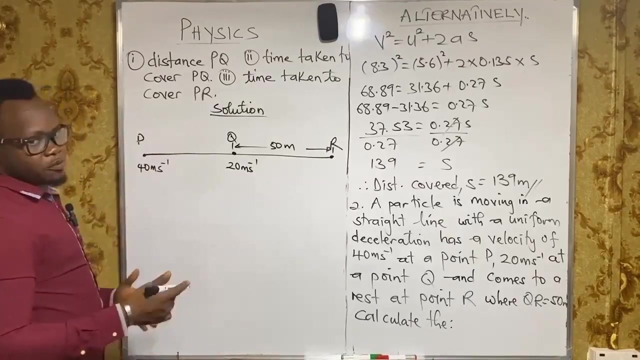 is 20 meters per second. and then, at r, it came to rest and we are told that the distance between q and r is 50 meters. we have to calculate the distance pq. but before calculating distance pq, we first of all need to know the rate at which this particle was decelerating. 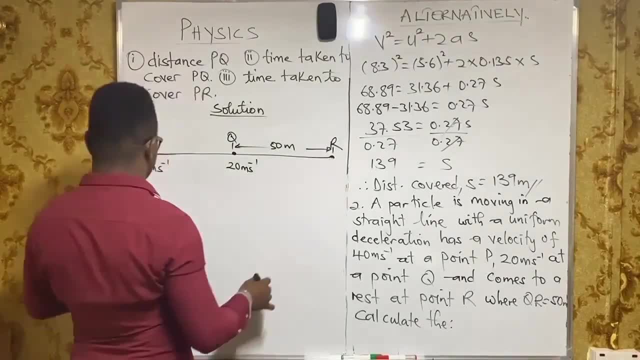 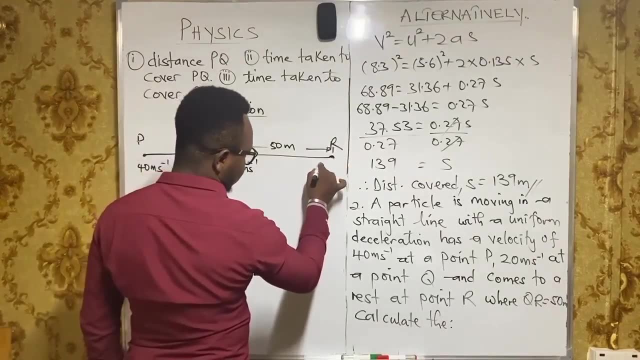 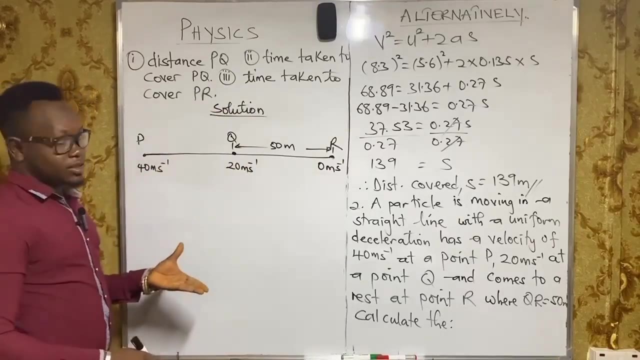 okay in solving this now. it started here 40 meters per second and decelerated to 20 meters per second and where it came at rest, the velocity there is zero meters per second. so from point p to point q, we don't know the distance, so we are going to start off with qr. so 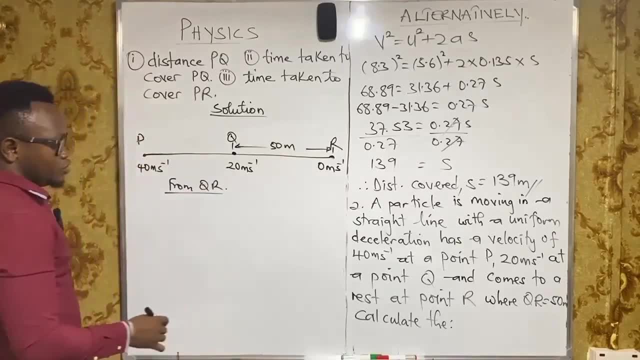 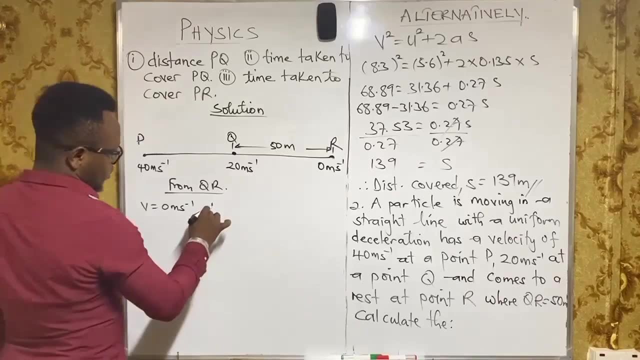 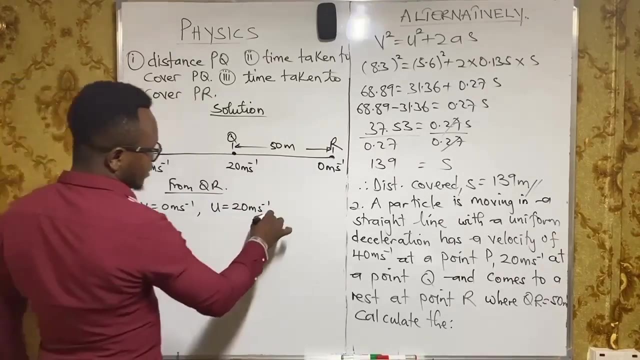 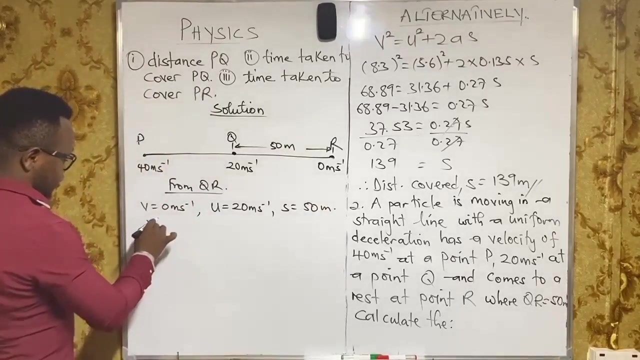 from qr here. that's what we are going to use. we know the final velocity is zero meters per second. the initial velocity u is 20 meters per second, and then the distance covered s is 50 kilometers. so, using the third equation of motion, which says v squared is equal to u squared, 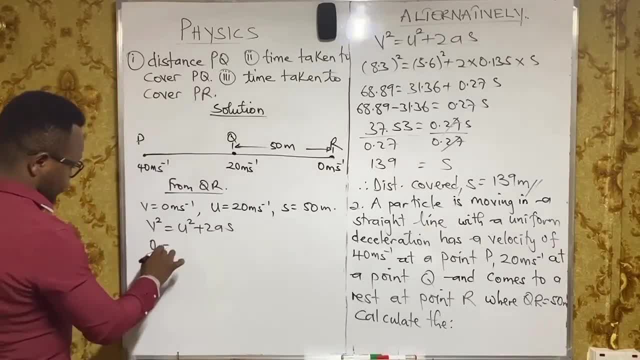 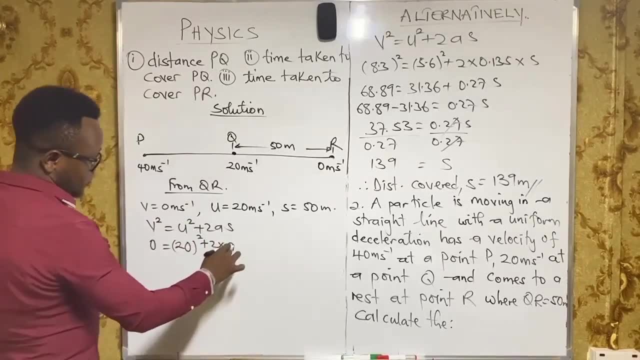 plus 2. s v is 0 is equal to. u is 20 squared plus 2, multiplied by acceleration- we don't know- multiplied by 50.. so 0 is equal to 20 squared will give us 400 plus and this will give us 100 acceleration. so 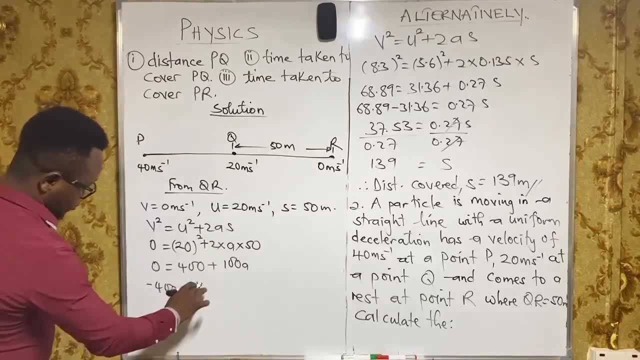 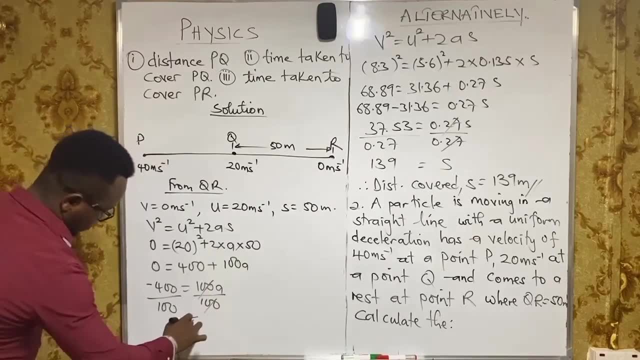 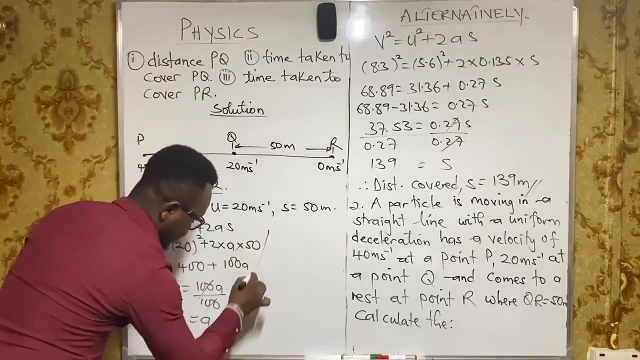 if we transpose this, we get negative. 2 minus 400 is equal to 100 a. so we can divide here by 100, here by 100, this and this will cancel, then a remains. so here we get negative, these zeros, and the zeros will go four. so that tells: 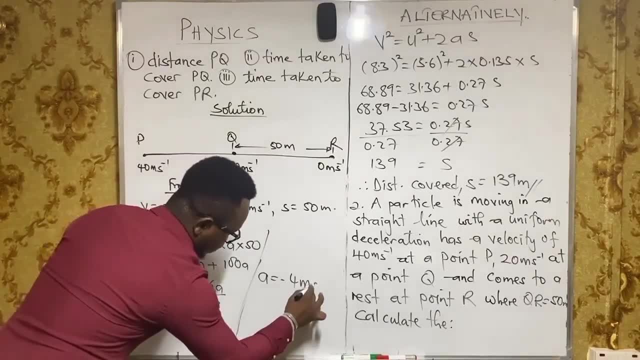 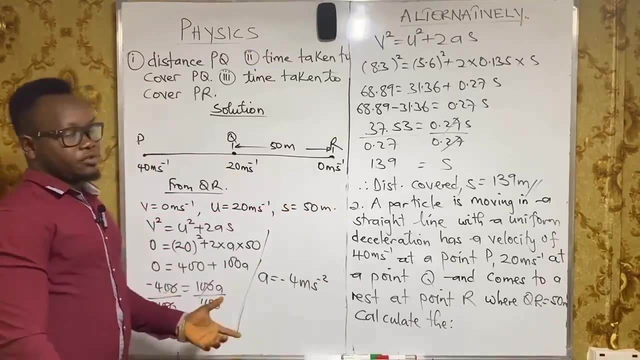 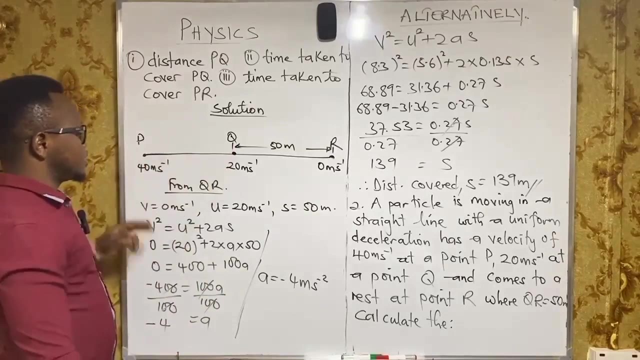 us that the acceleration is negative, four meters per second square. so this is negative because the body is decelerating. i told you earlier that deceleration is the negative to acceleration. so now we can calculate distance pq, because we now know the deceleration okay and we 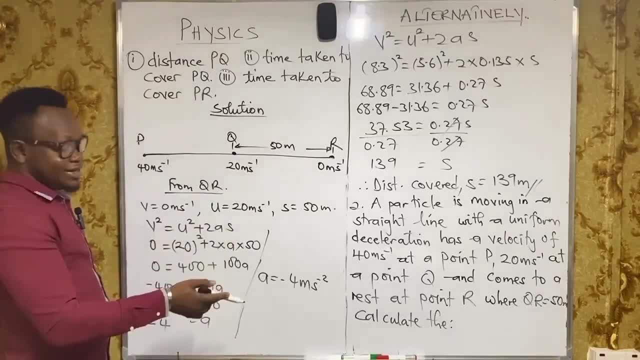 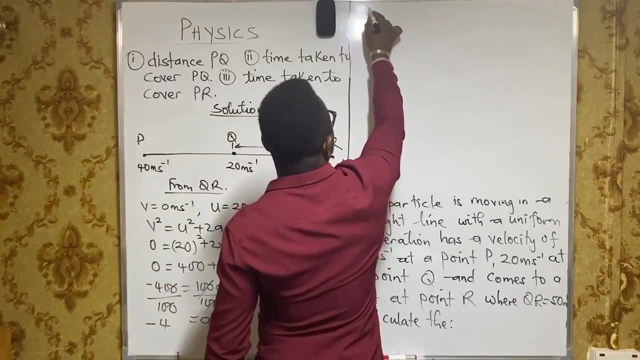 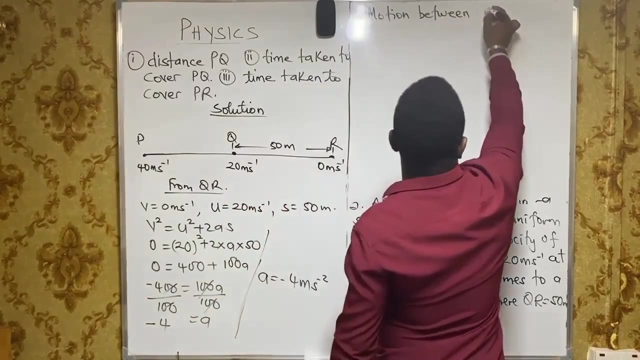 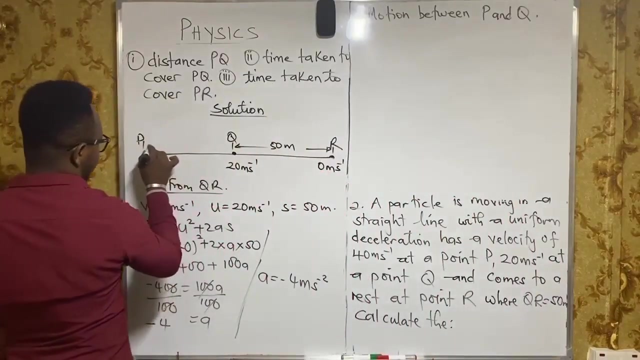 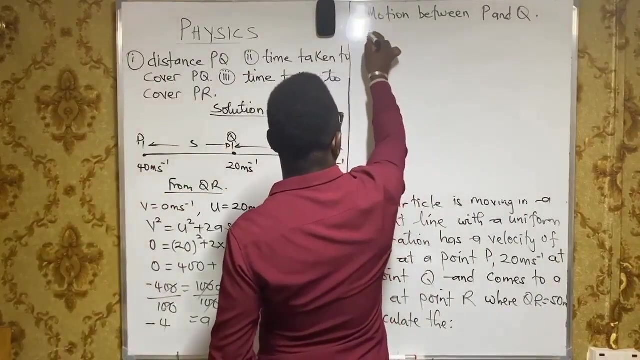 know the initial velocity and the final velocity. so now for the motion. so so now for the motion between p and q here. so this distance here, from this point to this point, i'm going to let it to be s, okay, so the distance is going to be s, which is what. 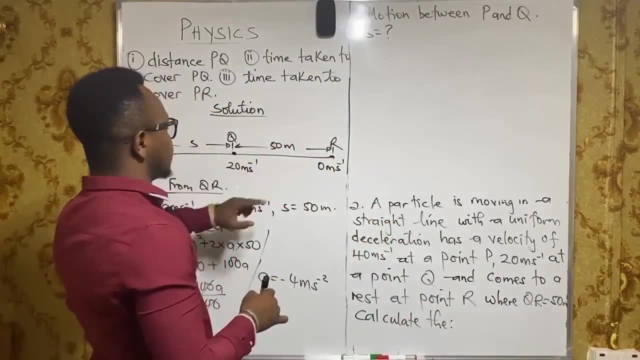 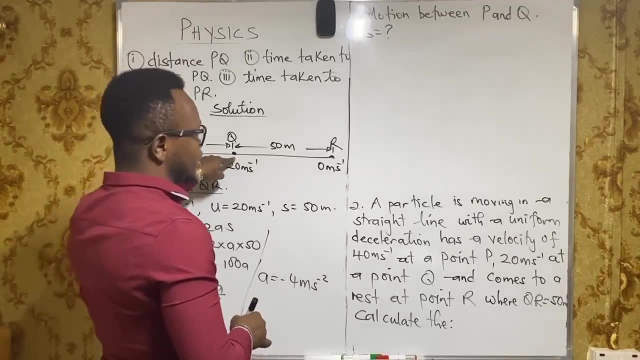 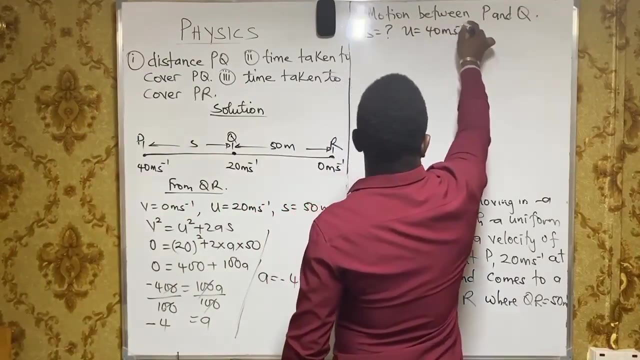 we want to calculate and then, from this point to this point, you have the initial velocity and then you have the final velocity. okay, so this is the final velocity, which is n, which is 20 meters per second. so u is equal to 40 meters per second. v is equal to 20 meters per 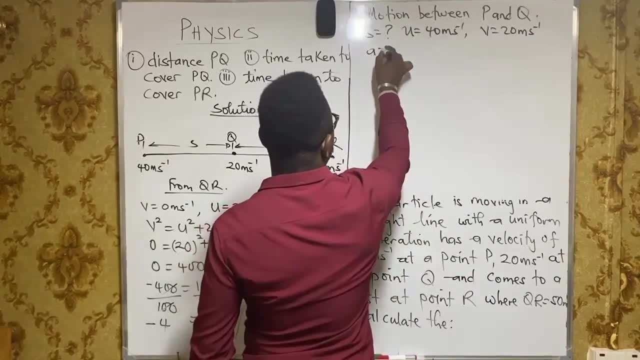 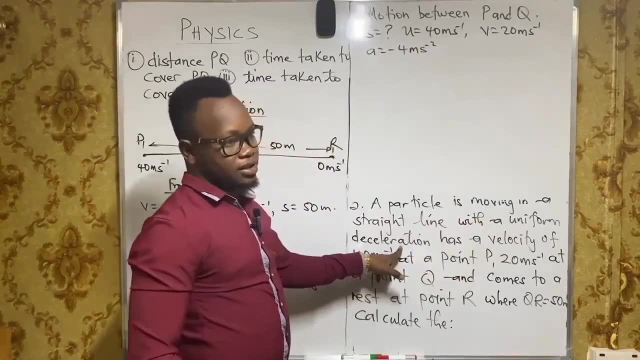 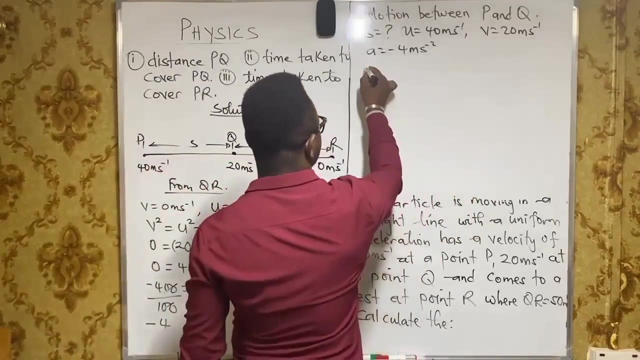 second, and then the acceleration a will now have it to be negative four meters per second because it was moving with a uniform deceleration, so meaning that deceleration is constant throughout the movement of the particle. so using the third equation of motion as v squared is equal to u. 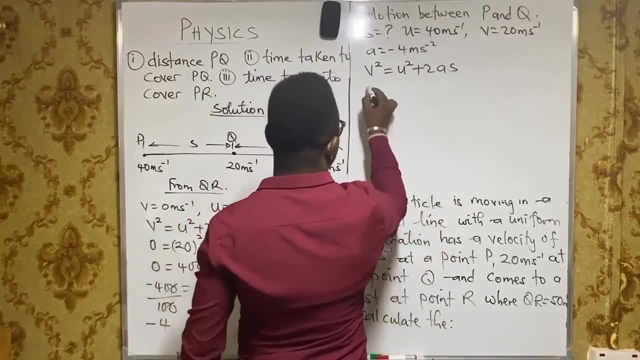 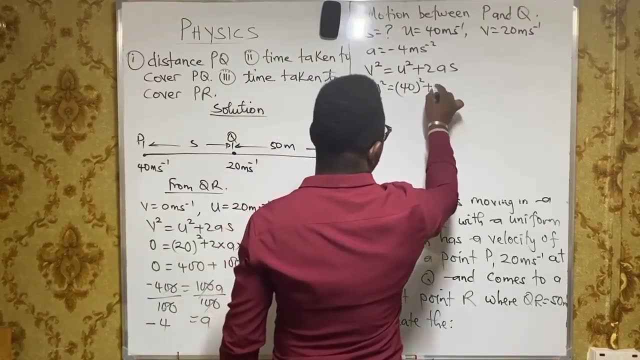 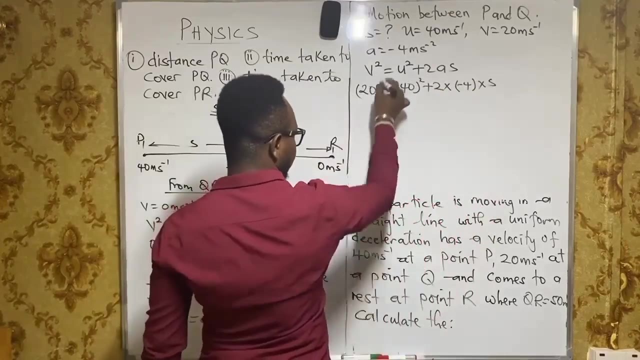 squared plus 2, as so it means v is 20 squared is equal to u is 40. so we say: 40 squared plus 2 multiplied by acceleration is minus 4 multiplied by s. so this here gives us 400 and this gives us so. 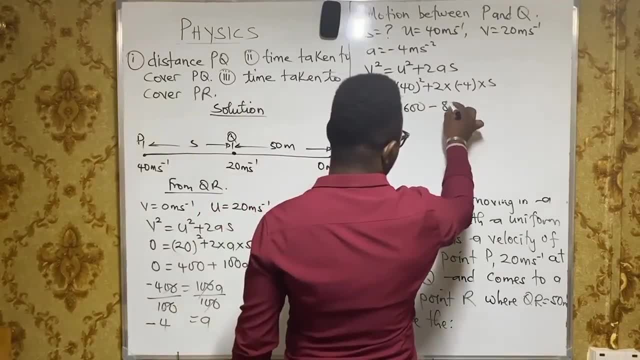 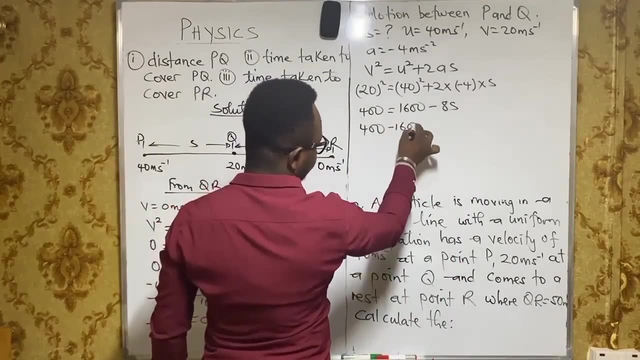 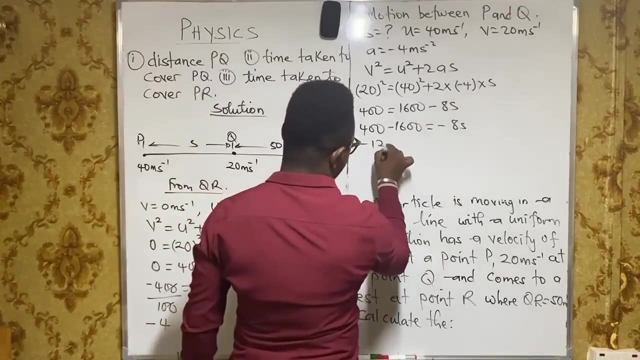 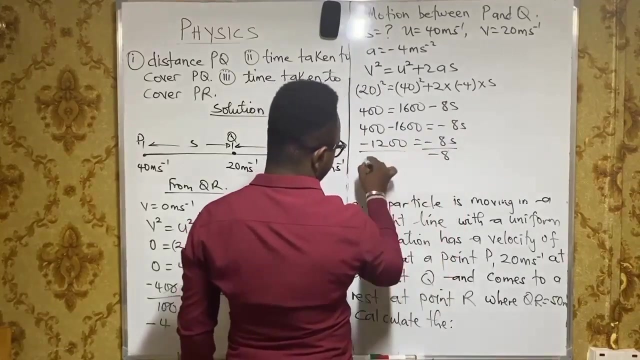 1600 and this gives us negative 8s. so what we do? we can transpose this 400. if this becomes negative, 1600 is equal to negative 8s. so 400 minus this gives us negative. 1200 is equal to negative this. so we divide here by minus 8, minus 8, this and this cancels. 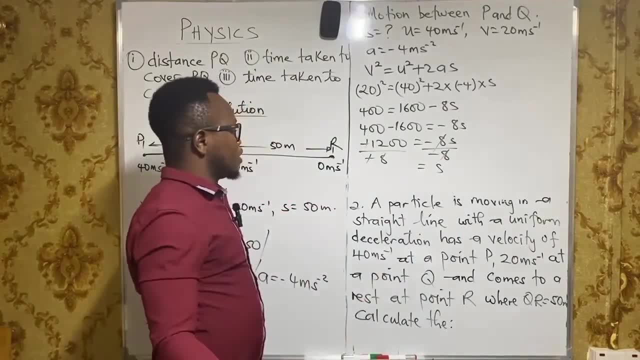 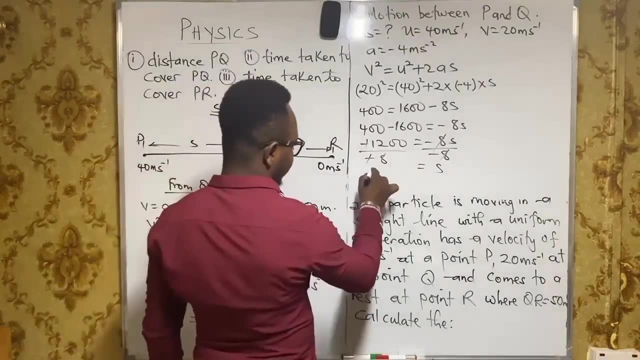 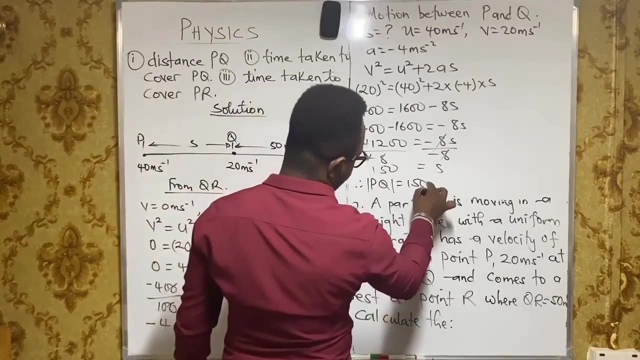 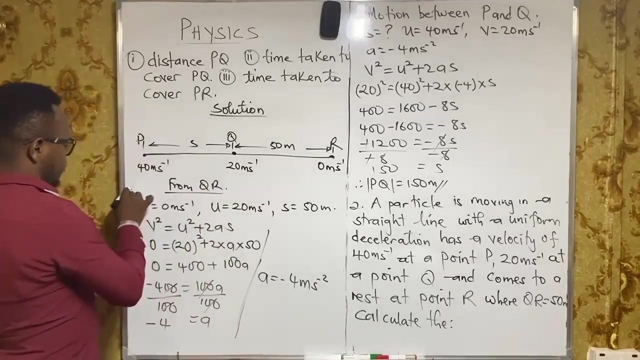 negative sine, 90 negative sine cancels. so 1200 divided by 8, 1200 divided by 8, that gives us 150.. so meaning the distance pq is equal to 150 meters. so that gives us distance pq. that's for roman number one. so we have it to be 150.. so next we are asked to: 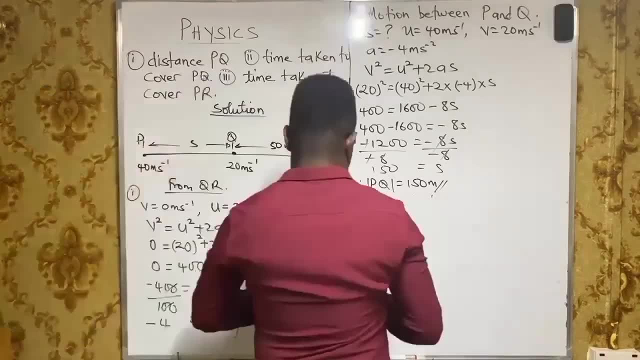 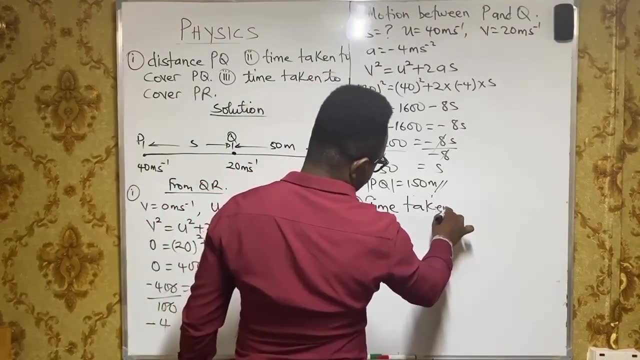 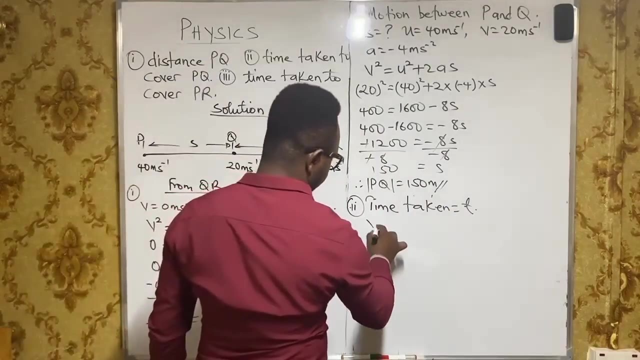 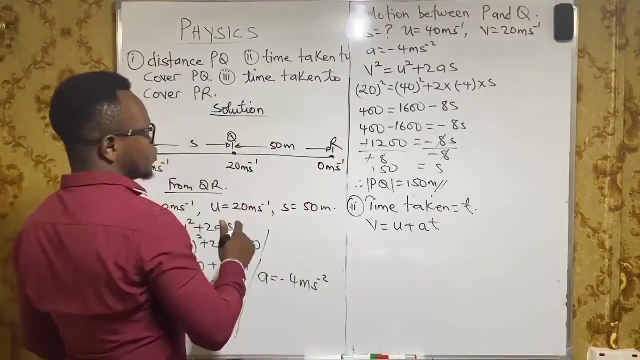 combine r to the xcq and let r and the x pedal. so for this one we need to use the square, because you want to calculate the time taken to cover our distance. this roman figure 2, time taken, that's t. so for us to get time taken we can use the first equation. 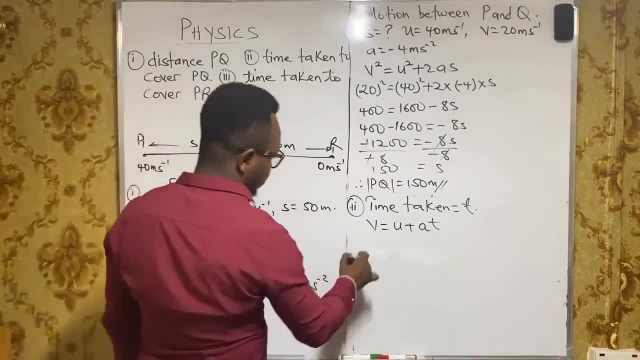 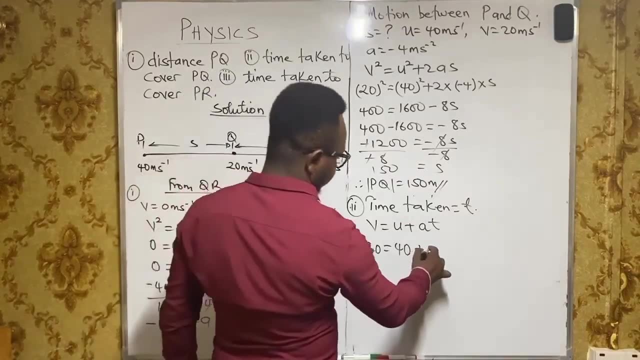 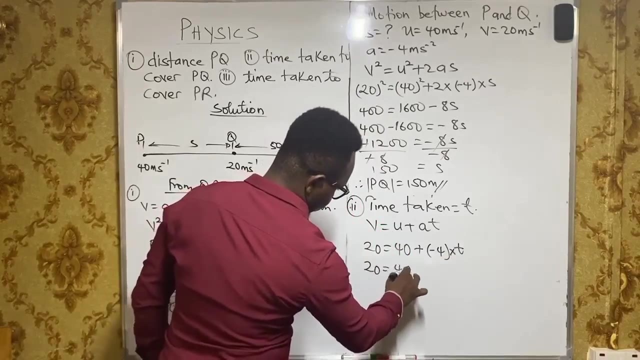 must equal to u plus 80, okay, so so we can say 20 is equal to 40 plus, and if we get the acceleration, and that is going to be negative 4 multiplied by T, so 20 will be equal to 40 minus 40. so if 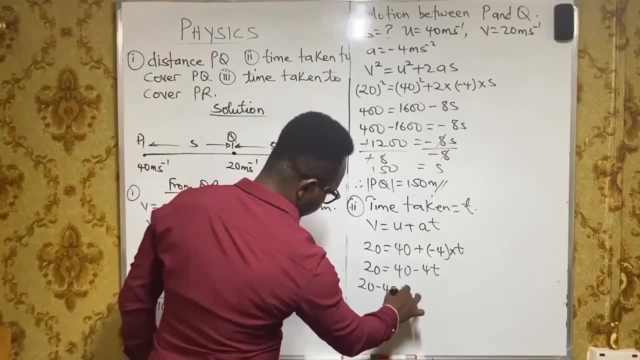 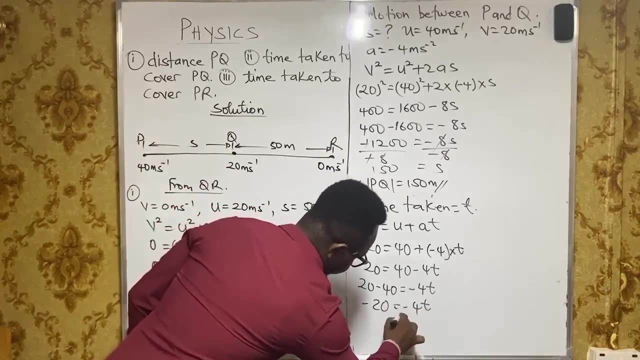 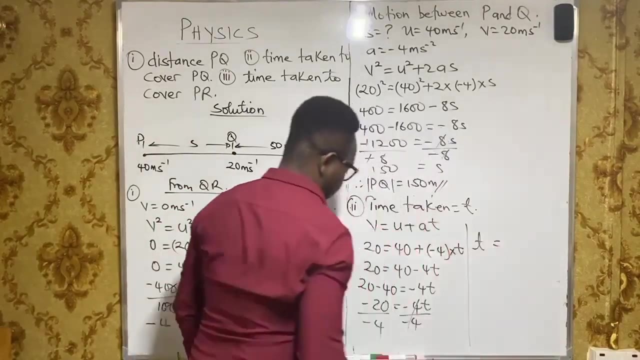 we transpose this, 20 minus 40 will be equal to negative 4 T. so here we get: negative 20 is equal to negative 40. we divide here by negative 4. negative 4 cancels T. remains here this and this goes. so we have the time to be 5. 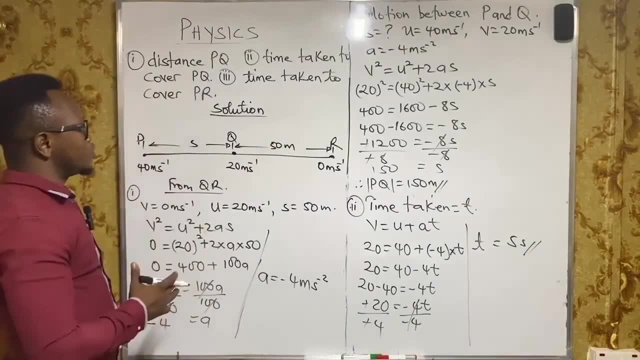 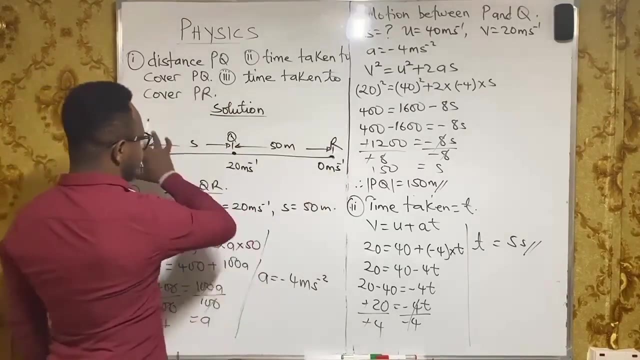 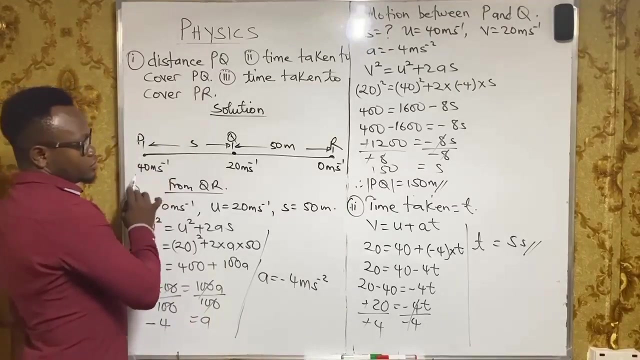 seconds. so meaning it took the particle 5 seconds to cover this distance from point P to point Q. and now the question says the time taken to cover P R, meaning from point P to point R, the whole distance. so in this case this initial velocity is 40, final velocity is 0. okay, that is to cover distance P R. 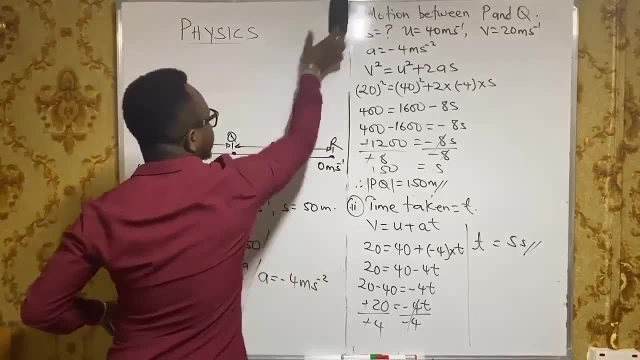 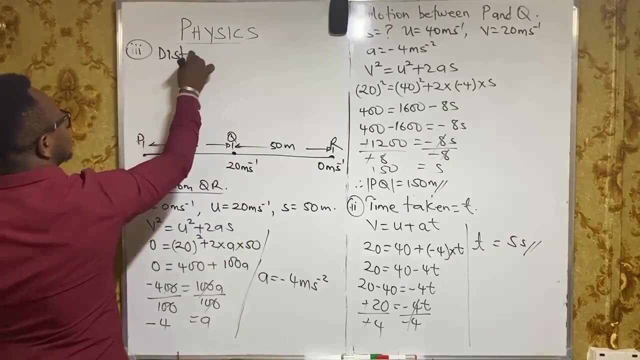 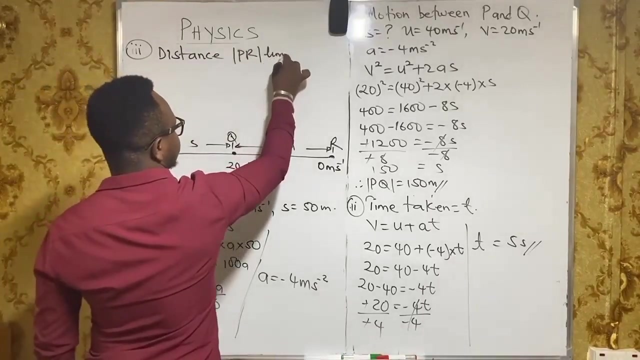 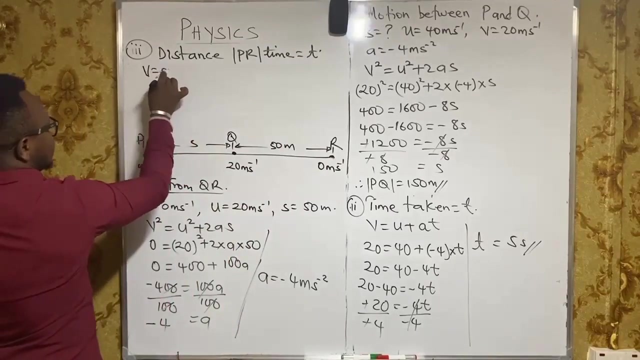 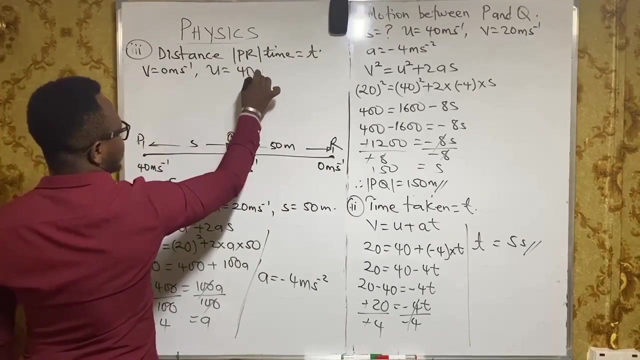 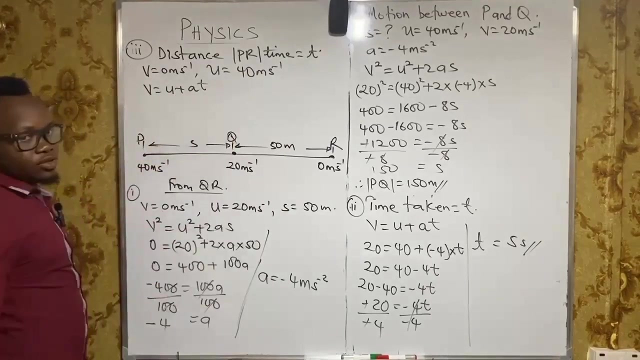 that's the entire motion. so to cover Roman, figure 3 says distance PR time. so in this case the final velocity is 0 meters per second. initial velocity is 40 meters per second. so using V is equal to U plus 80 or if you want, you can use SS equal to UT plus half 80 square, because you know the. 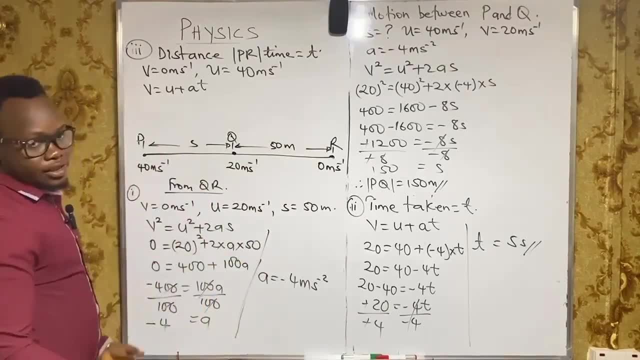 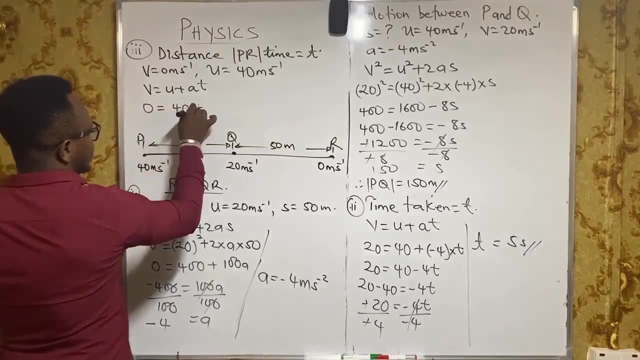 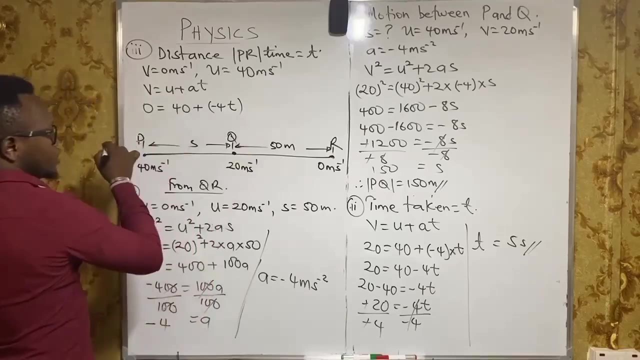 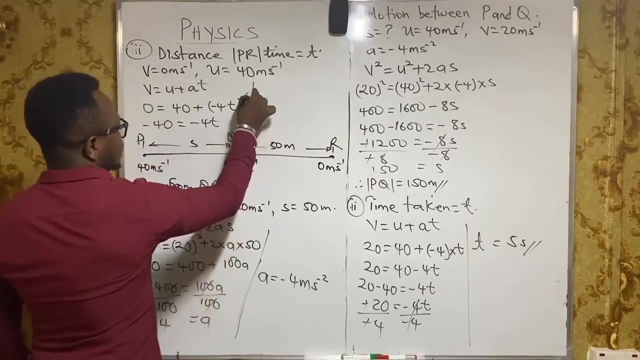 total distance to be 200 meters. you can also use that. you get the same answer. so in this case, here this becomes, 0 is equal to u is 40 plus. and then here we get negative 40. so this situation mean if we transpose this we get negative 40 is equal to minus 40. so negative 40 here minus 40, we divide. 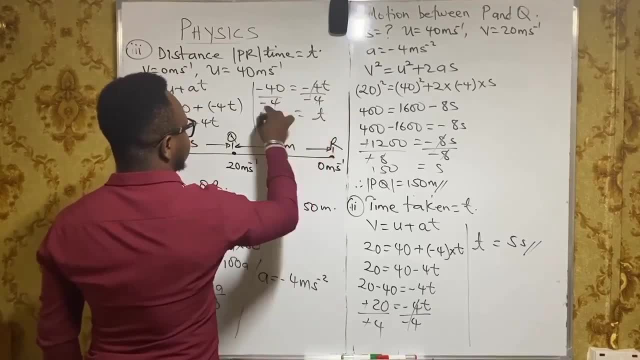 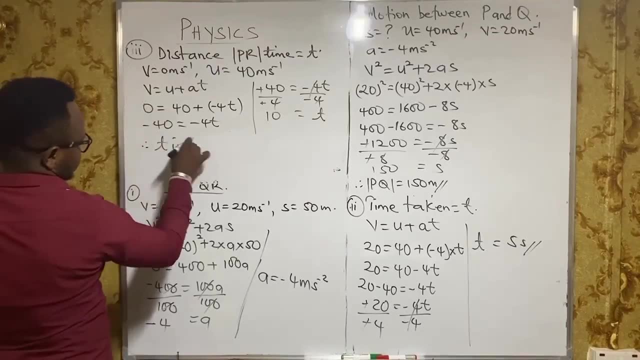 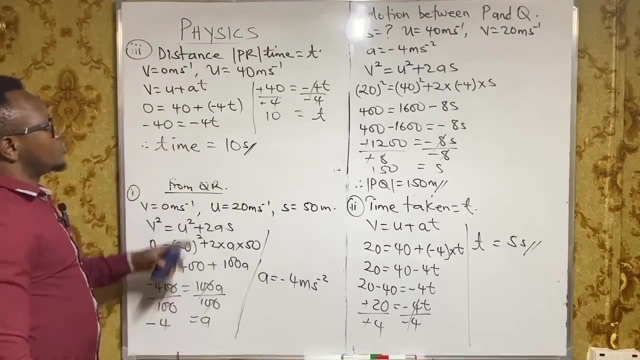 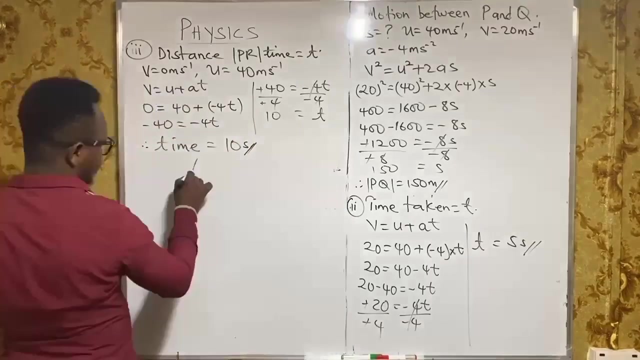 by negative 4, negative 4. so you remain. so this gives us 10. therefore the time is equal to 10 seconds. so this is the time it will take the particle to cover the entire distance, that's when p to point r. you can also use an alternative method. you say alternatively: 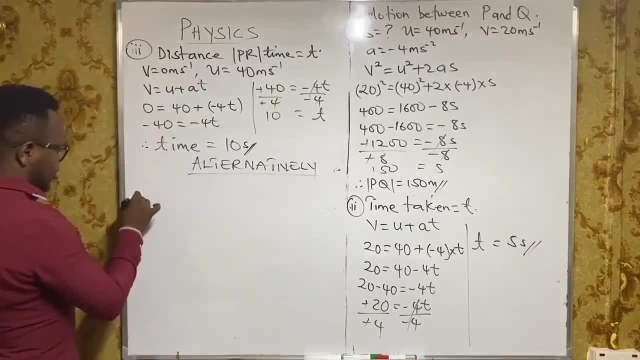 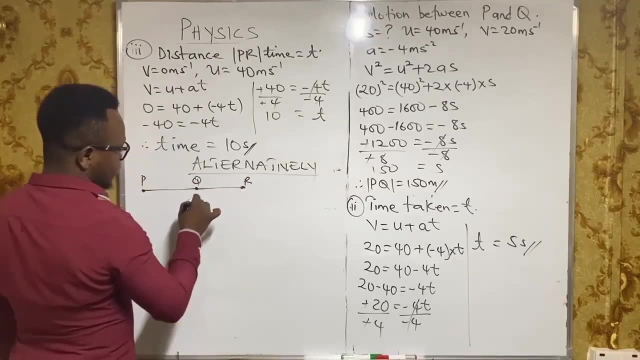 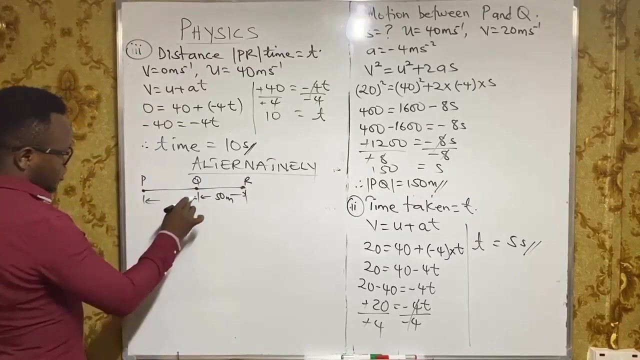 you want to calculate the time, but you know that the journey started from point p and you headed to point q and then to point r. this distance we are given to be 50 and these are the distance we calculated it. we have it to be 150 here. the initial velocity is: 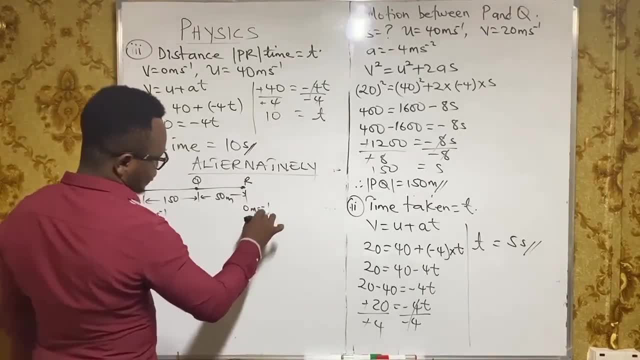 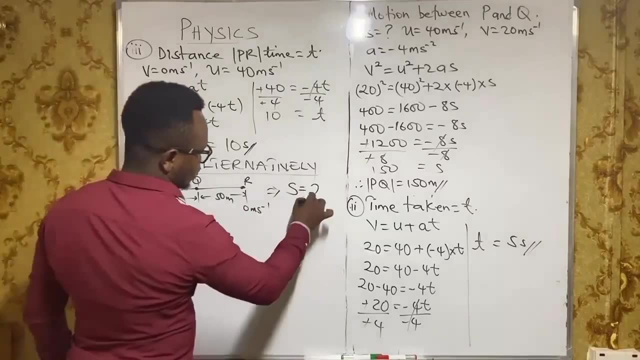 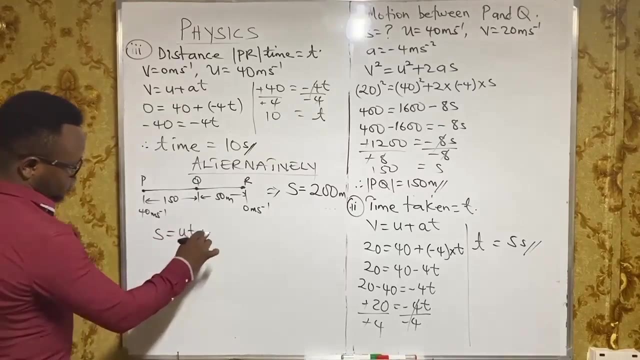 40 meters per second and the final velocity is 0 meters per second. so meaning so this implies: total distance is 0 meters per second and the final velocity is 0 meters per second. s will be 150 plus 50, which will give us 200 meters. so using s is equal to ut plus half 80. 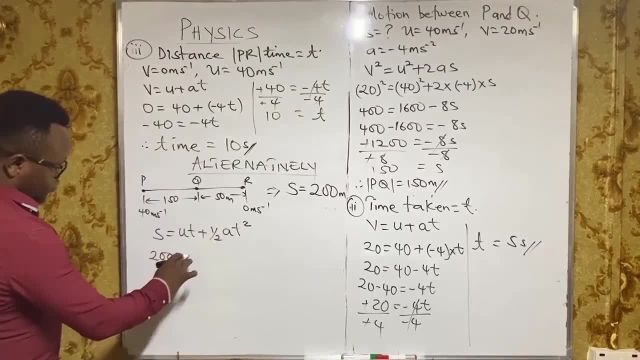 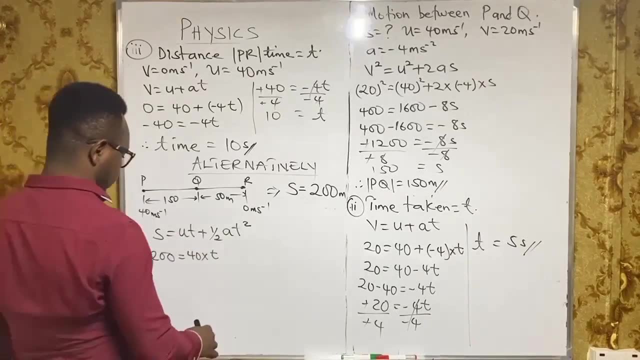 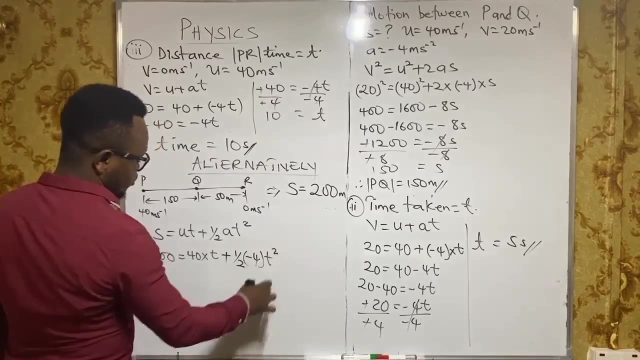 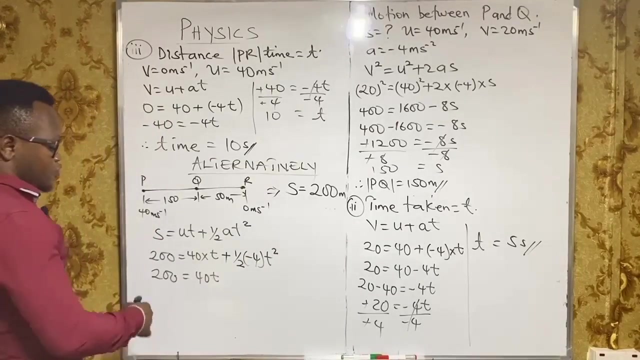 squared s is 200. we equate it to initial velocity. is 40 multiplied by the time, don't know- t plus. so this is half into negative 4 t squared. so 200 is equal to 40 multiplied by t. is 40 t minus plus times minus gives us. 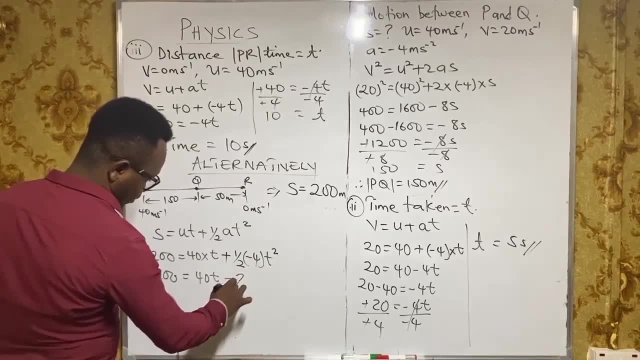 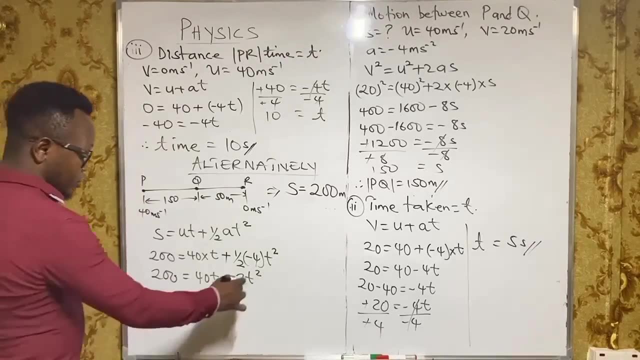 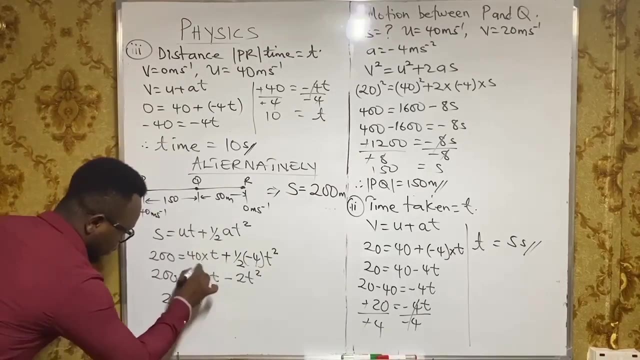 minus, and then 4 divided by 2, we get 2 t squared. so looking at this, you know you are going to arrive at a quadratic, because you're seeing the highest power, h2. so if we transpose this on this side, we get 2 t squared, and then we get 2 t squared, and then we get 2 t squared. 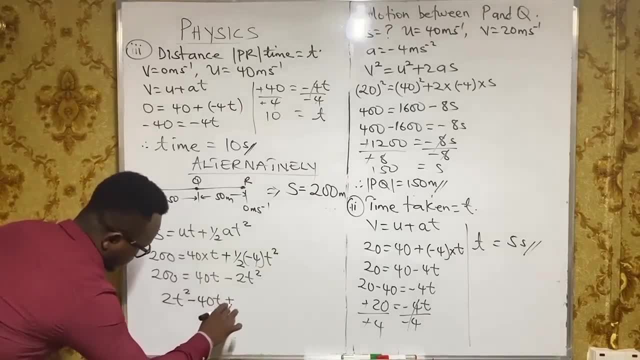 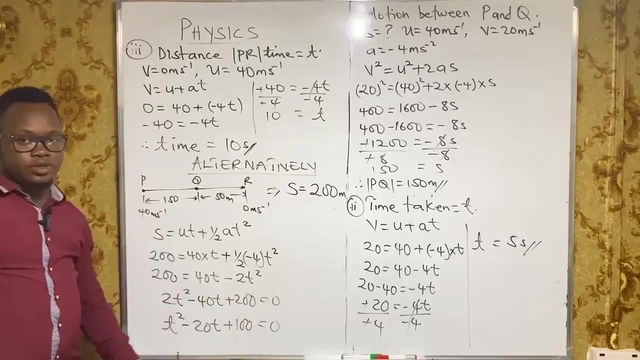 and this followed: we get: minus 40. t plus 200 is equal to 0.. so dividing both sides by 2, we simplify it to be t squared minus 20, t plus 100 is equal to 0.. looking at this here, this one can. 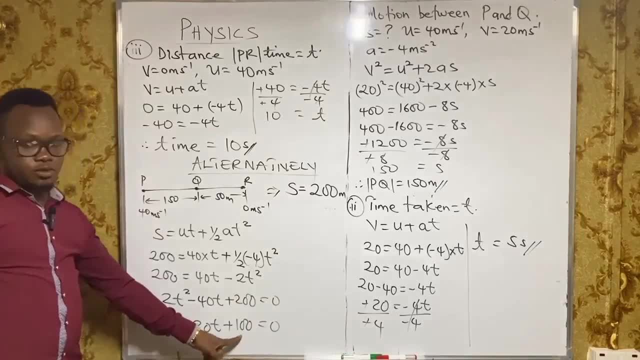 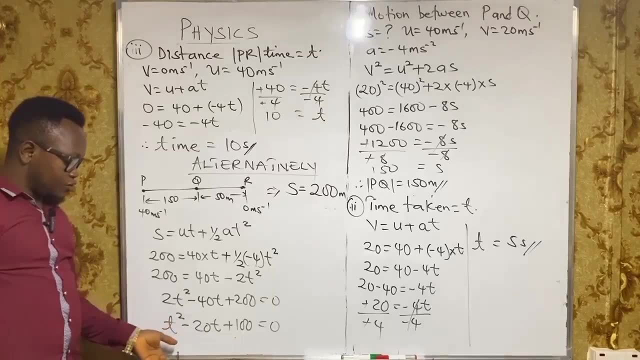 be factorized. because the sum is negative, 20, the product is positive: 100 t squared, so two numbers: if we multiply, we get 100. if we add we get 20.. so we get 100 plus 100 is equal to 0.. so this is. 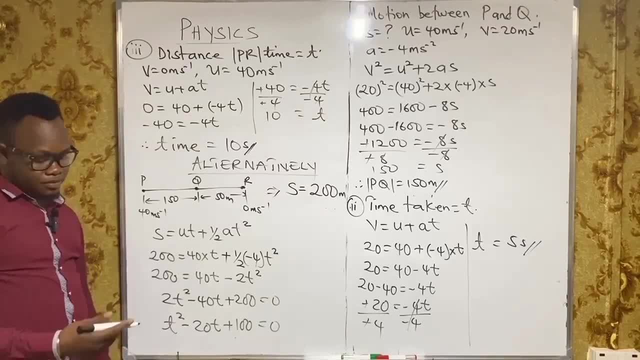 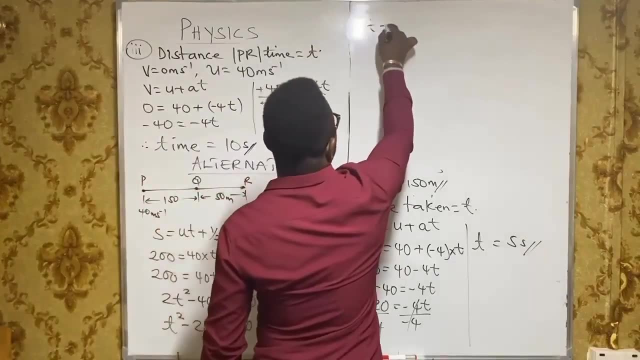 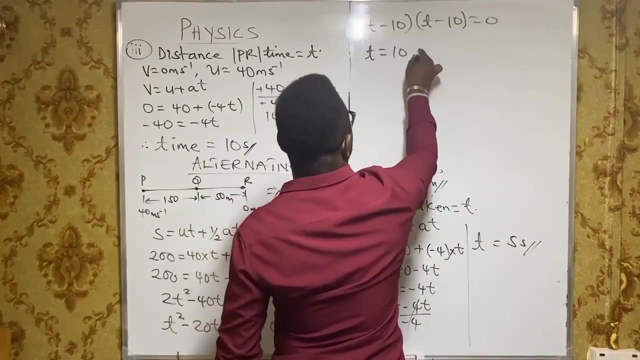 20 will be negative 10 and negative 10.. that's minus 10 and minus 10.. being that the coefficient of t square is unity, so you say t minus 10 in one bracket, and t minus 10 equal to 0, so t is equal to. 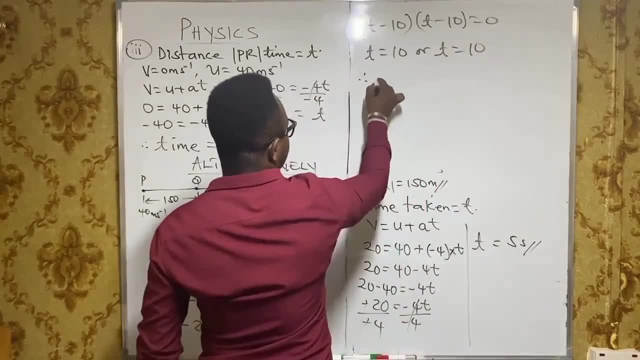 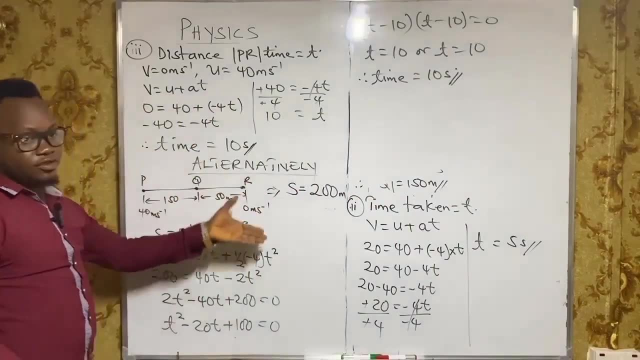 10 or t is equal to 10.. so you get 10.. so that means the time is equal to 10 seconds. so this is an alternative method to solve a problem. so let's go ahead and solve the problem. so we're going to. 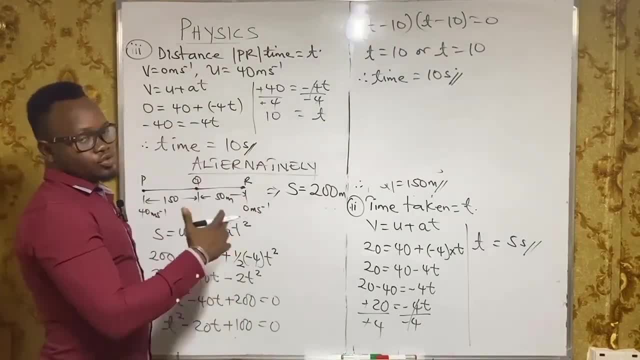 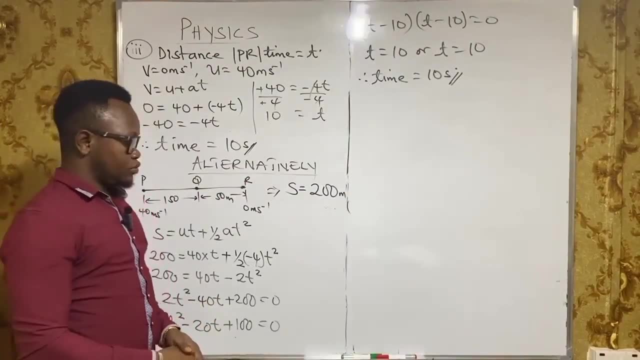 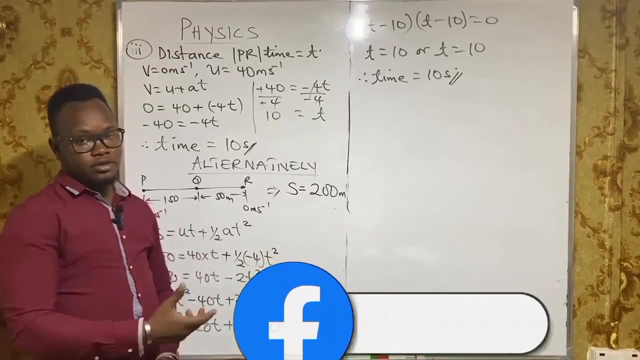 do it. let's go ahead and solve the problem. just cut together like this- I had seen it- so that we didn't have t squared minus 10 squared, so cute. let's do this one. so that goes into this. now I put in the number I'd like to set to our green here, so we've got it again for. 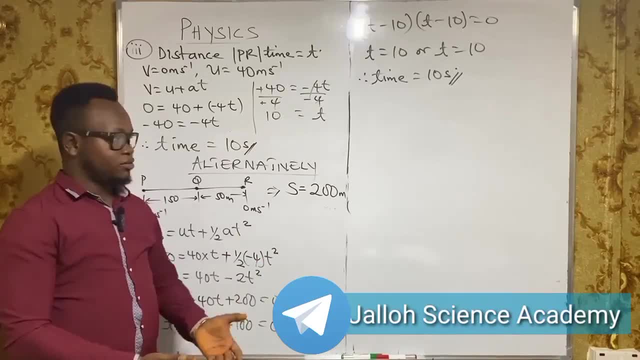 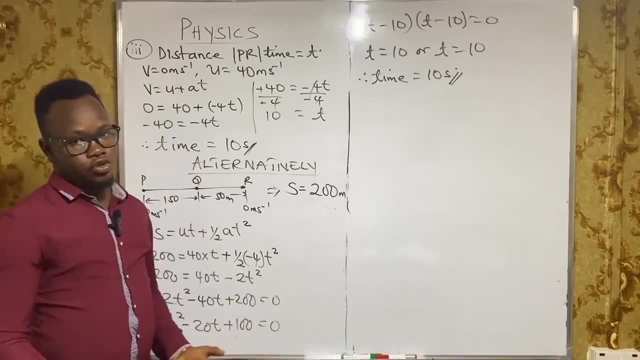 give beautiful colors to ouribe Academy. join the channel, drop your questions. your assignments will help you solve them. thank you very much. love you all. 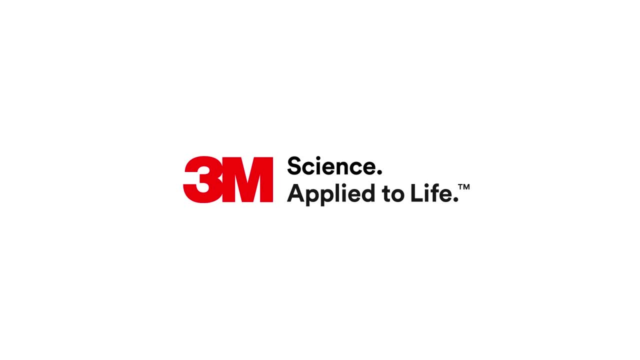 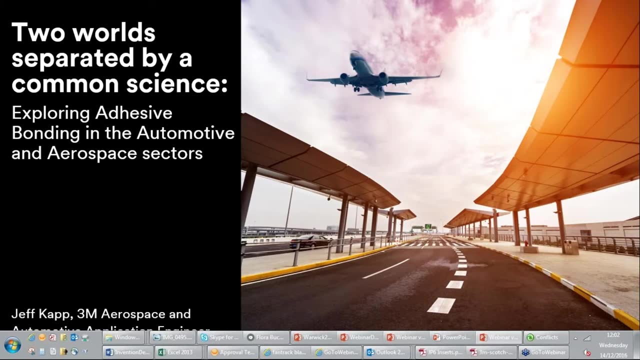 Thank you for joining 3M's webinar. Here we will be exploring adhesive bonding in the automotive and aerospace sectors. Jeff Catt will be speaking to you today. He is an application engineer who specialises in composites, With 16 years of experience in the commercial application. 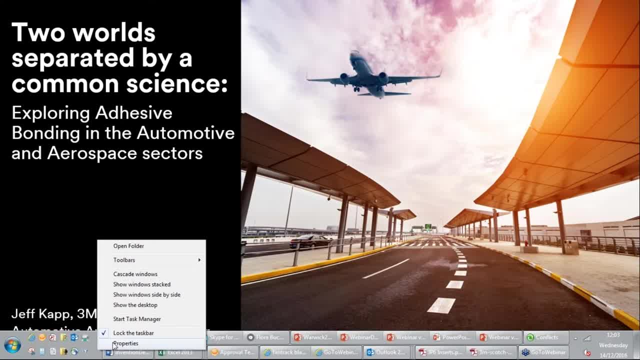 of adhesives. he has worked on a wide range of vehicles, from transit vans through to McLaren and now Aerostructures. Jeff has spent the majority of his time at 3M specialising in automated applications, but has recently moved into our aerospace division applying our